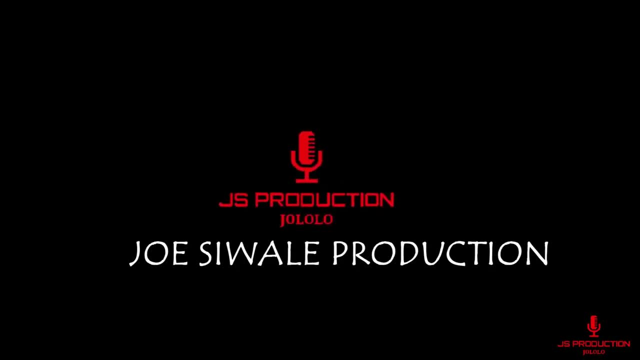 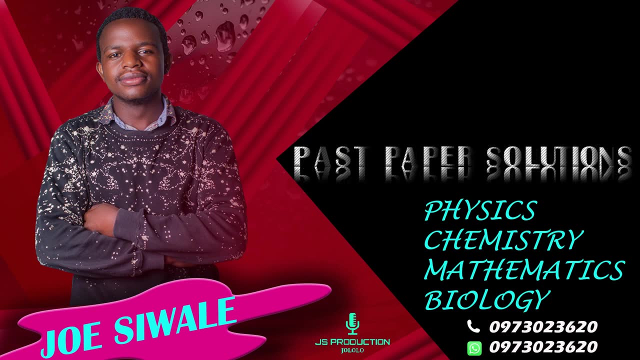 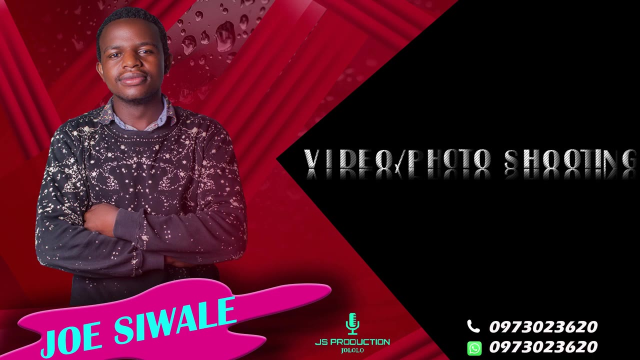 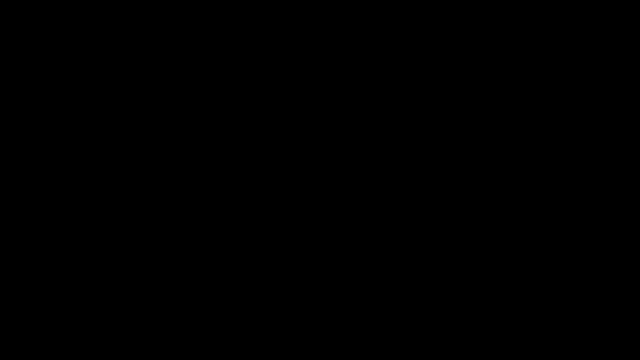 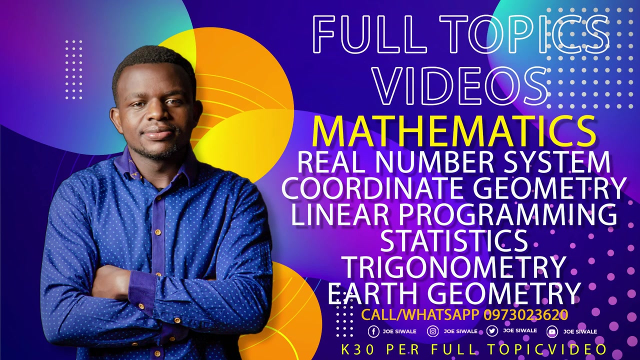 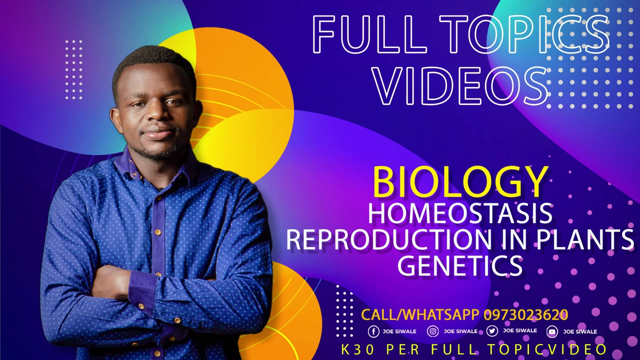 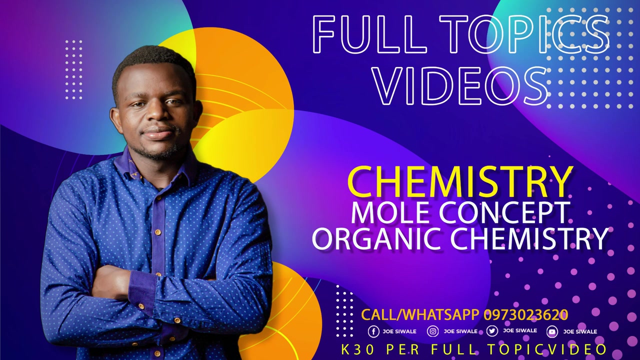 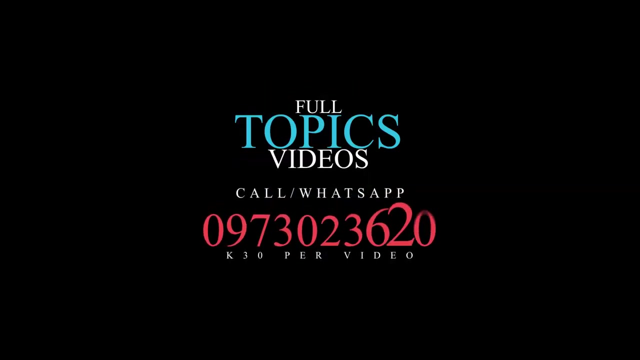 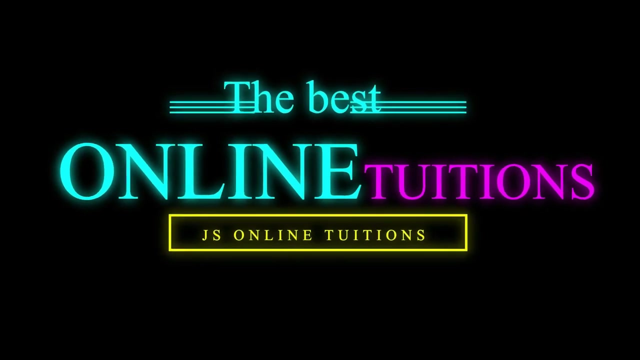 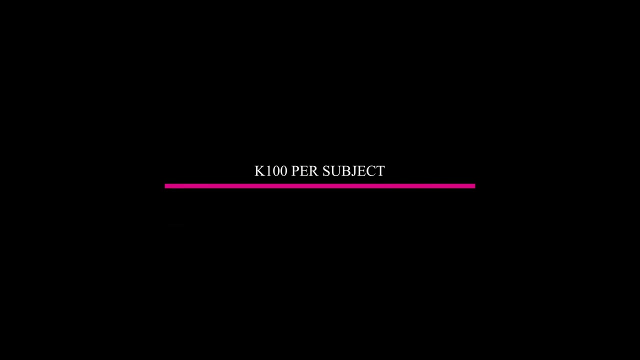 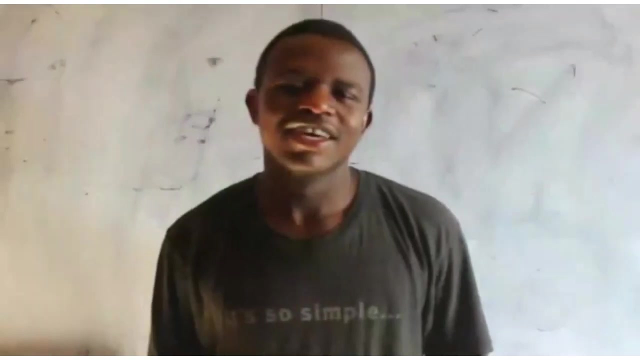 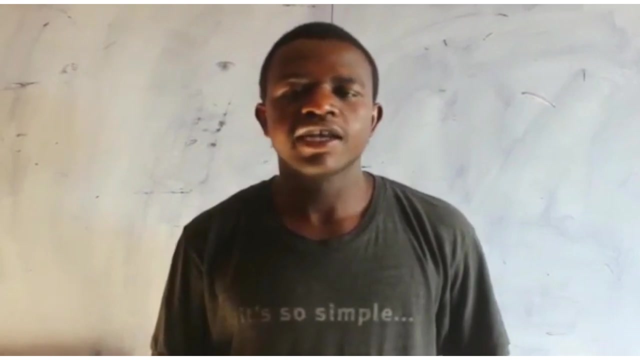 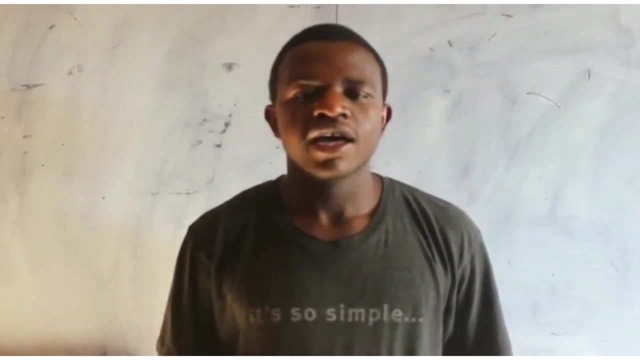 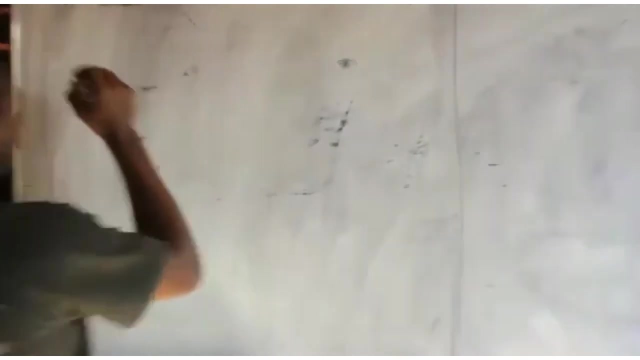 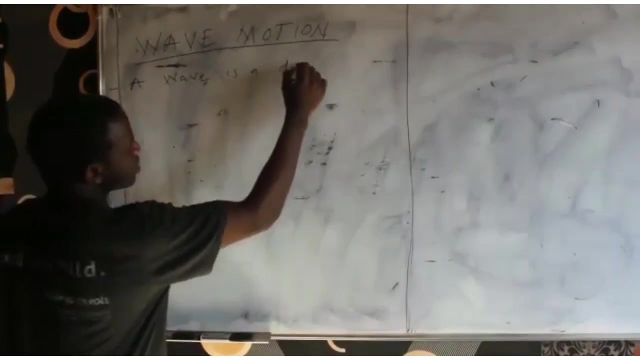 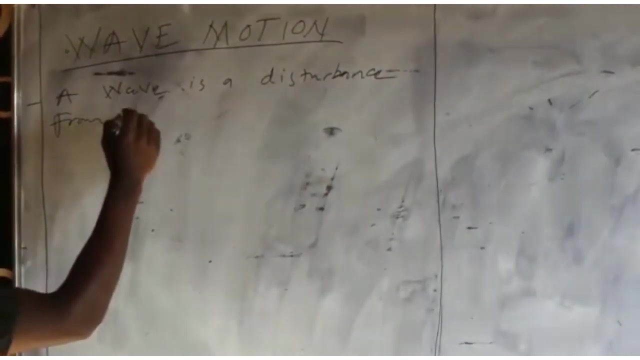 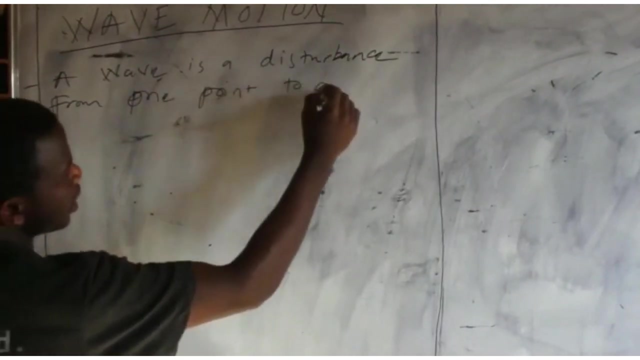 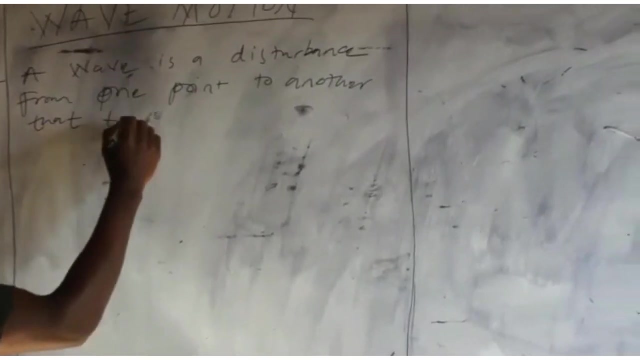 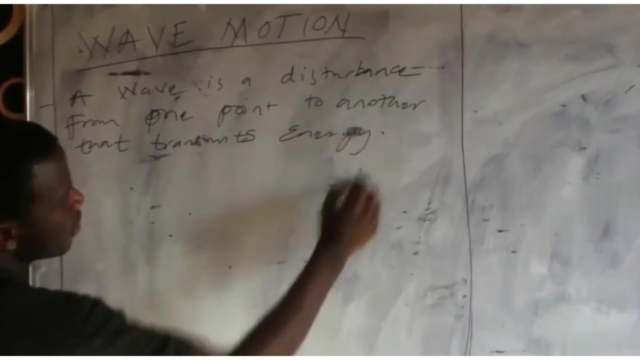 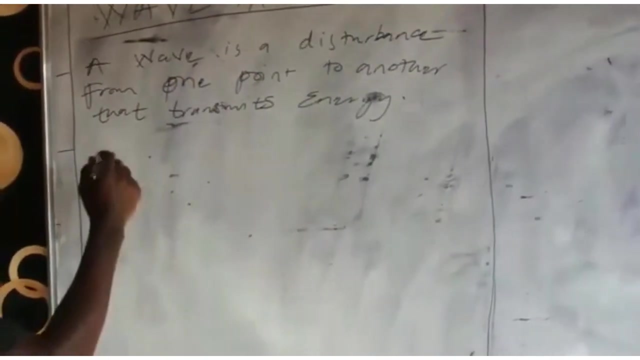 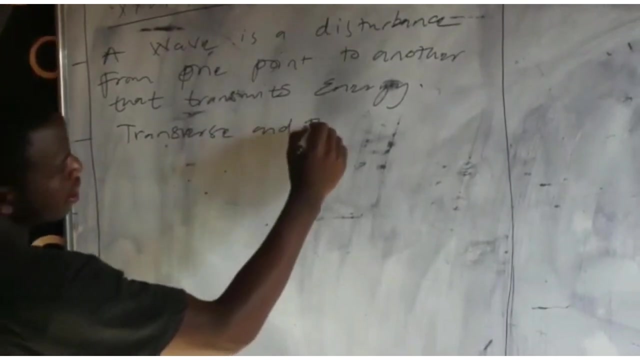 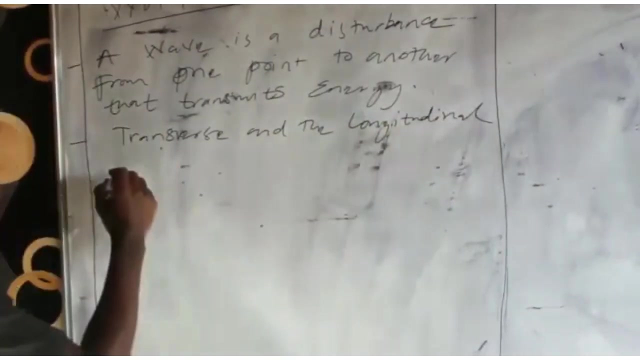 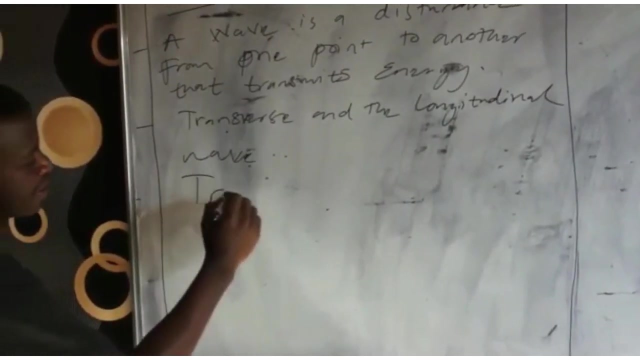 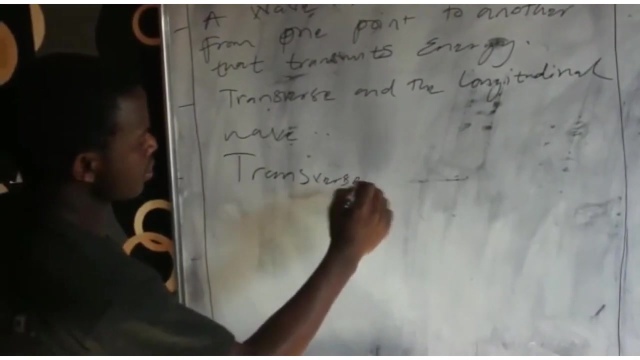 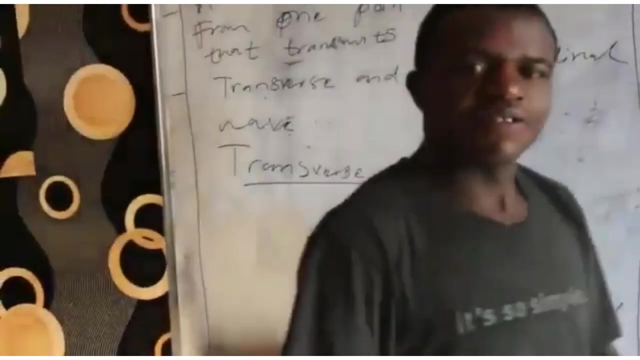 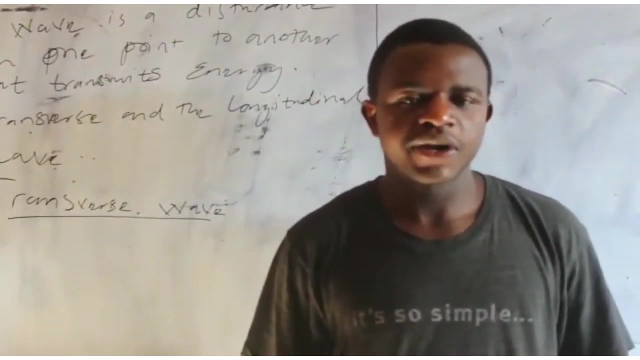 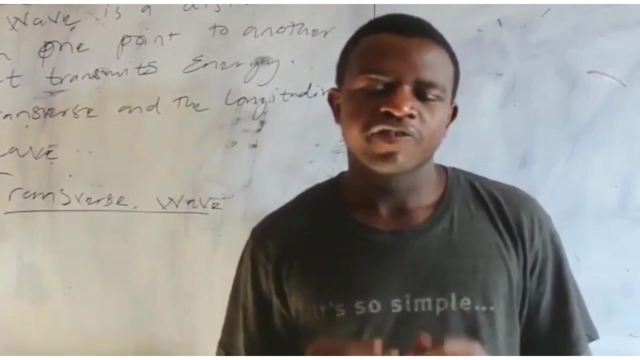 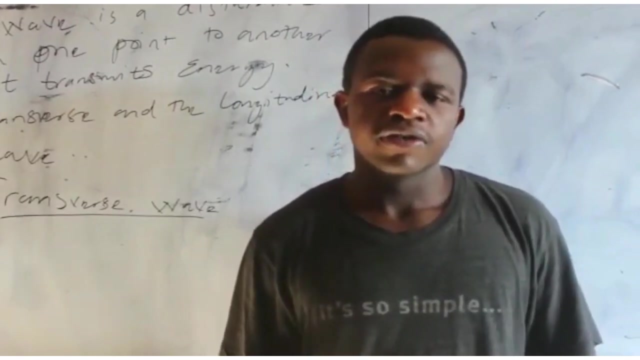 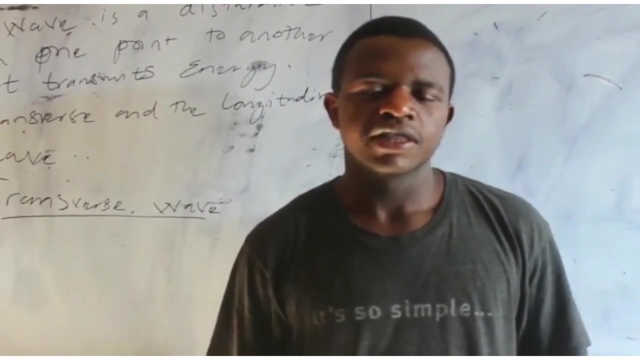 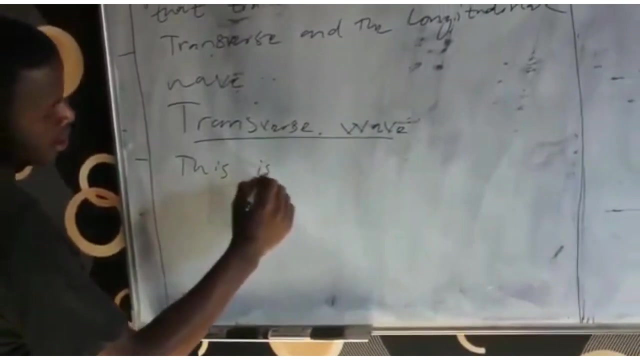 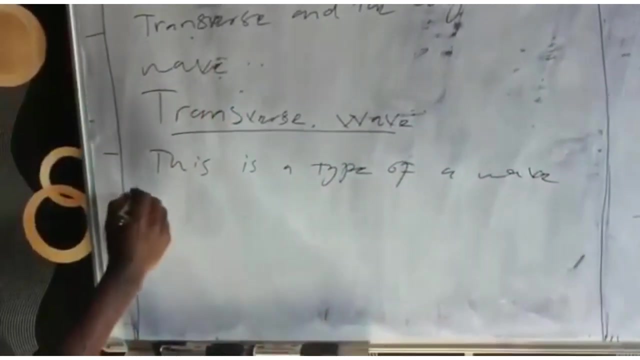 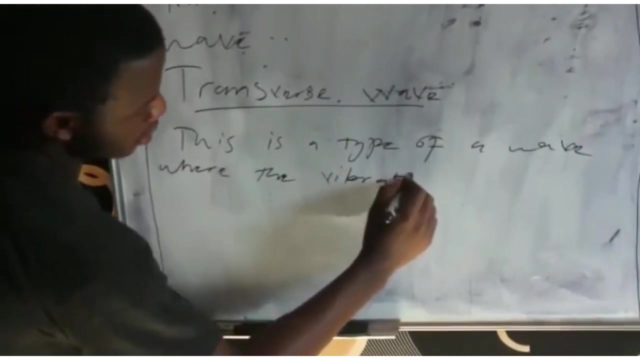 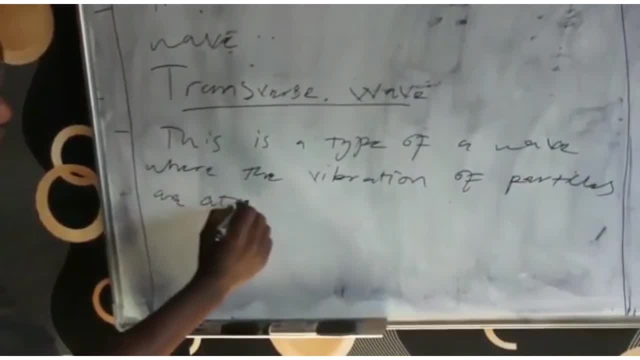 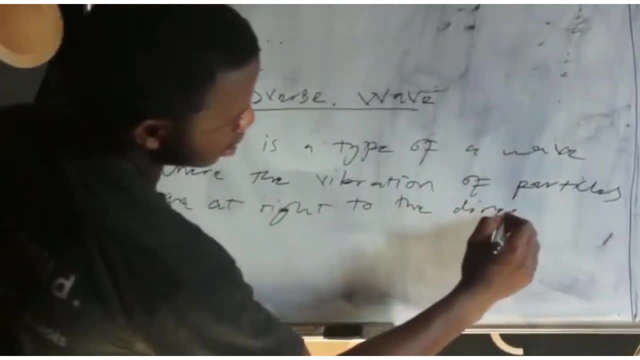 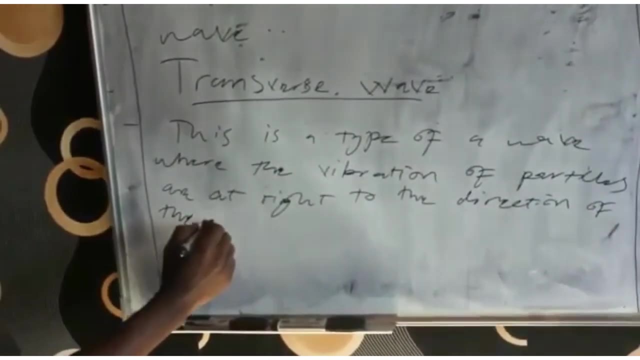 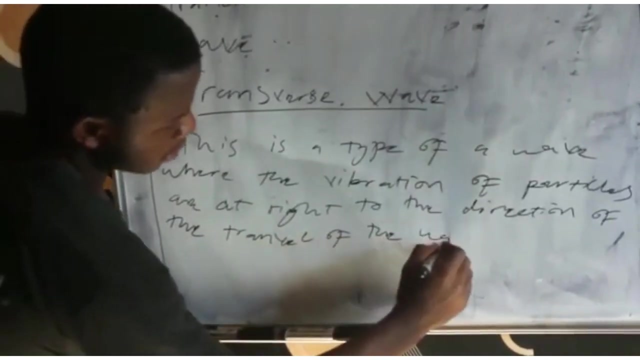 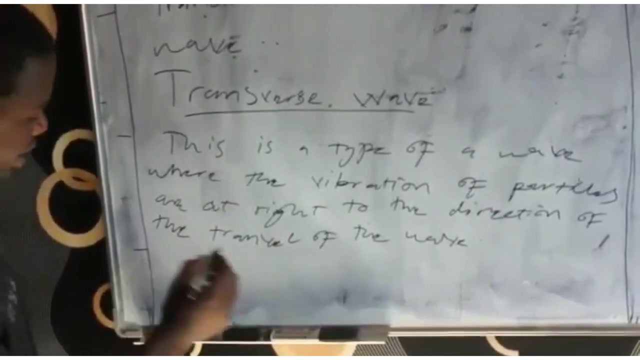 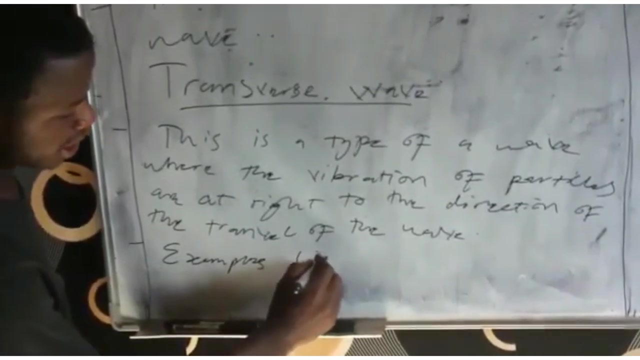 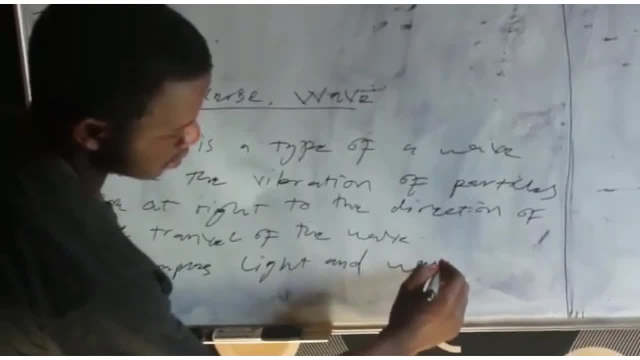 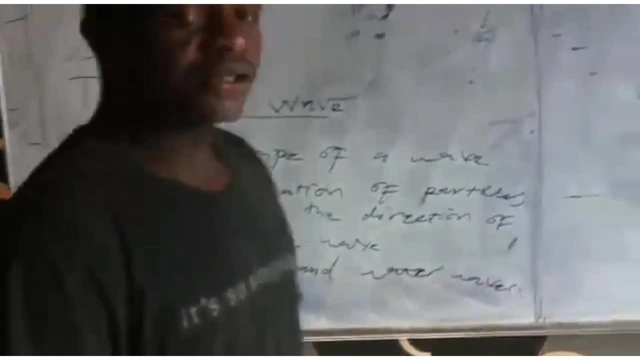 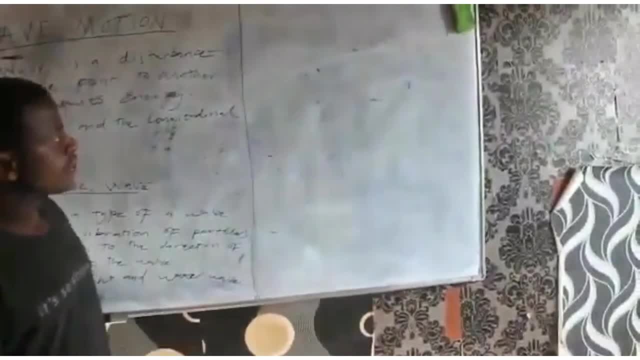 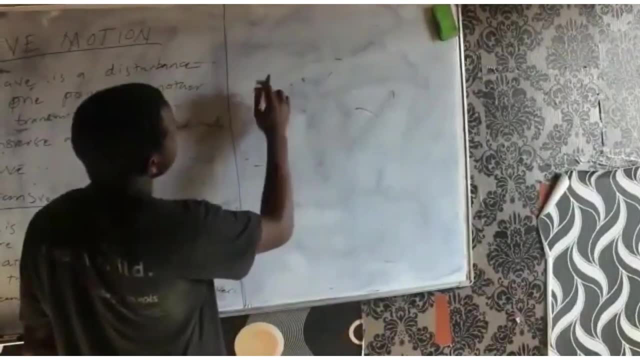 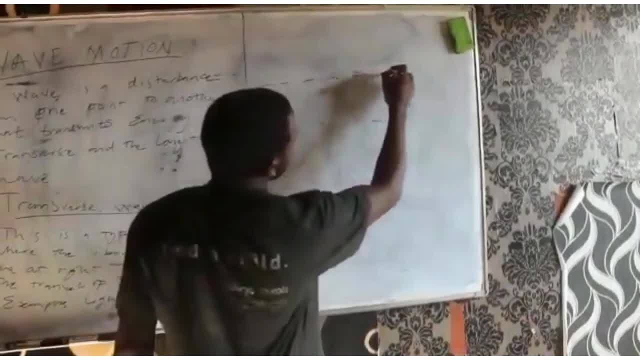 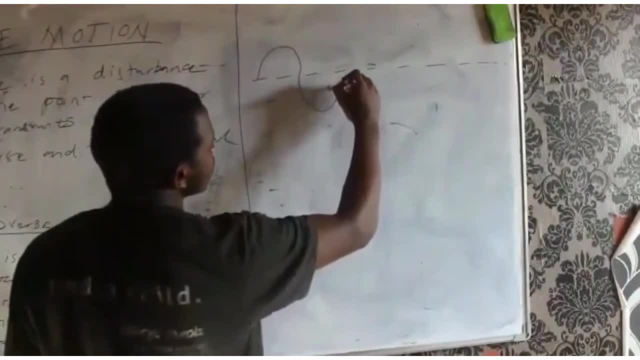 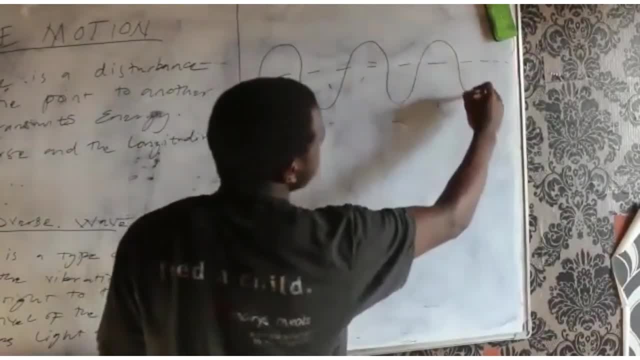 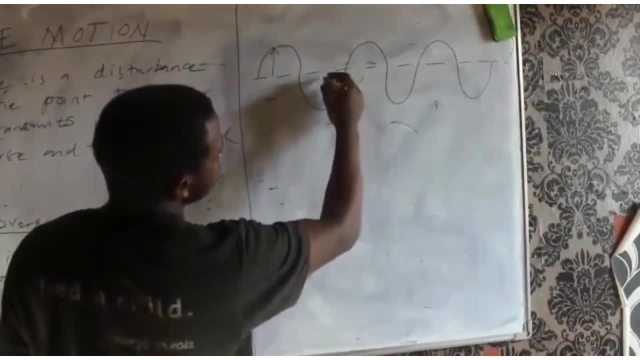 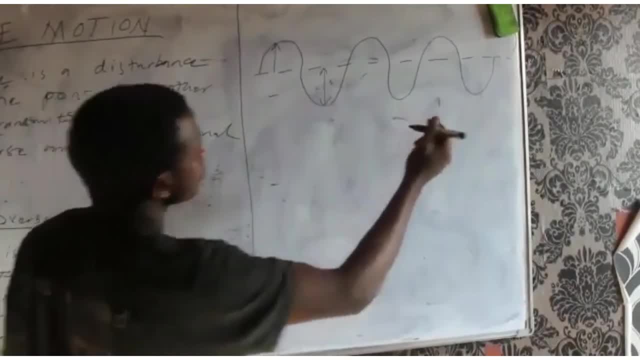 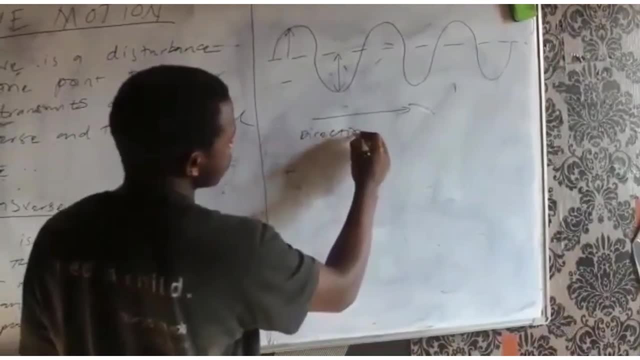 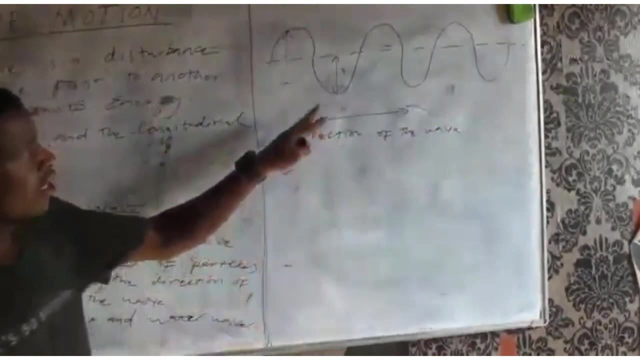 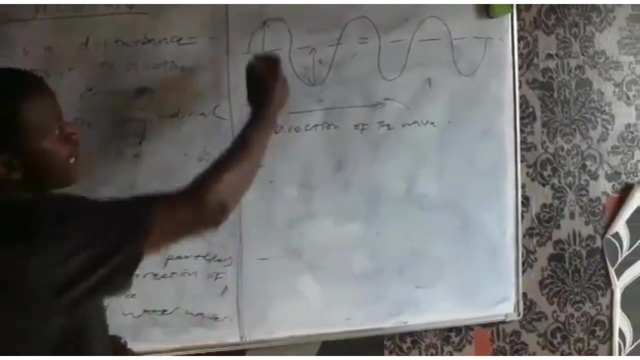 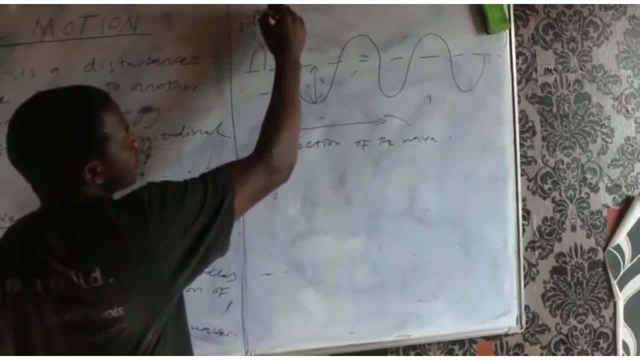 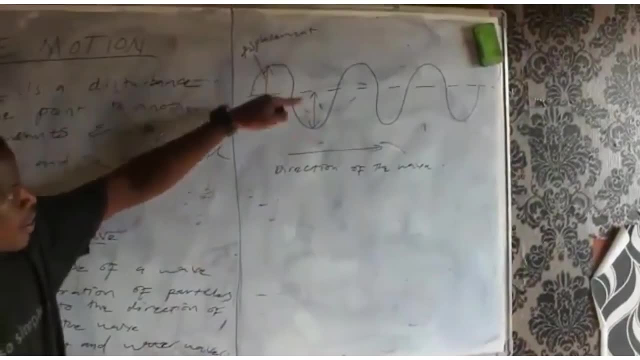 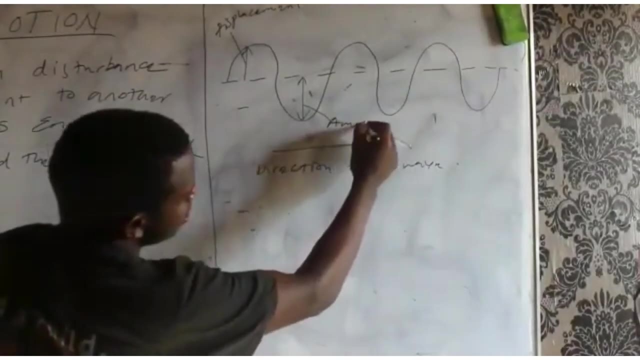 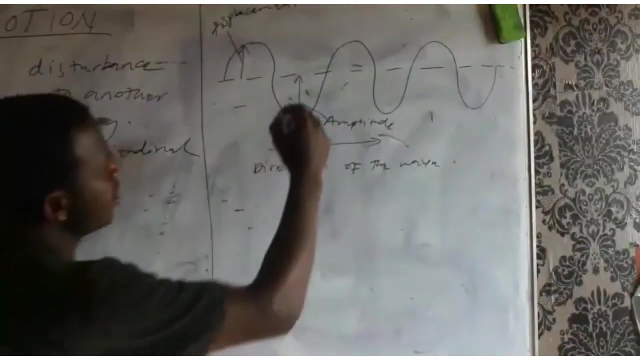 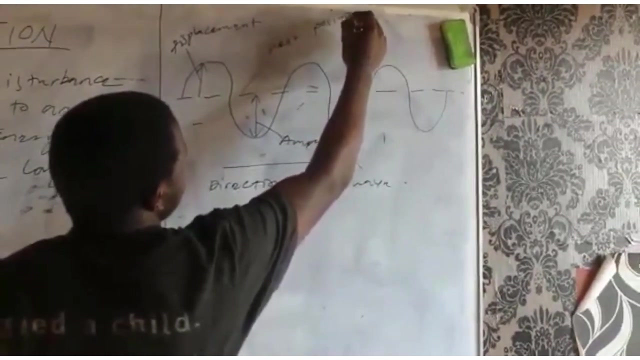 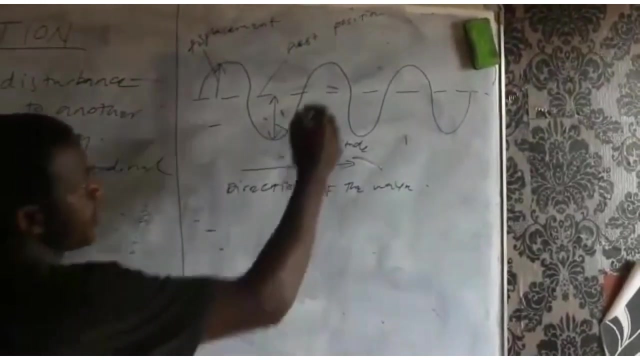 This arrow represents the displacement, Then this arrow, the point from here to here, is referred to as the amplitude. Then the dotted line is referred to as the rest position. Okay, Then the upper part of the wave here is referred to as the crest. 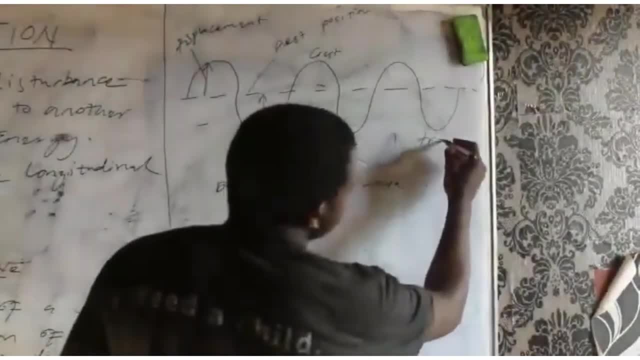 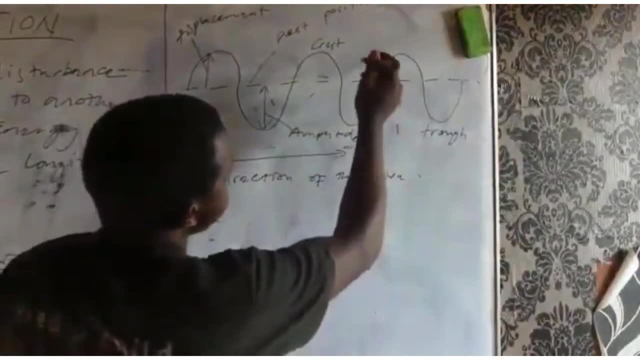 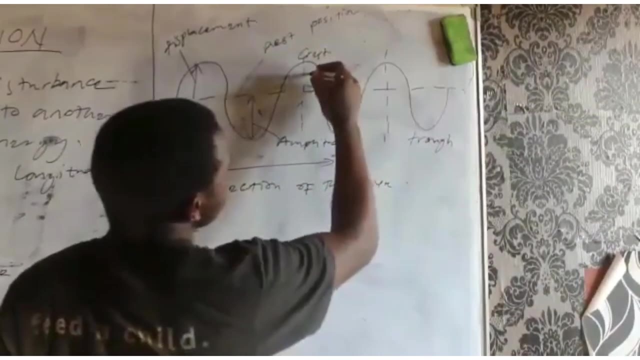 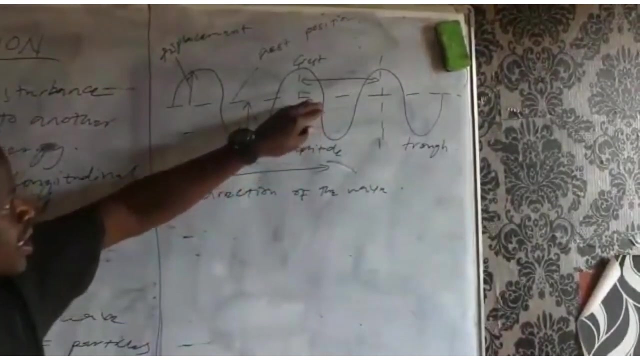 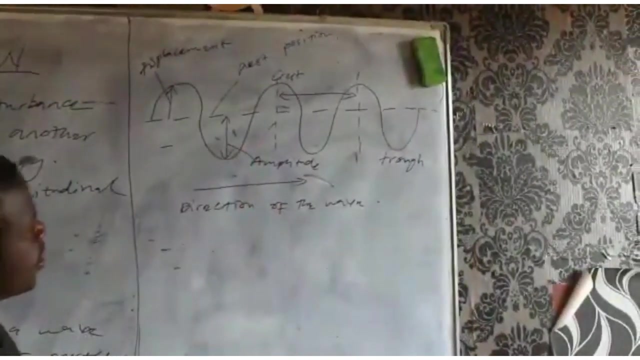 The lower part is referred to as the trough. Okay, Then the distance between two successive crests. so, as you can see, I have the crest here, I also have the crest there, So that distance is referred to as the wavelength. Okay, 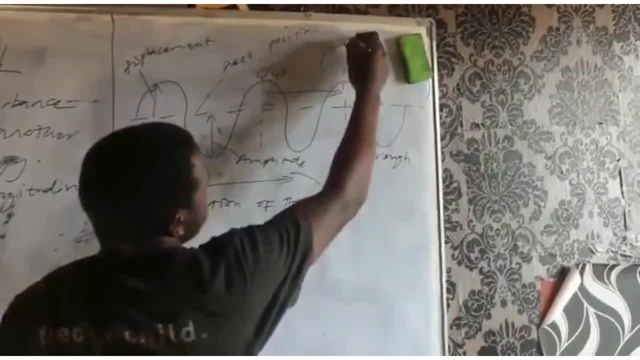 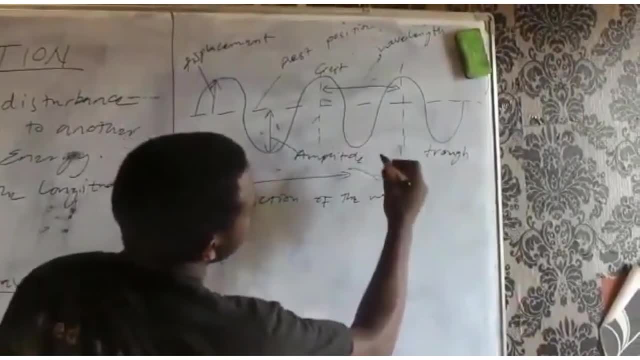 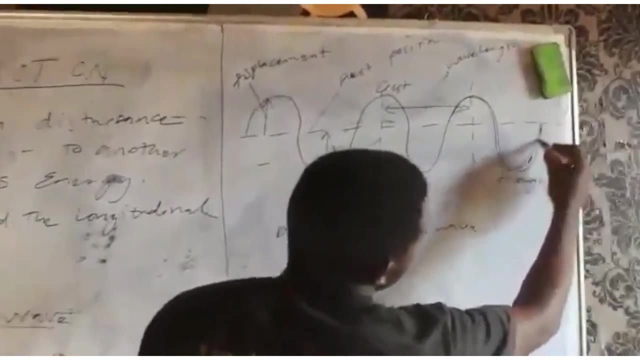 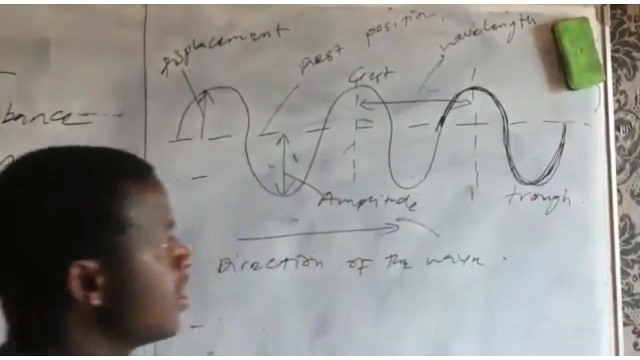 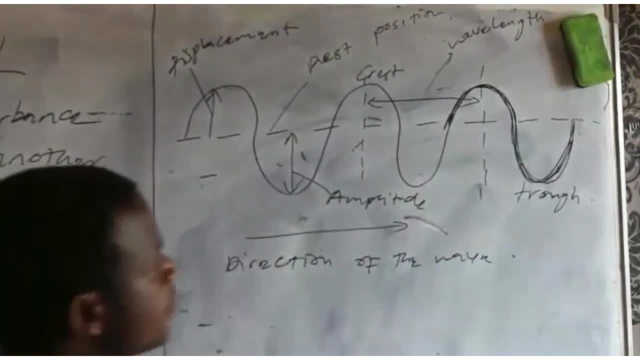 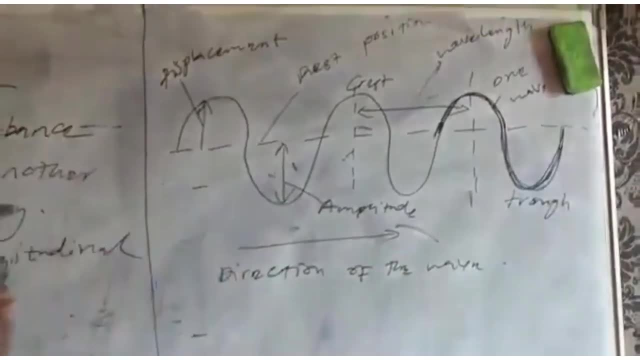 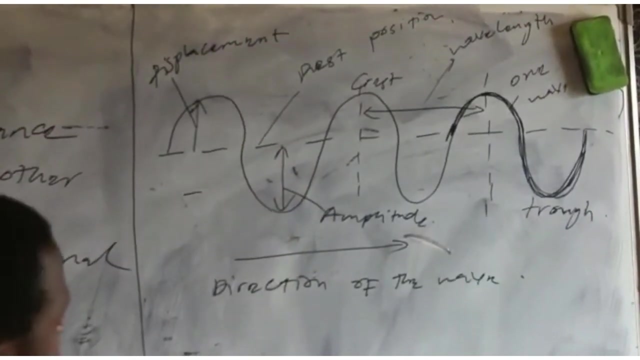 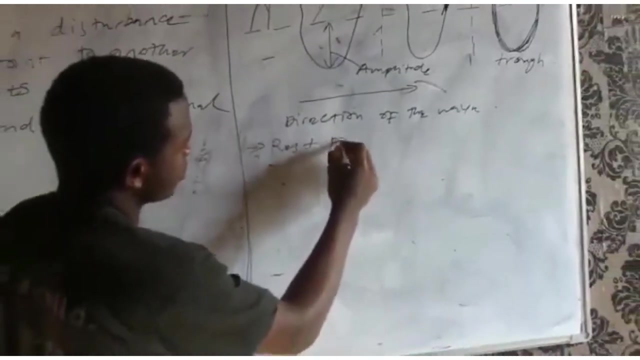 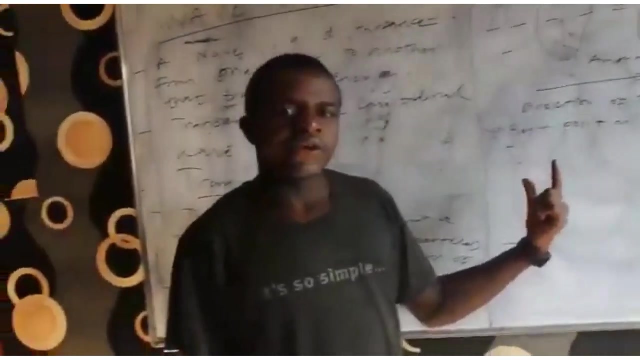 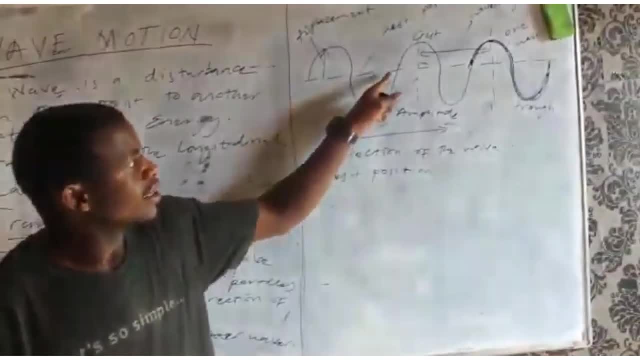 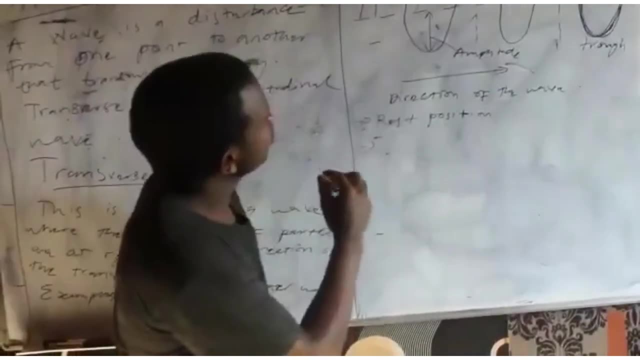 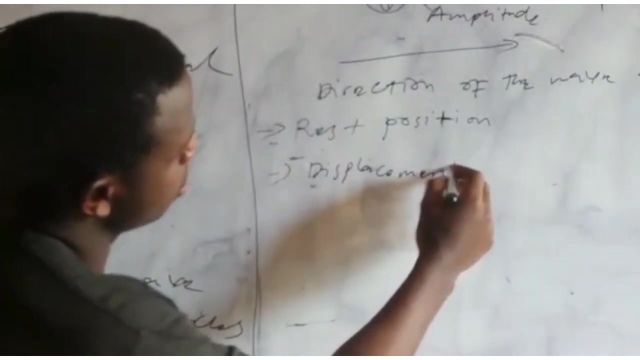 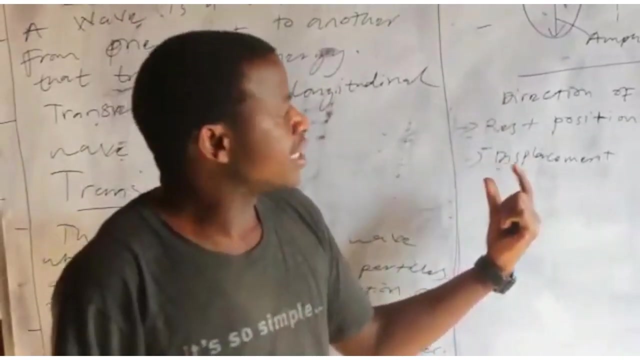 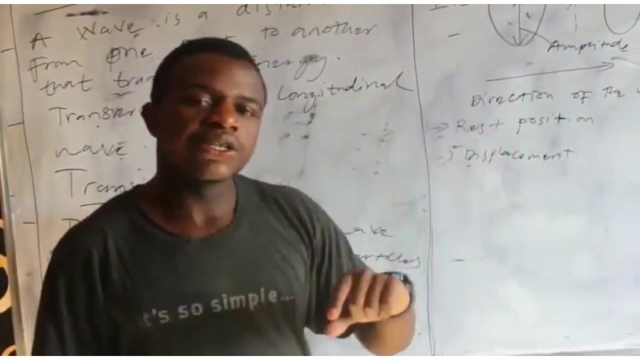 you can see this line. it shows that the particles here they don't vibrate. so that's the rest position. then to the displacement. so the displacement shows the direction and it shows the distance and the direction of the particles from the rest position. so it just shows the distance of the directional, the. 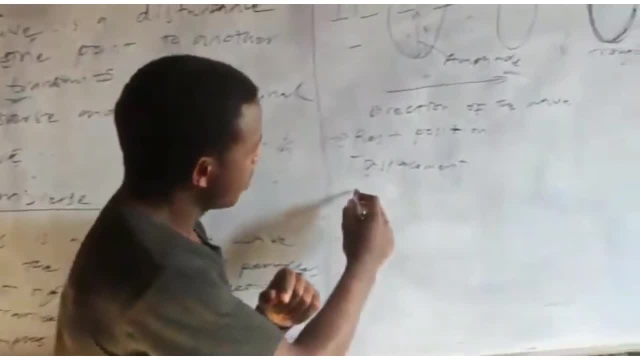 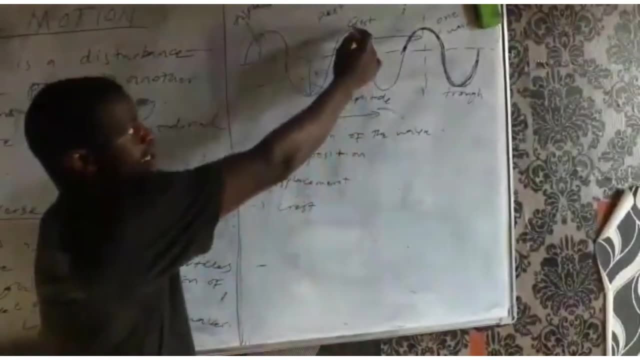 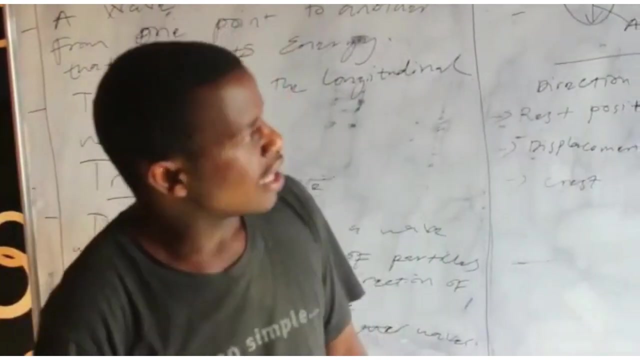 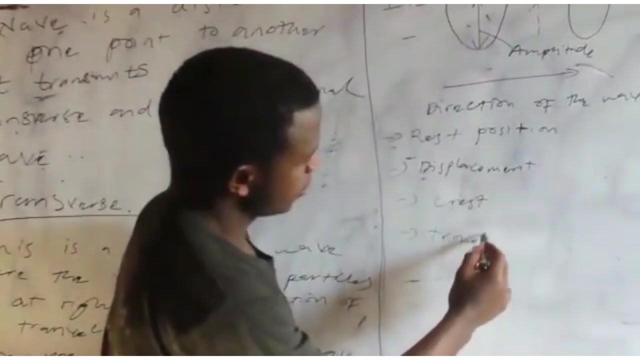 particles from the rest position. then I have the crest. so the crest, which is this part, the crest is define as the highest point of the wave, so the crest is just the highest point of the wave. then I have the trough. here the trough is defined as the lowest part of the wave. as you can see, my trough is here, so this part is one. 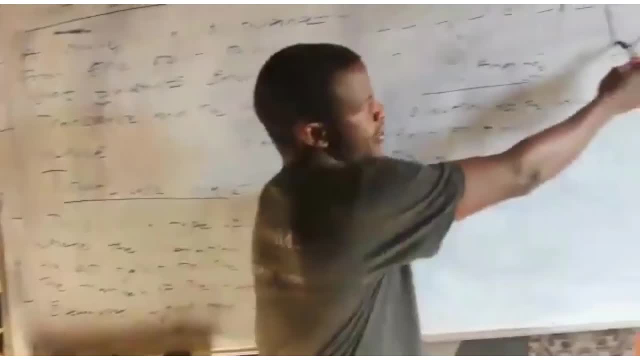 second, higher than the crest. well, an incomplete trough means that the trough here is lower than the wave, is not z stable. so then the trough is defined as the median, while left, as you can see, this is right here. and then youēve already seen that the left half plus hat is a verticalundo in this. 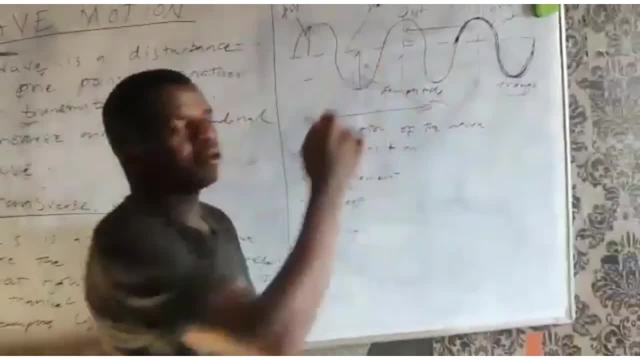 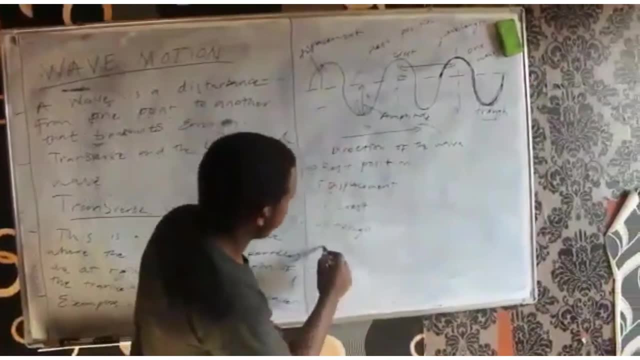 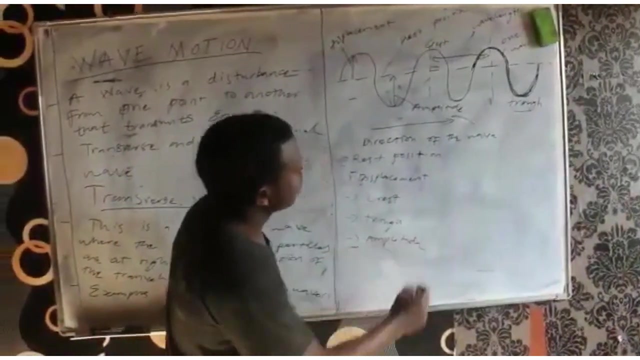 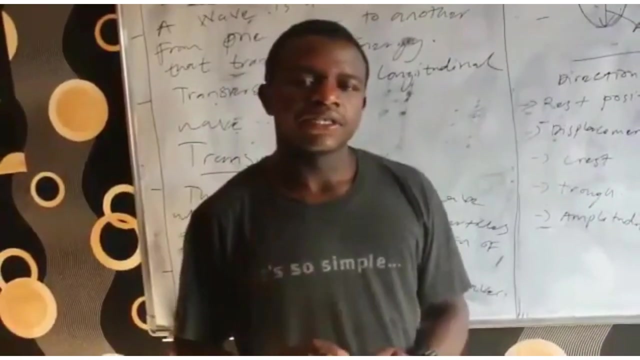 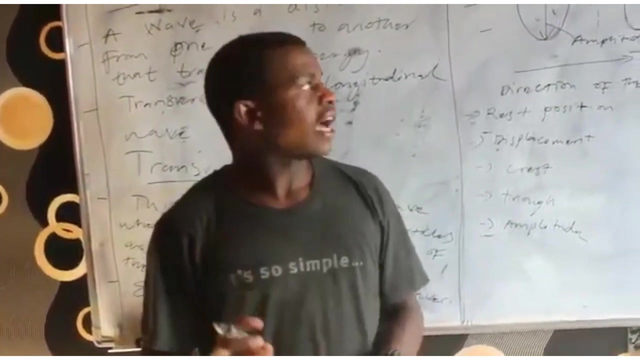 above right hand position: EVERYTHING IS B meu this part. this part may form the traps. then the other way that I have on this diagram, I have the amplitude. so the amplitude is defined as the maximum displacement of the particle from its resting position. is the maximum displacement of the particle from its rest position, that's the amplitude. then 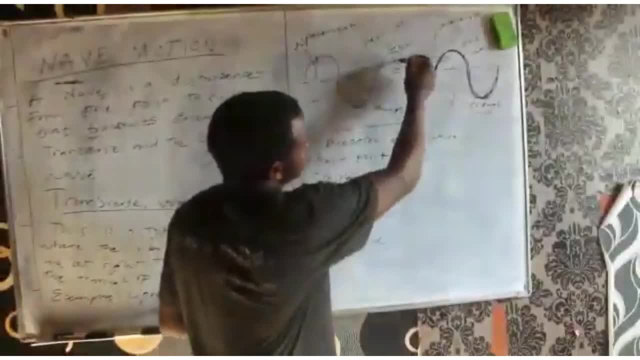 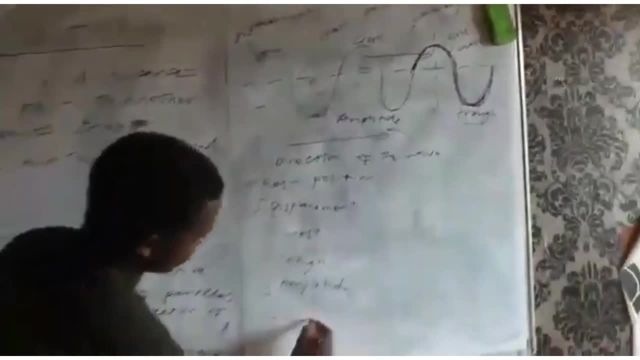 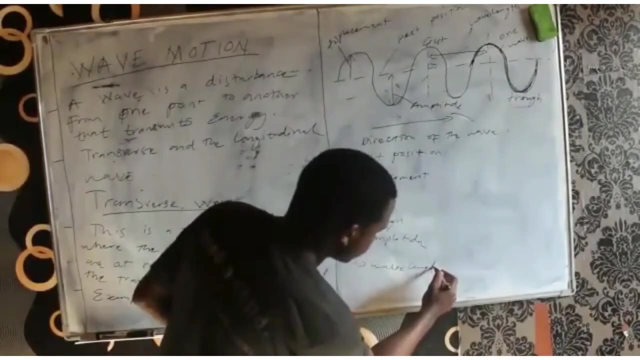 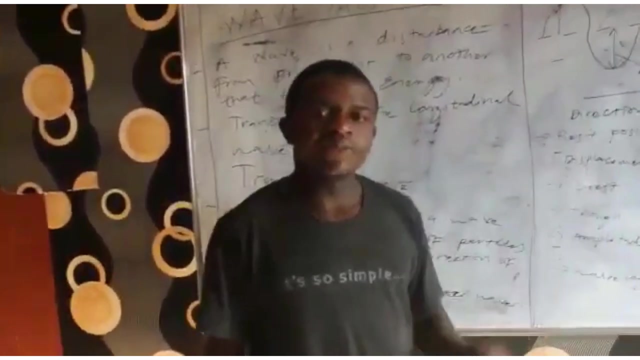 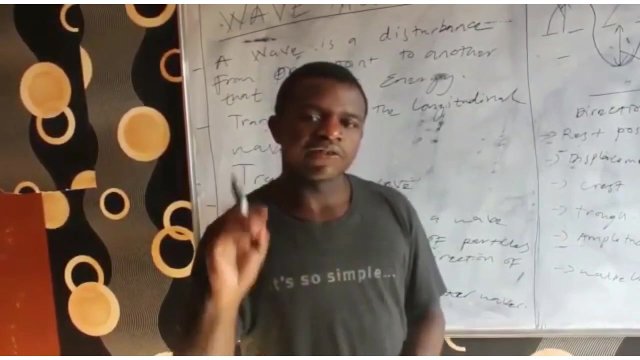 I also have the wavelength, this party, so the parts from me to here, so wavelength. so the wavelength is defines the distance between- oh oh, successive traps. is defined as the distance between two successive traps or two successive crests, and from the diagram I used my crest, this part, and 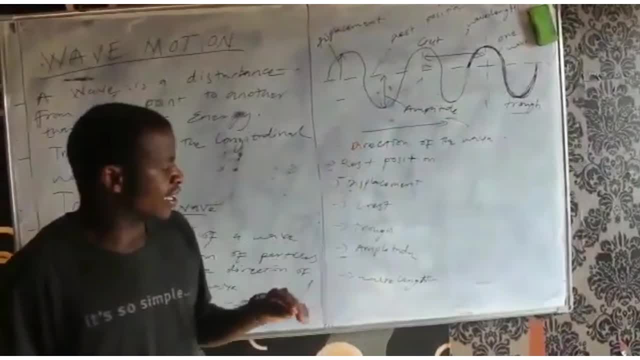 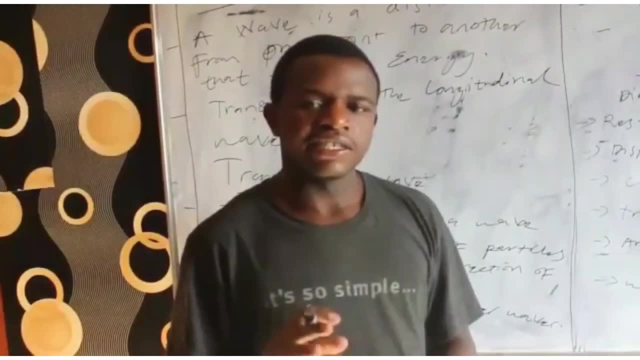 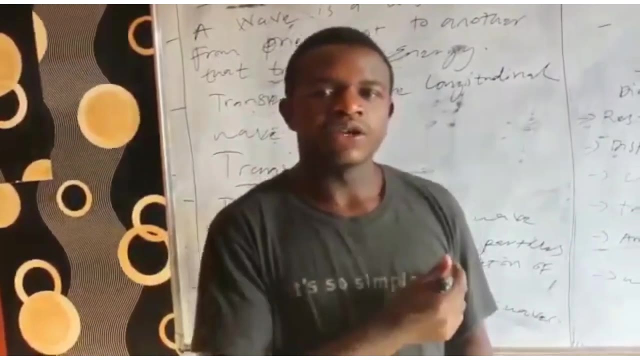 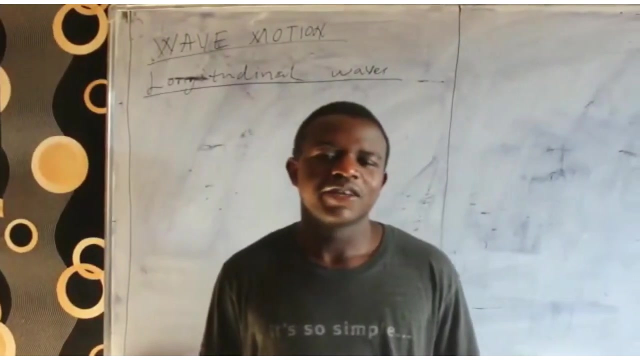 this part, but in other books the wavelength is defined as the distance in which a wave repeats itself. the distance in which a wave repeats itself. so we are going to proceed. the next thing that we're going to talk about is the longitudinal wave. the next thing that we're going to talk about is the longitudinal waves. 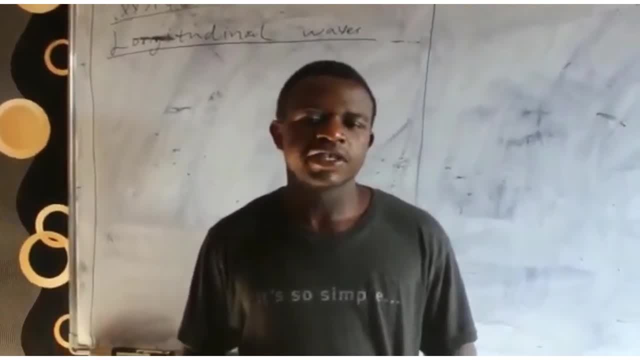 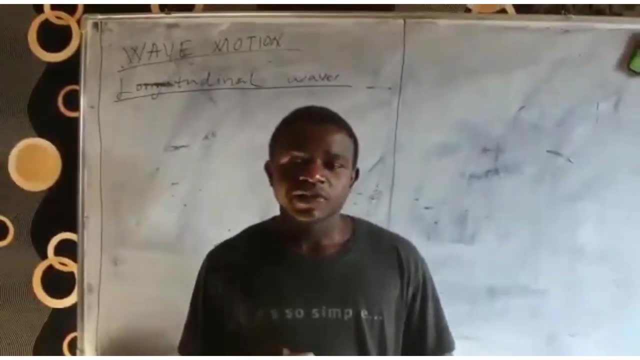 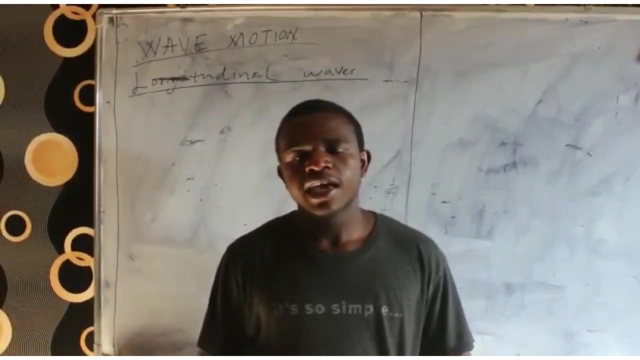 so longitudinal waves are types of waves where the vibrations of the particles are parallel to the direction of the travel of the waves. so they are defined as the types of waves where the vibration of particles are parallel to the direction of the travel the waves and the types of North Indian an. 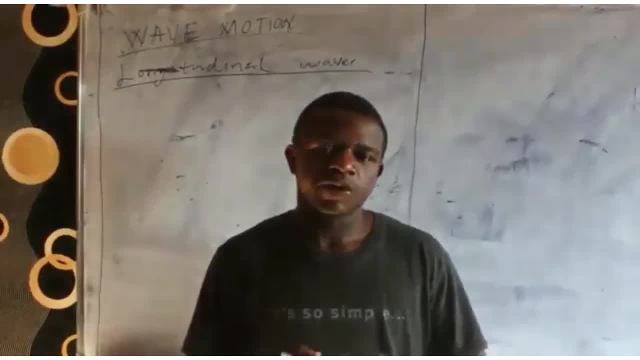 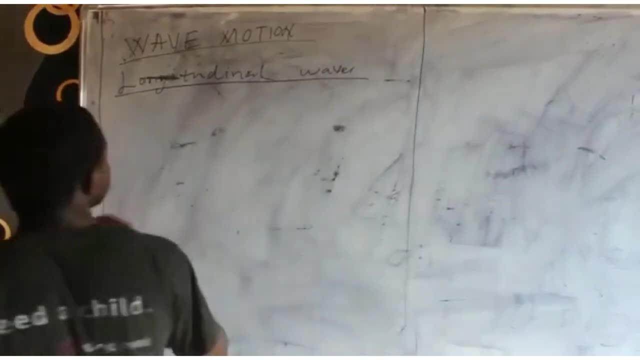 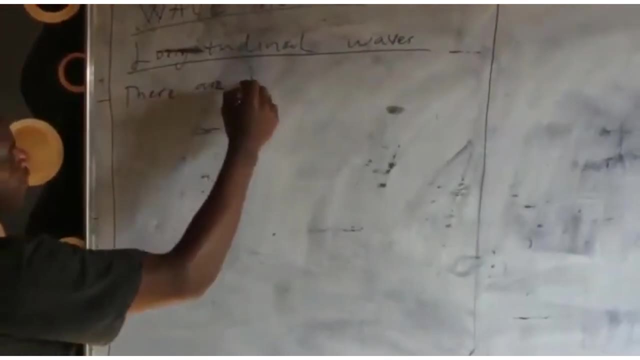 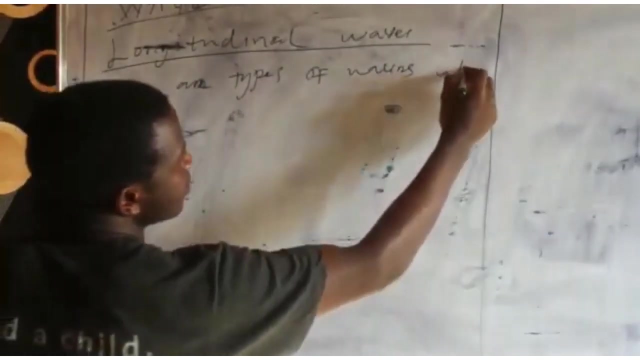 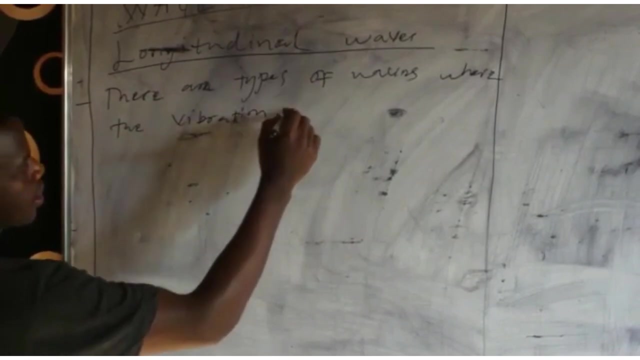 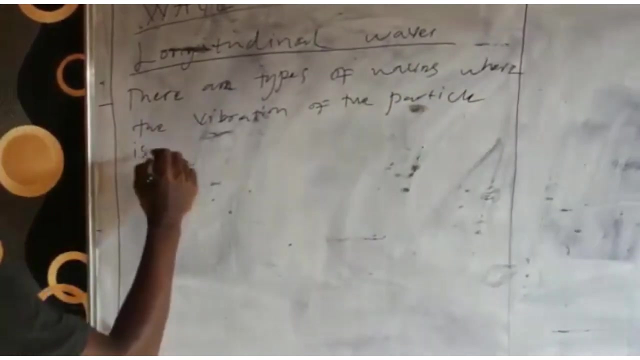 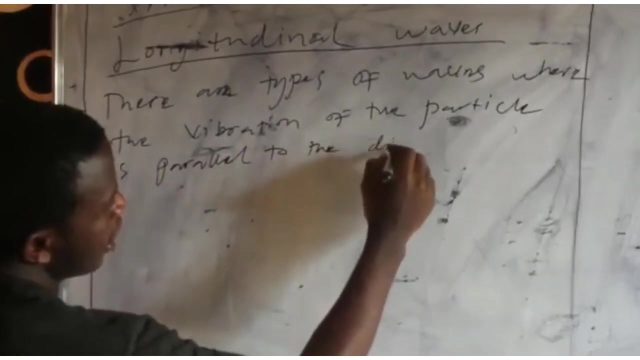 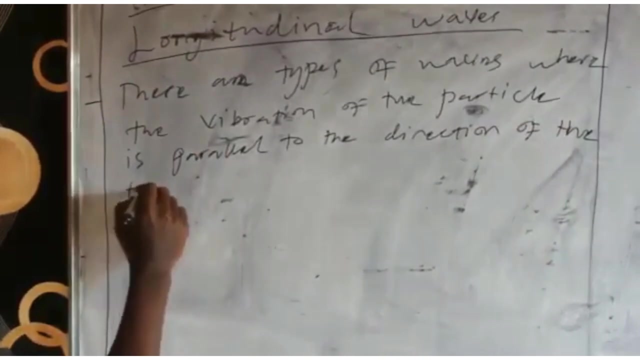 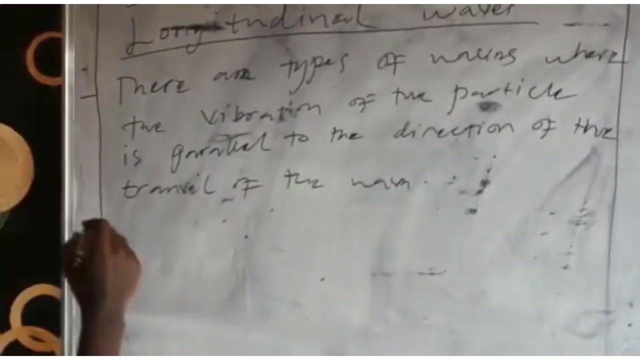 waves, we have the sound waves and the extreme waves, so let me just write this definition on the board. so the longitudinal waves these are. these are types of waves where the vibration of the particle is parallel to the direction, direction of the travel of the web. then examples of longitudinal waves: we have examples. 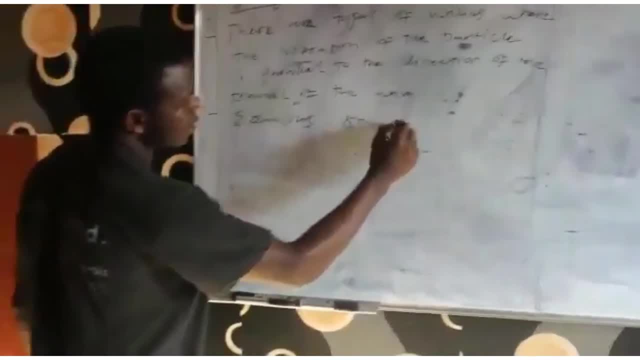 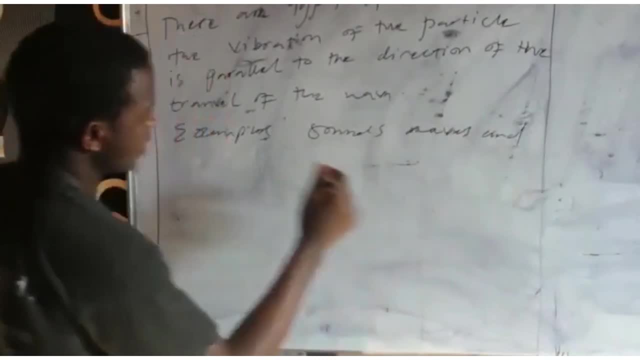 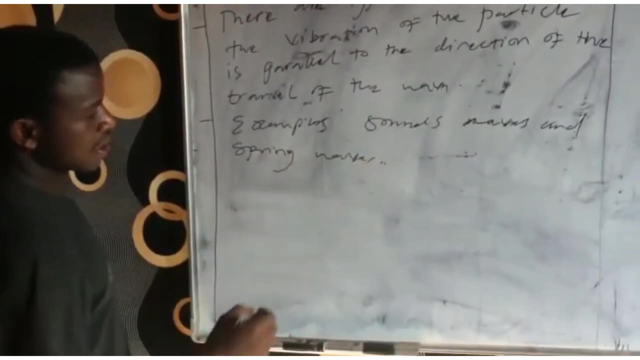 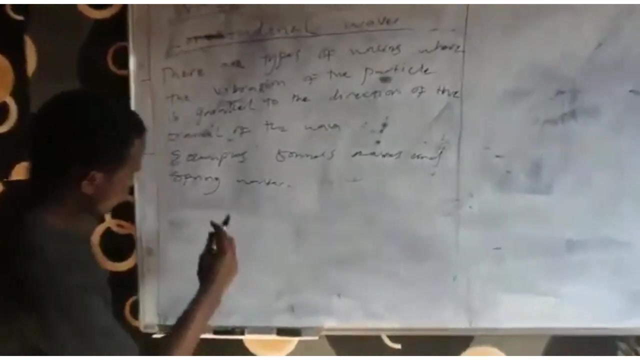 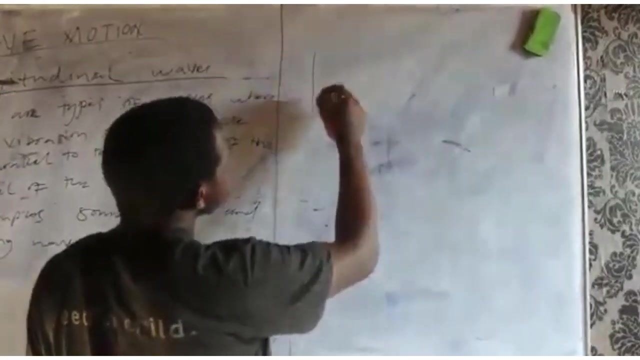 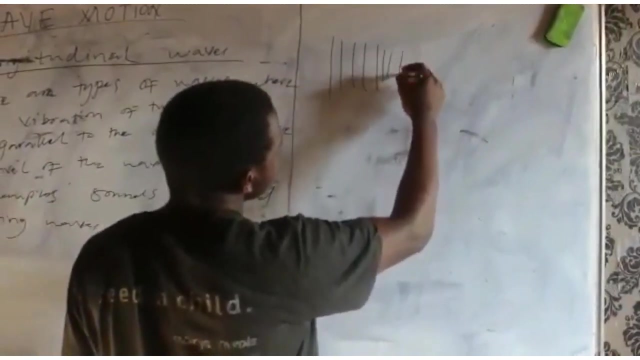 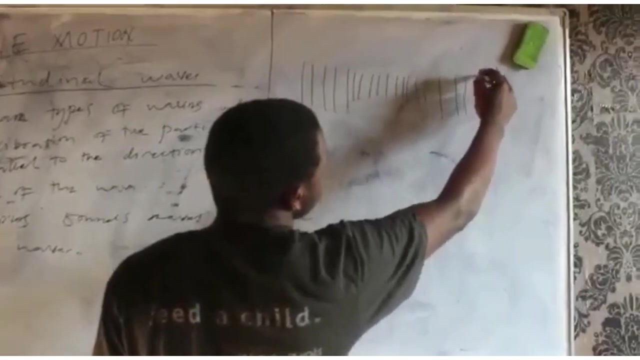 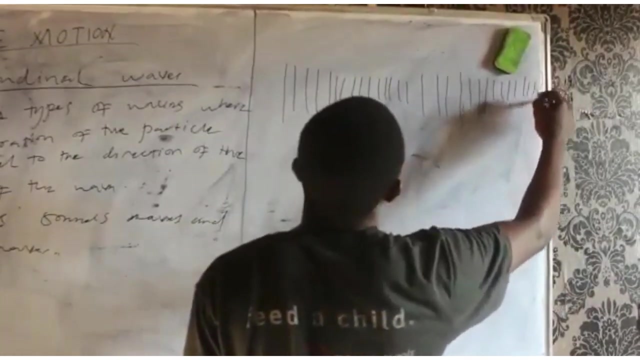 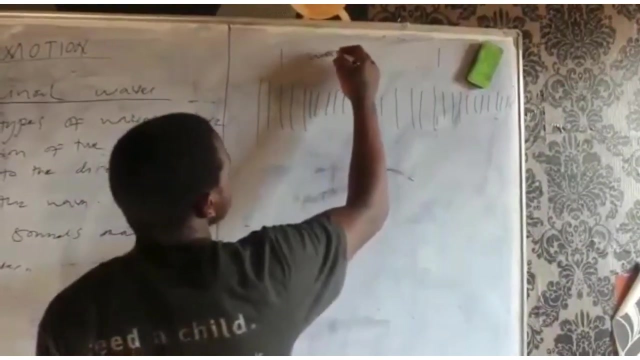 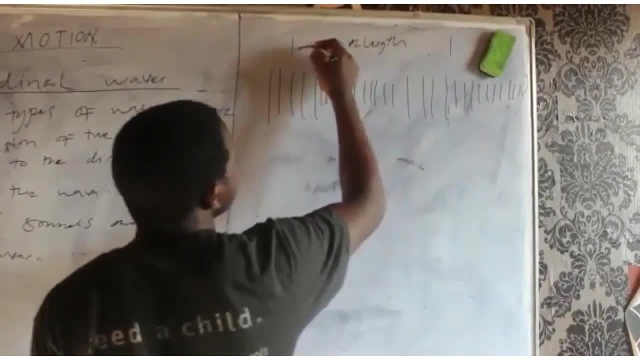 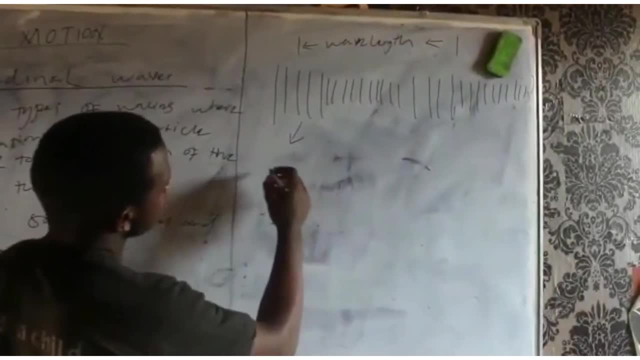 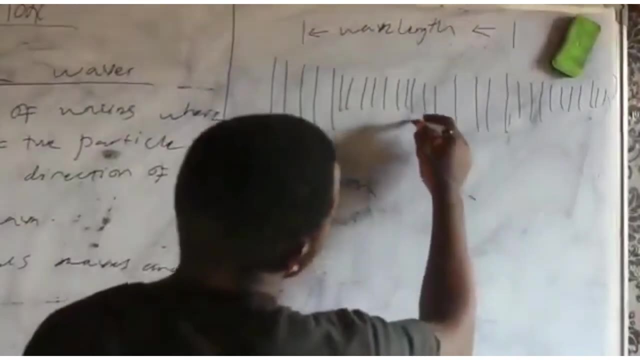 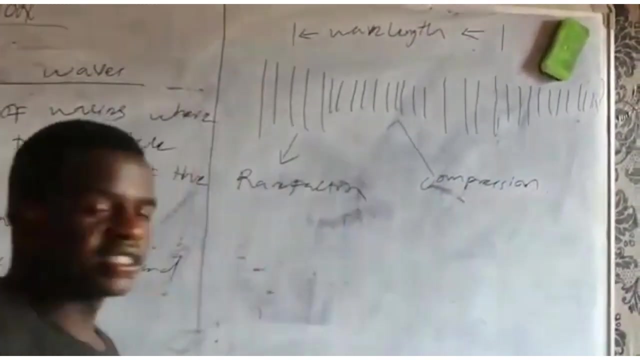 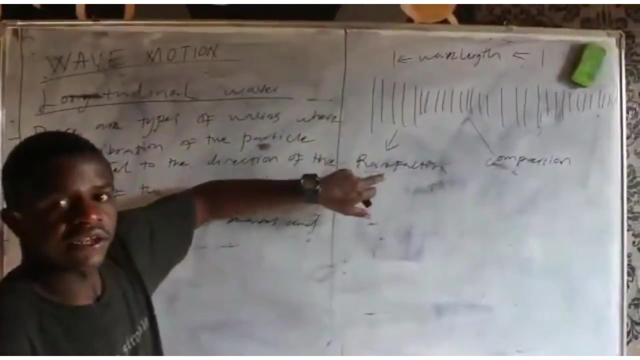 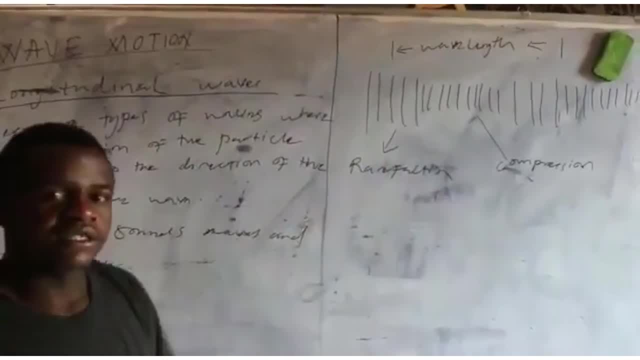 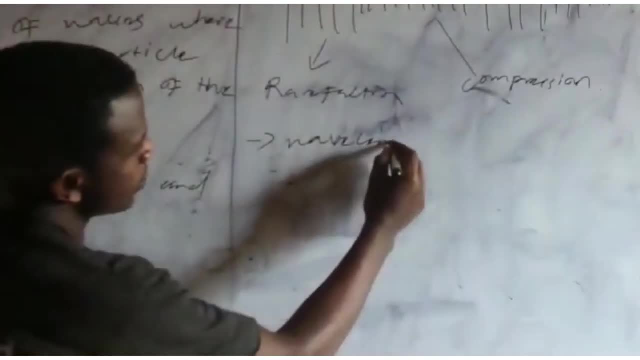 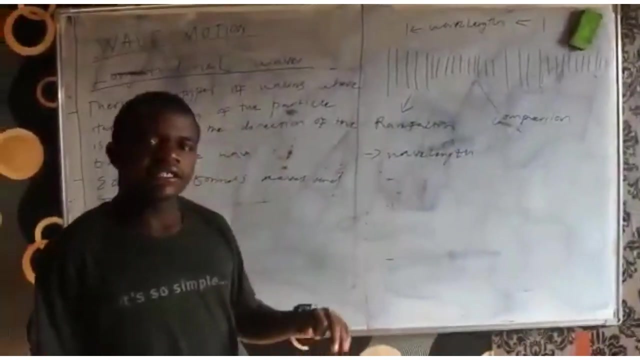 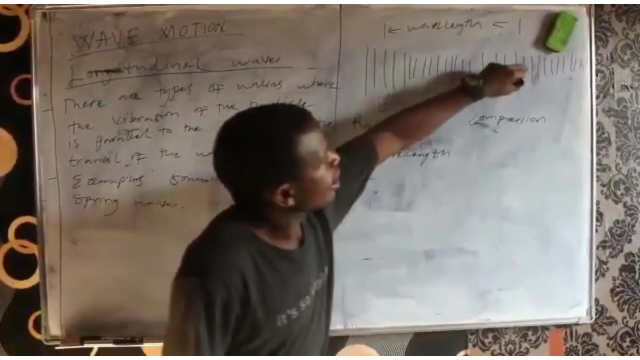 to us the wavelength. so let's look at the definitions of these weights. so the first weight of the wavelength. so the wavelength is defined as the distance between two successive real functions. so, as you can see, we have a real function here and the real function so it's the distance between two successive real 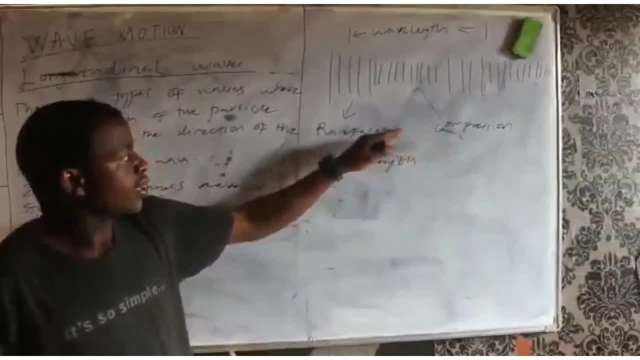 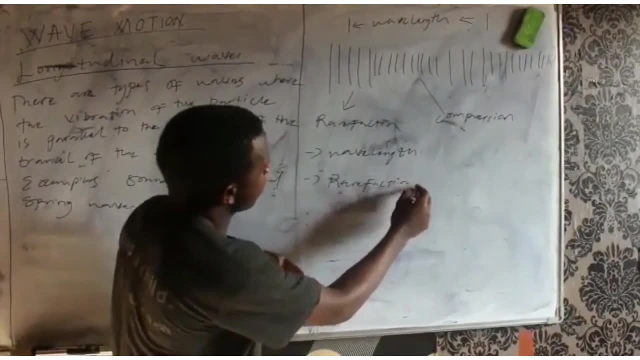 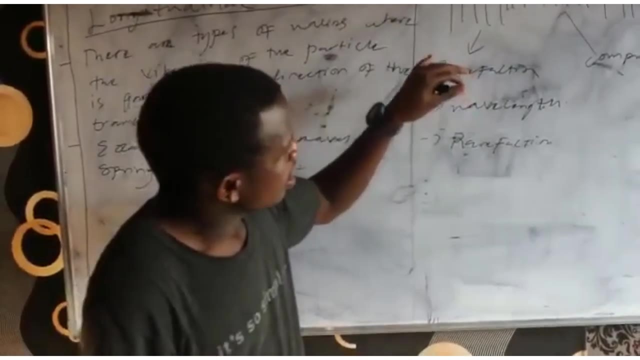 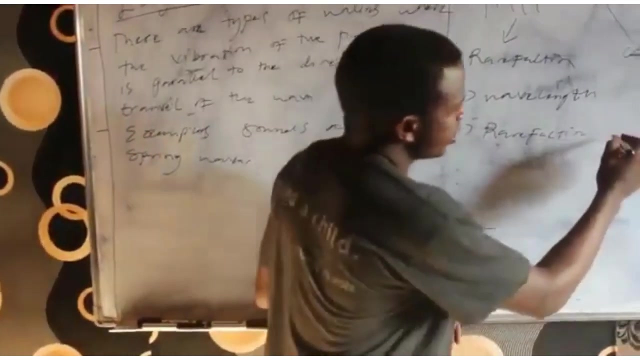 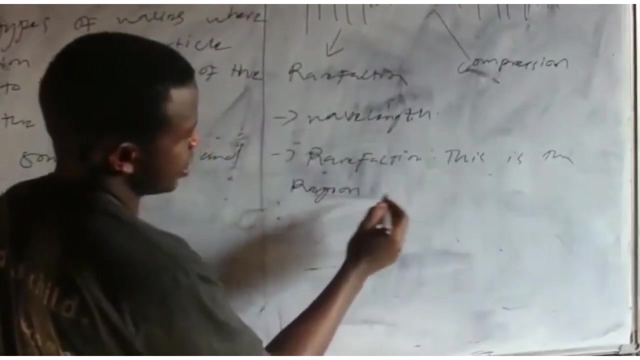 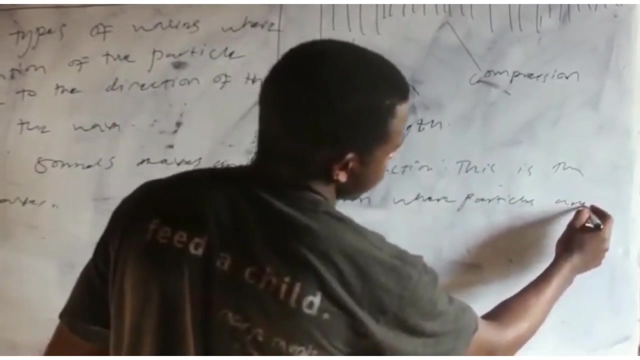 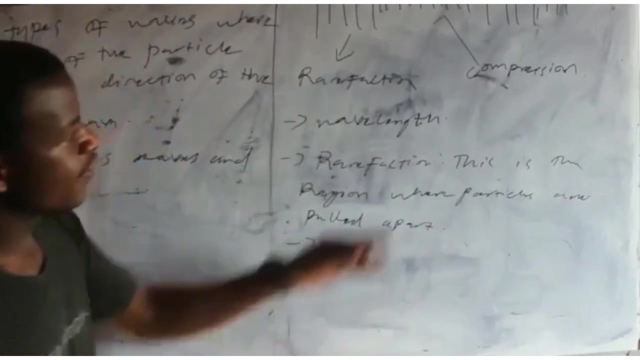 function. then what about the? the weight, real function, so, real function. this is a region where the particles are not close together. the particles are put apart. so this is where they reach. this is the region. this is the region where particles are put apart. then we also have the. 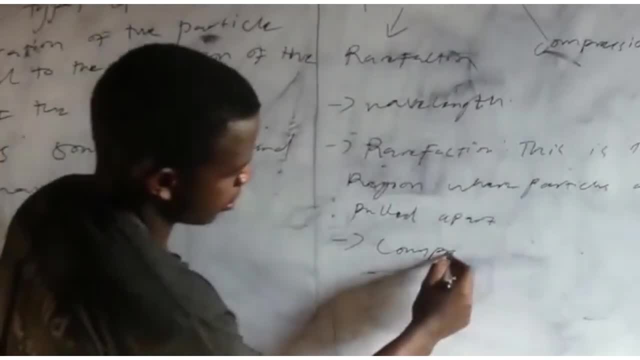 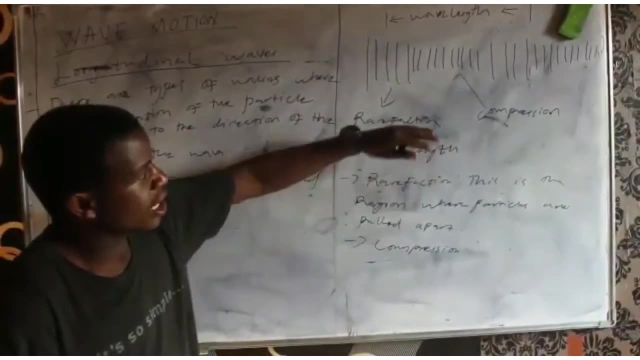 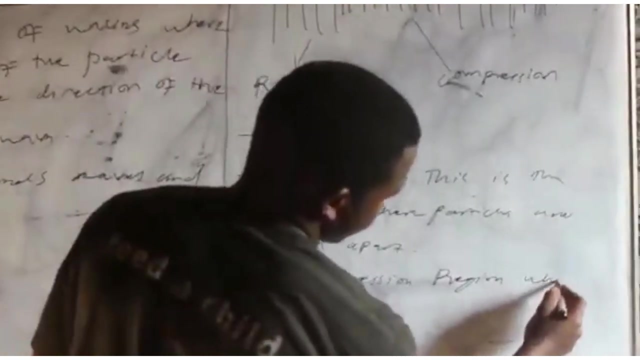 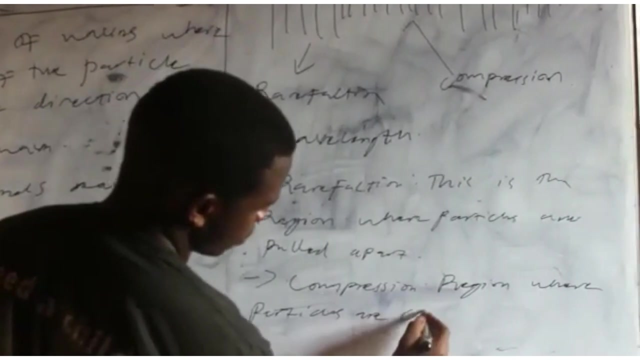 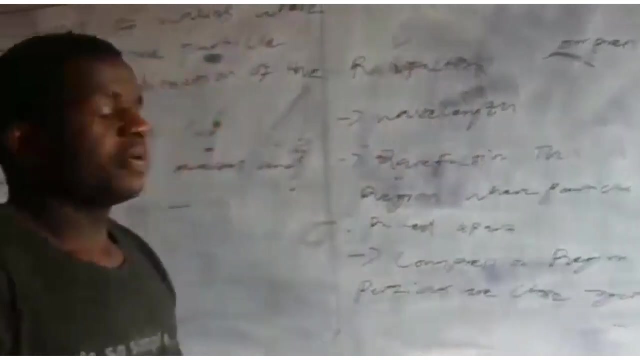 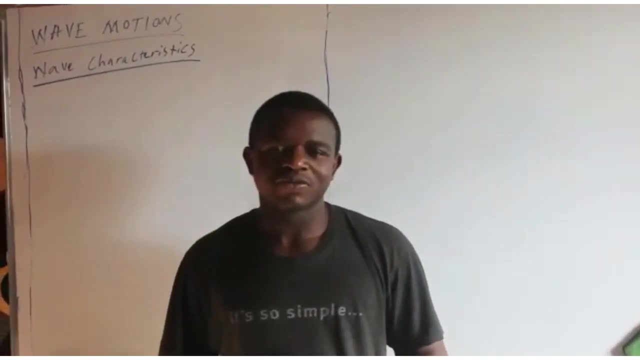 compression. the compression is defined as the region where the particles are closer together, so the region we have particles. so next time we are going to proceed on wavelength. thank you very much. so today, in wave motion, we're going to proceed. we're going to look at the 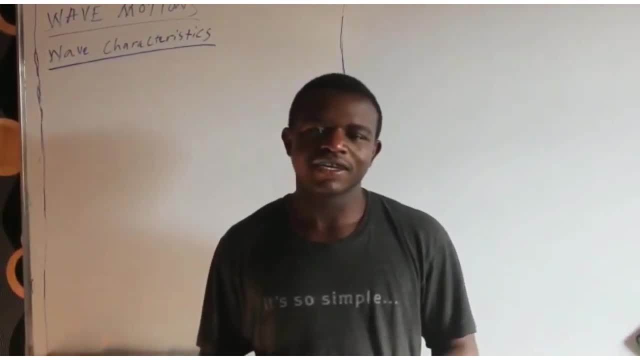 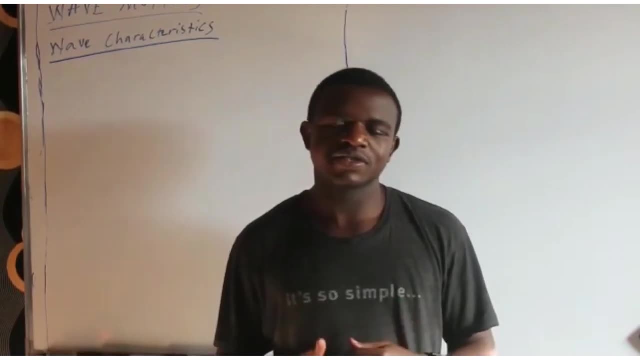 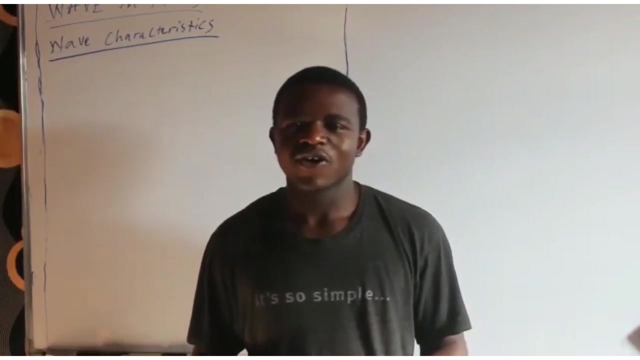 characteristics of waves. and last time we defined what waves are and we talked about two types of waves. we said that types of waves we have- transverse waves and longitudinal waves. so today we're going to proceed. we're going to look at the characteristics of waves, so waves that are produced by a continuous 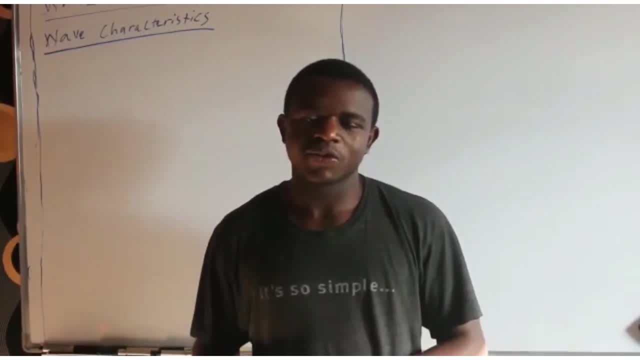 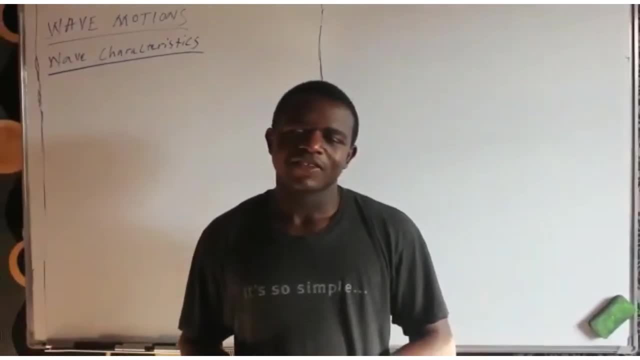 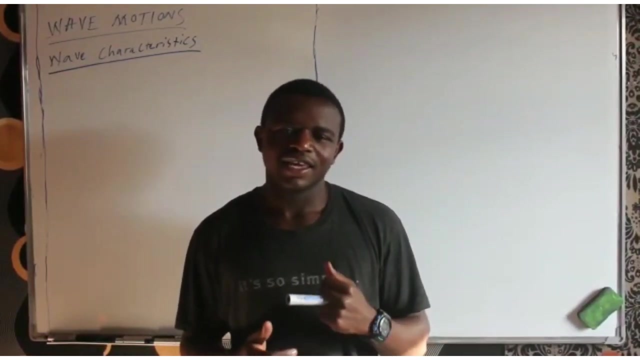 vibrating object are referred to as periodic waves. and these periodic waves, they have the amperage of the waves, and the amperage of the waves is the amplitude, the wavelength, the frequency and the period. so, periodic waves, they have the amplitude, the period, the frequency and the wavelength. so what is? the wavelength. the wavelength is defined as the minimum distance at which a wave repeats itself, and wavelength is measured in meters, and the symbol for is lambda, which is a Greek letter. then we're going to go to the amplitude. so what's the amplitude? the amplitude is defined as the maximum displacement of. 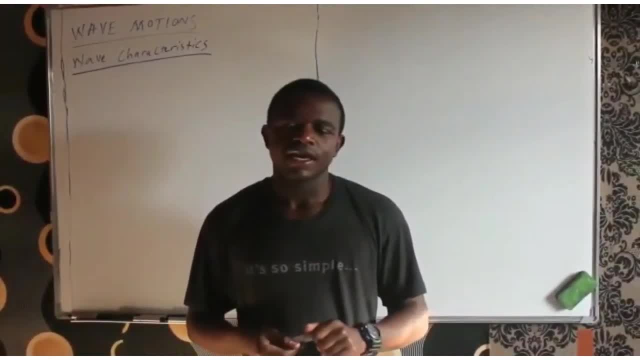 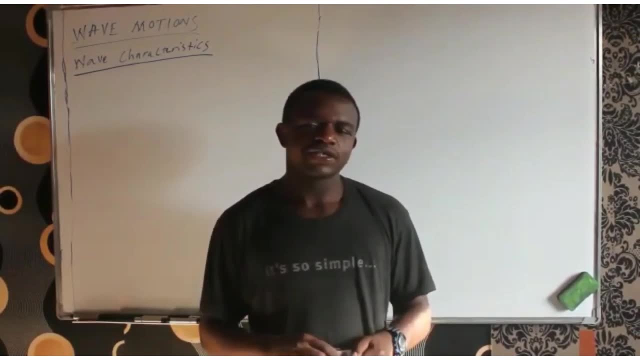 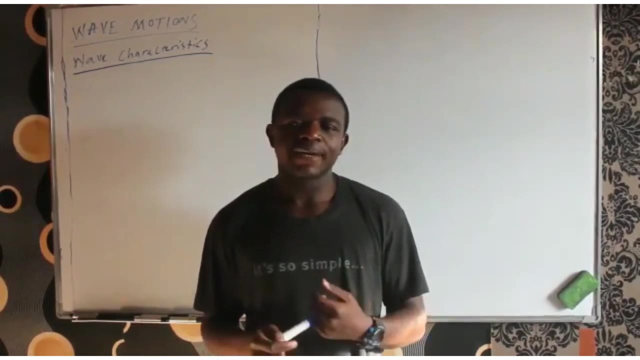 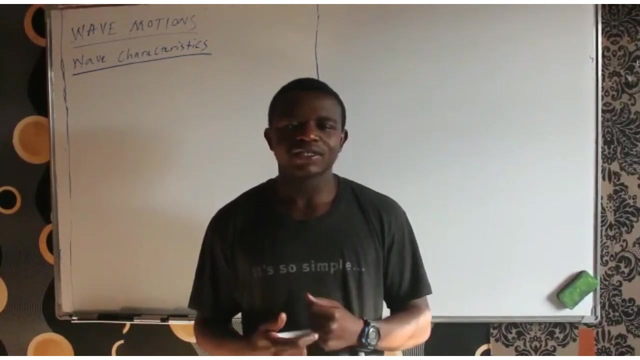 the particle from its rest position and amplitude is represented by the symbol M. then going to frequency, so what's frequency? frequency is defined as the the number of waves that are passing through a setting point: Two seconds. so these are the number of waves that are passing through a certain point per second two. 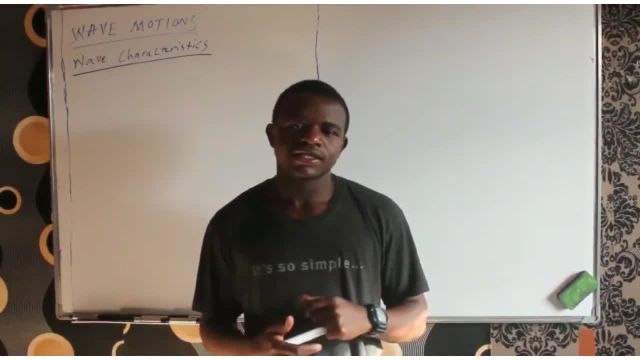 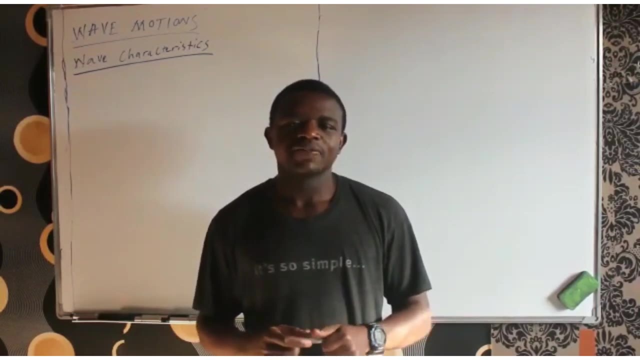 and frequency's measured in has, and this is H and a, Z and the symbol of frequency's, F. then we go to the next one, which is a period. so what's period? period is defined as the time taken and its probability. so what's the amplitude of theboynd? did you notice that's covered with. 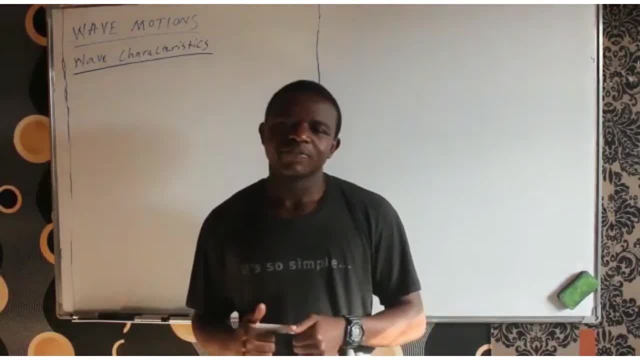 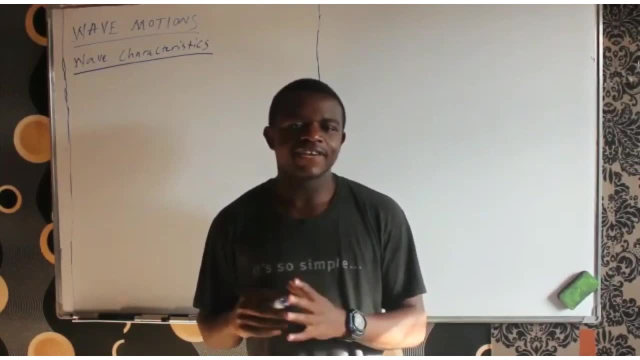 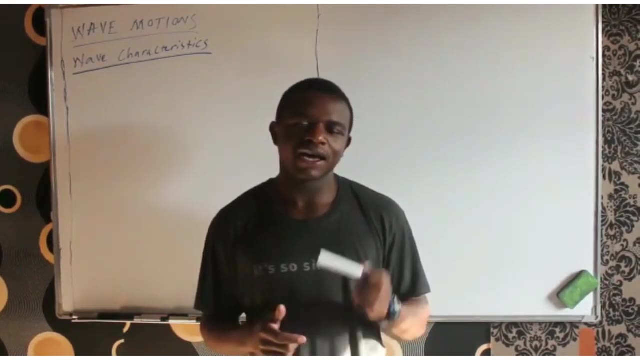 for one complete wave to be formed, and the symbol of period is capital letter T. and period is also defined as the inverse of frequency. So when calculating period you can say period is equals to one divided by frequency. So let me just write these notes on the whiteboard. So I've said: 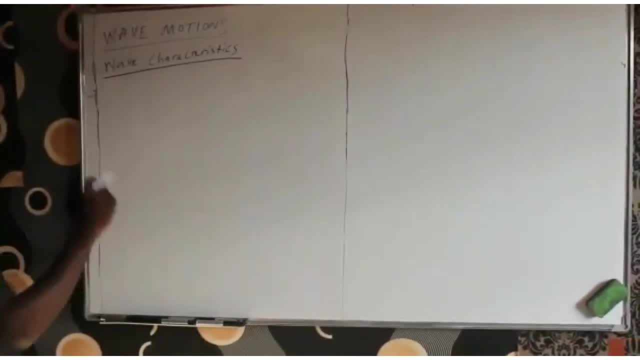 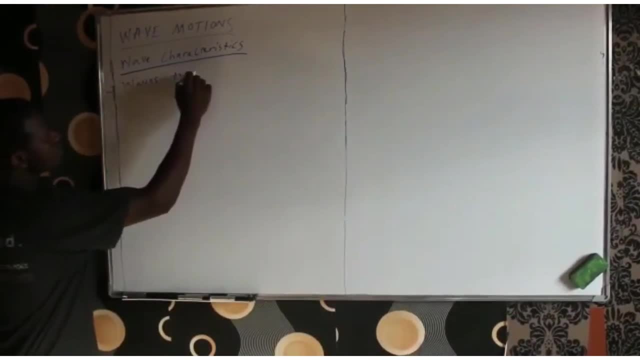 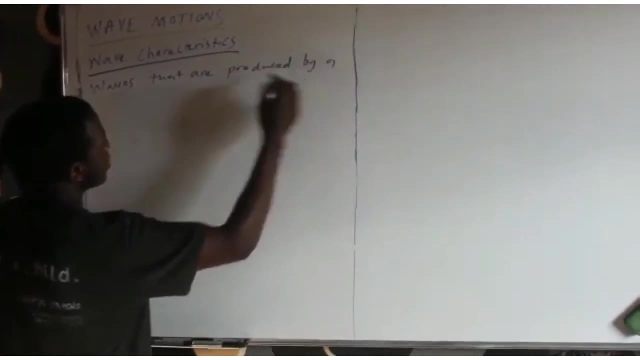 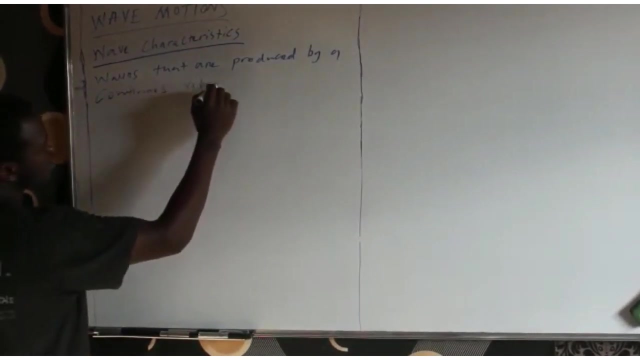 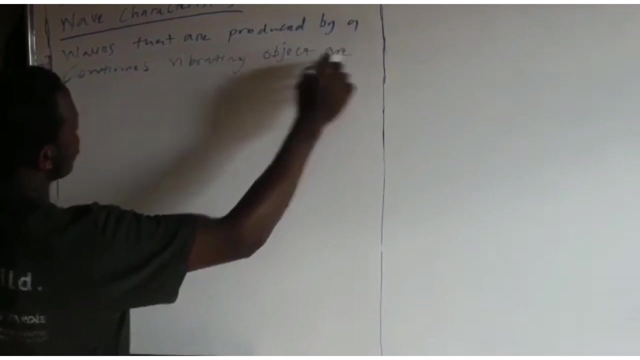 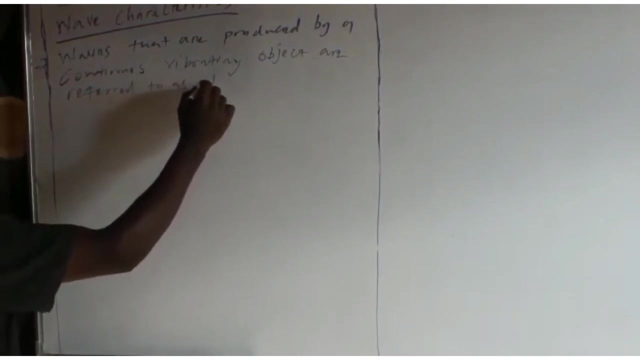 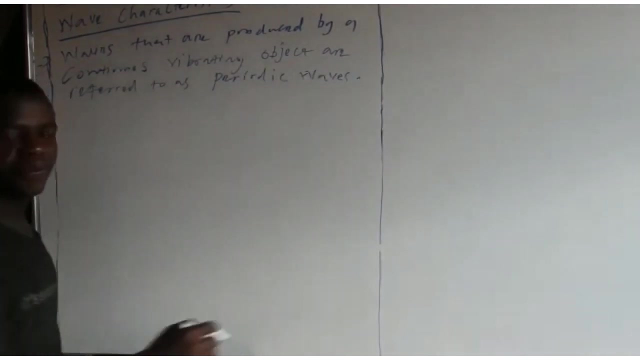 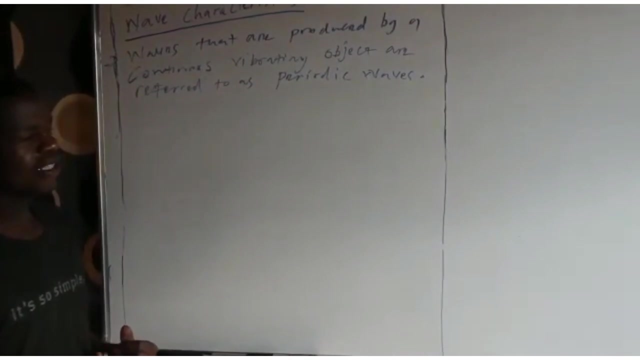 waves that are produced by a continuous vibrating object are referred to as periodic waves. So waves that are produced by a continuously vibrating object are referred to as periodic waves. And these periodic waves, they have the amplitude, wavelength, frequency, and frequency and period. So the periodic waves. 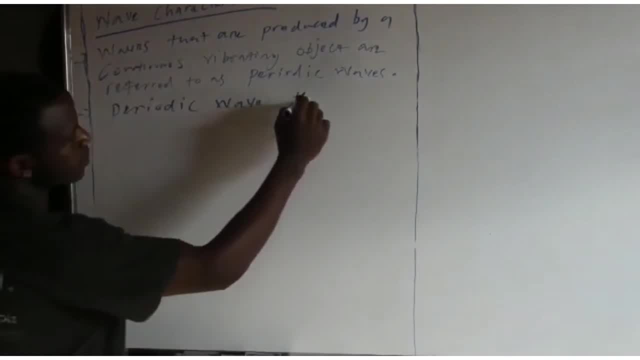 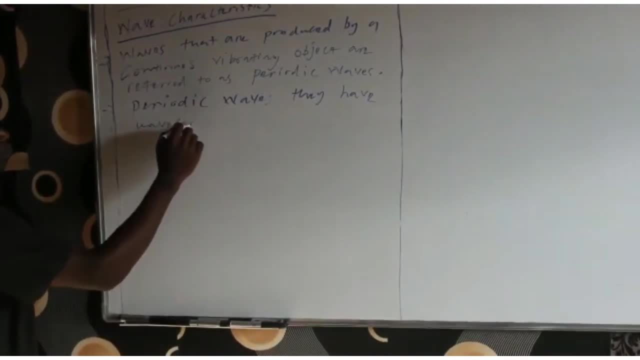 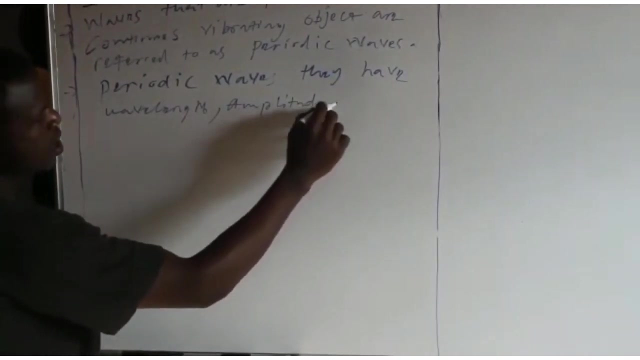 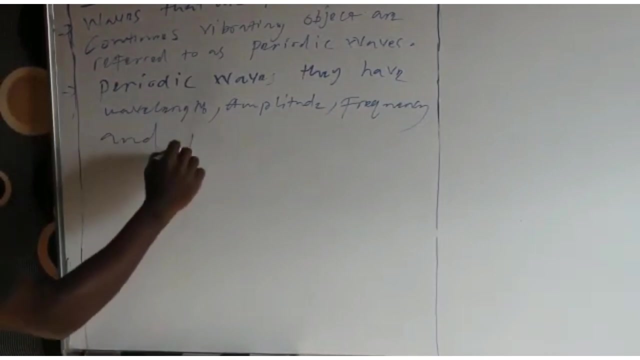 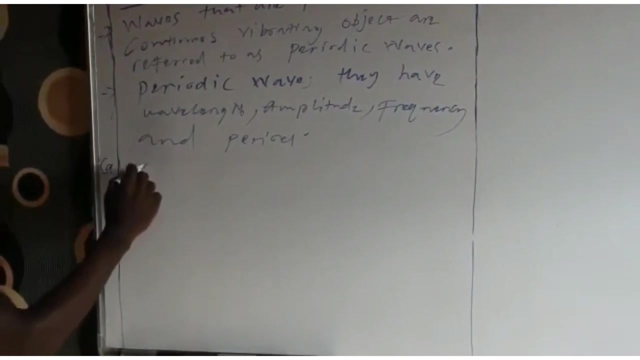 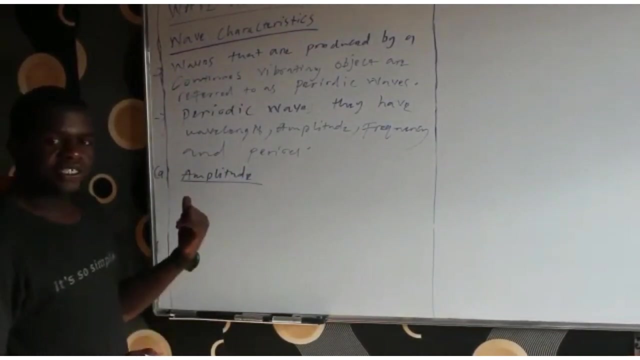 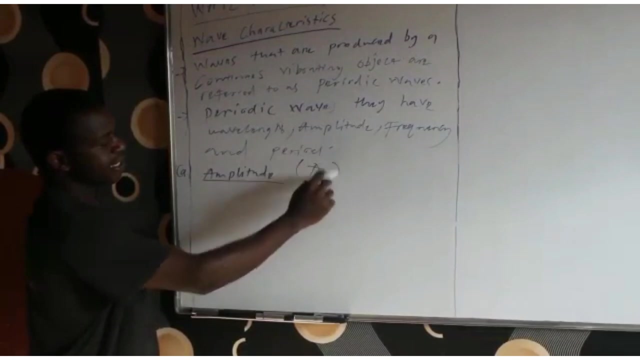 they have the wavelength, the amplitude, the frequency and period. So we start with the amplitude. So the amplitude is defined as the maximum displacement of a particle from its rest position, and the symbol of amplitude is capital letter A. So this is the maximum. displacement, We go to wavelength. So what's the definition of wavelength? Wavelength is defined as the maximum distance at which a wave repeats itself, And the symbol of wavelength is a Greek letter which is lambda, and wavelength is measured in meters. So wavelength is the minimum distance at which a wave repeats itself. 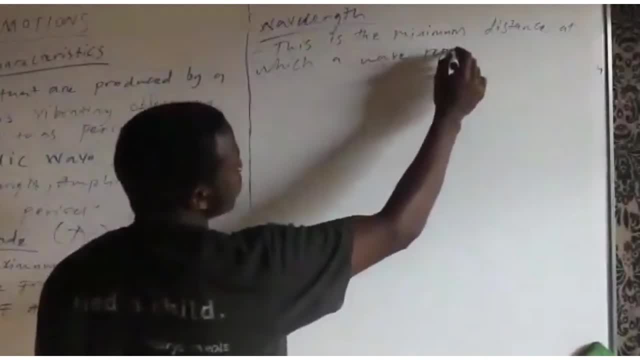 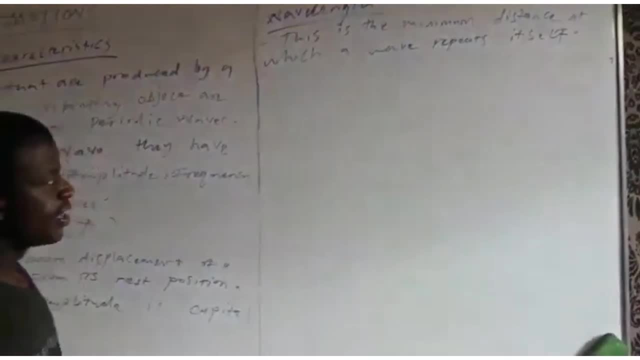 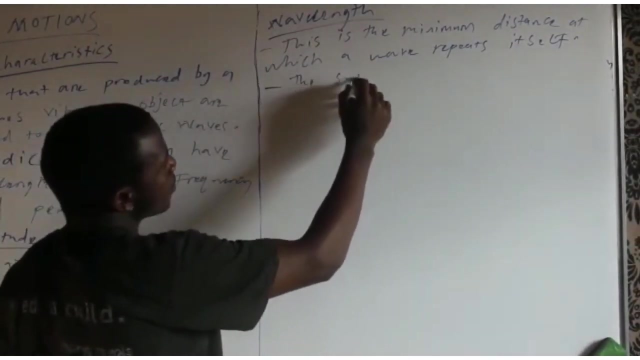 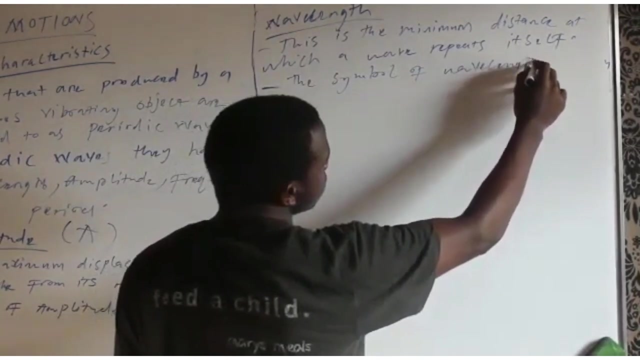 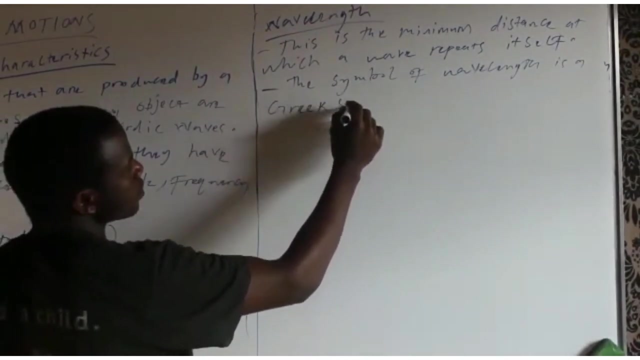 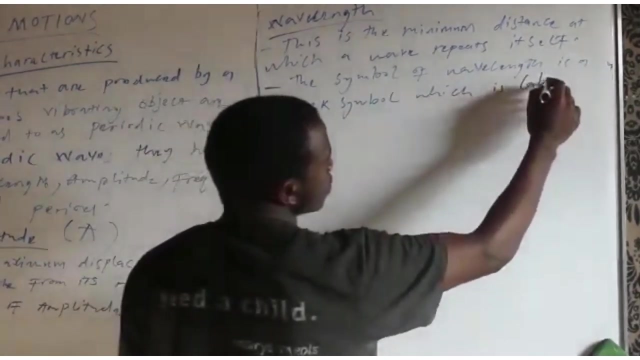 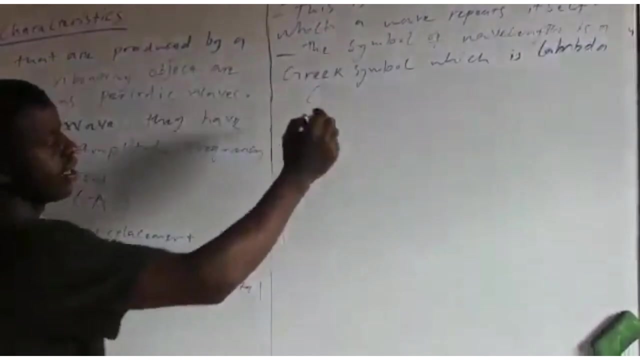 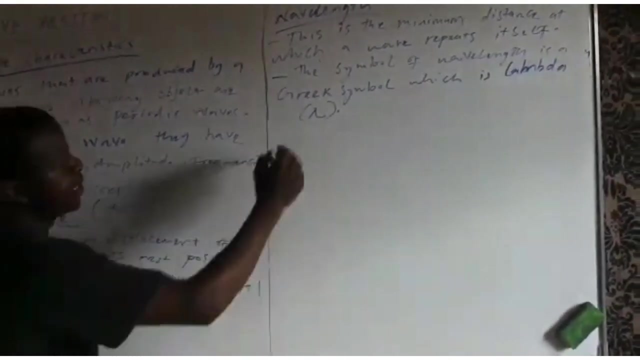 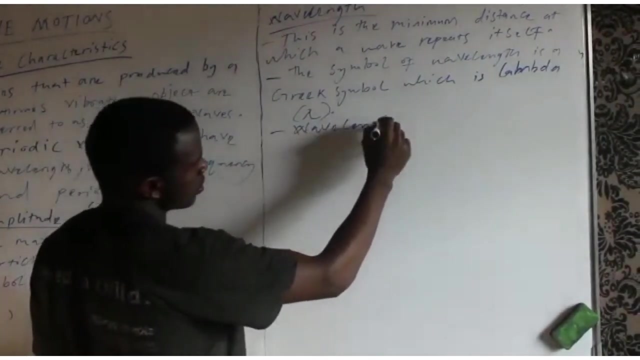 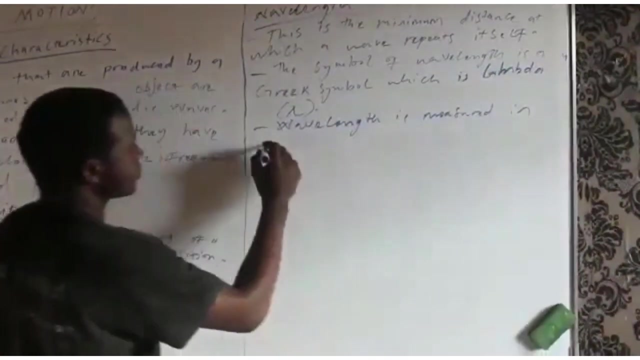 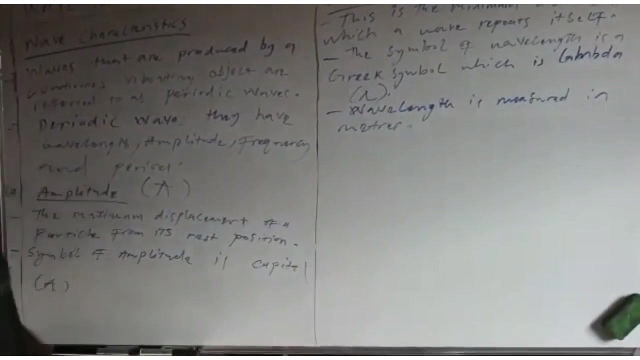 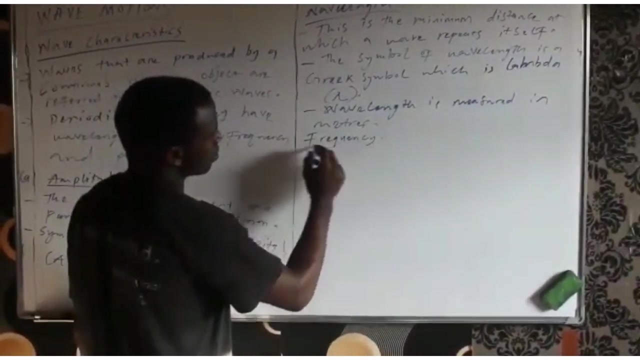 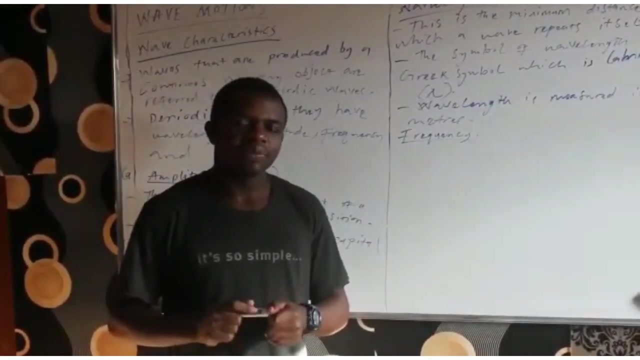 Then the symbol of wavelength is a Greek letter, which is lambda, So lambda is given like this: this is the symbol of lambda, And the units of wavelength are meters, So wavelength is measured in meters. We proceed, we look at frequency, So frequency is defined as the number of waves that are passing through a certain point per. 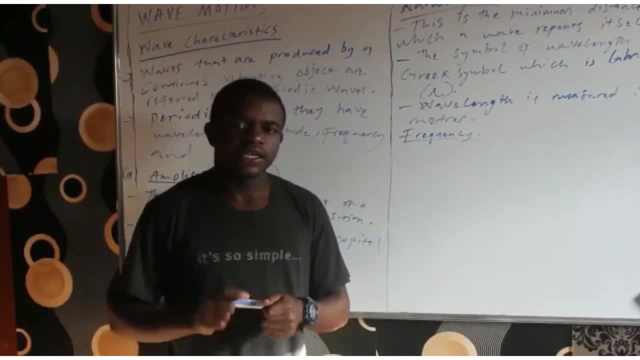 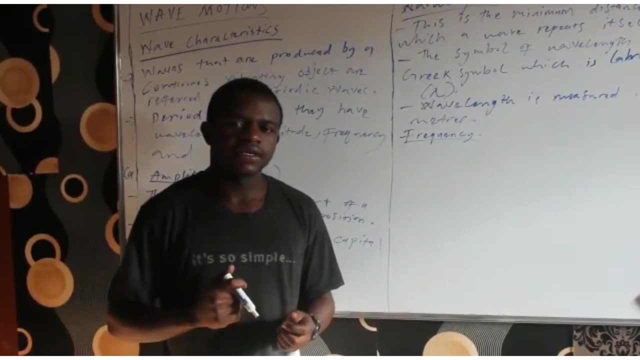 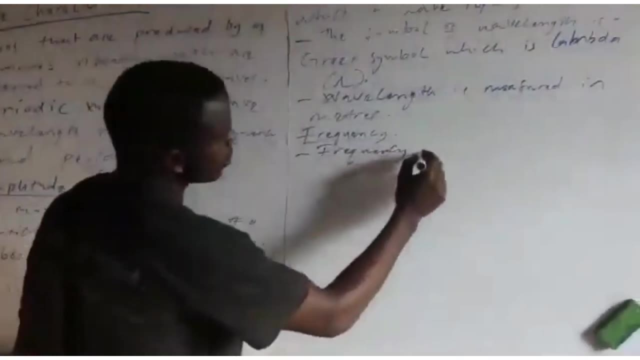 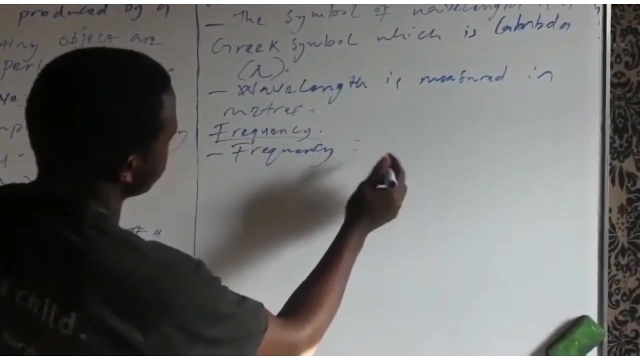 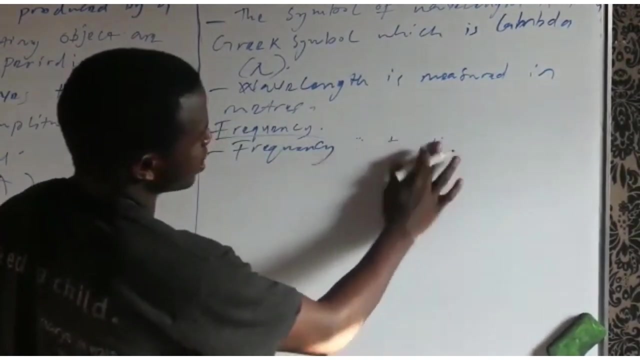 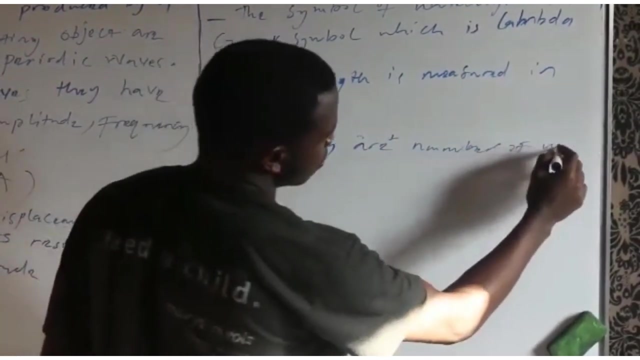 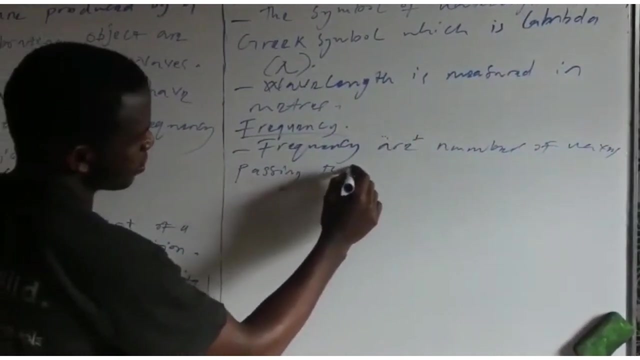 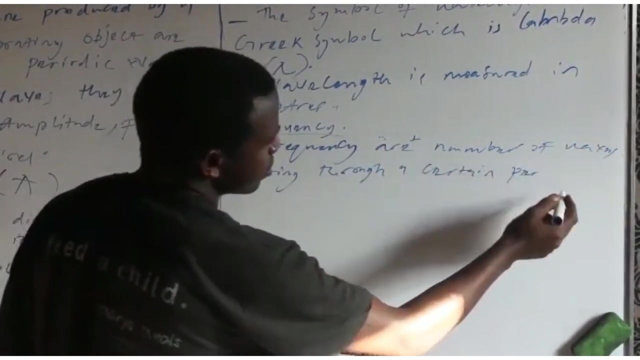 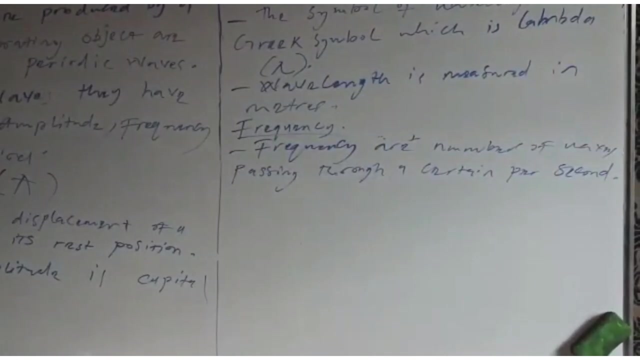 second, And the symbol of frequency is a calculator f, And frequency is measured in hertz, which is hz. So frequency, 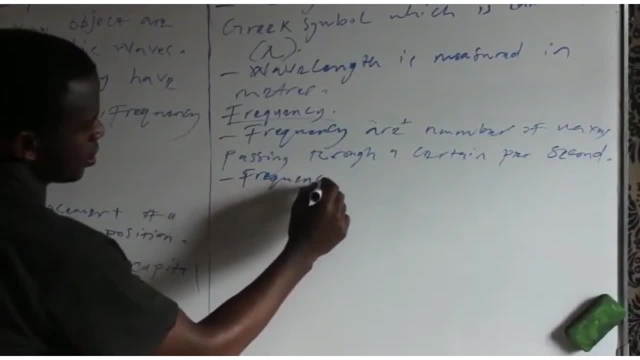 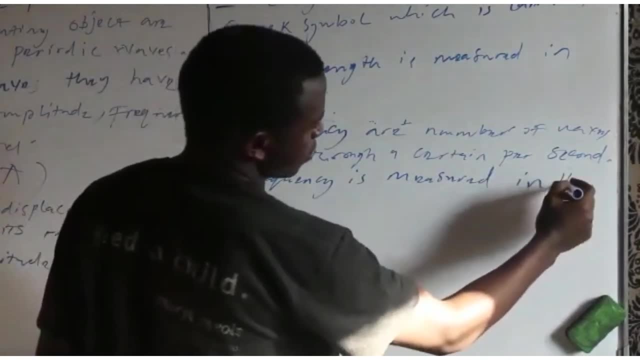 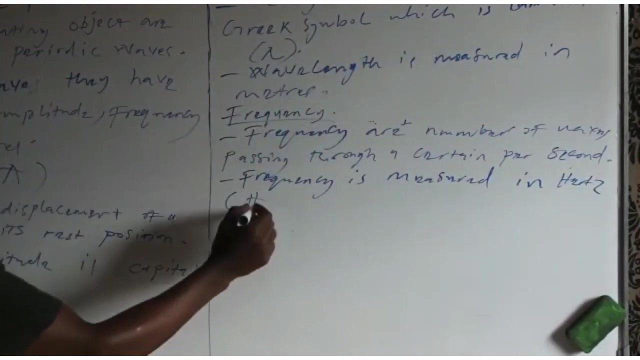 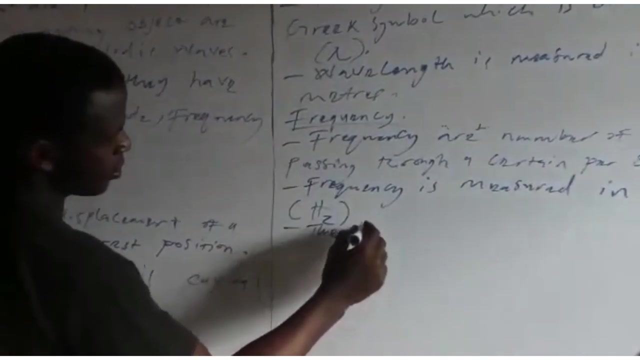 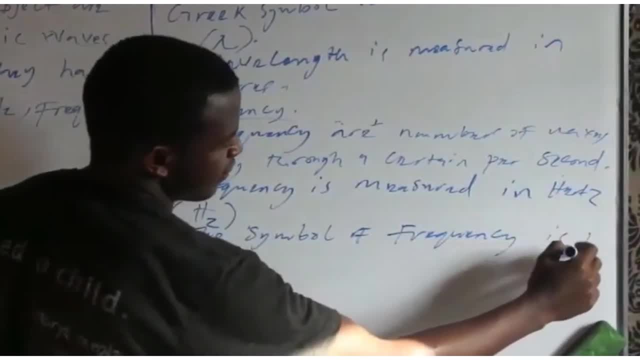 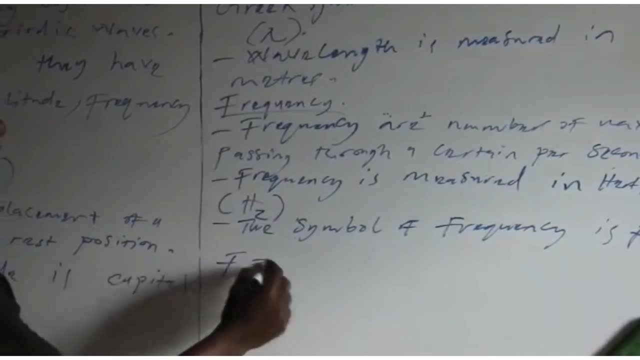 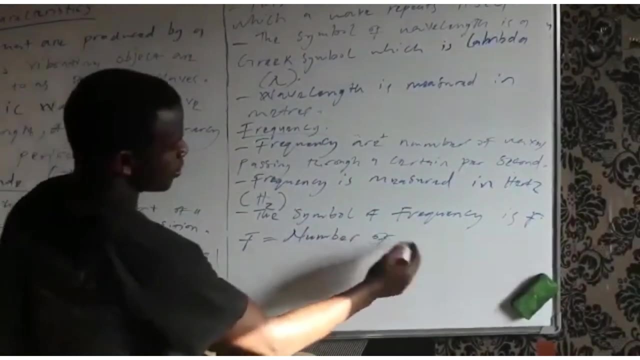 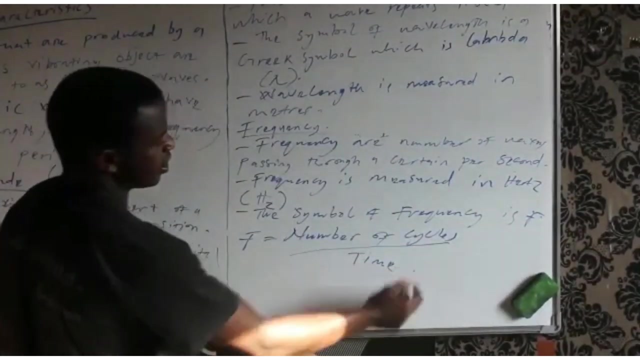 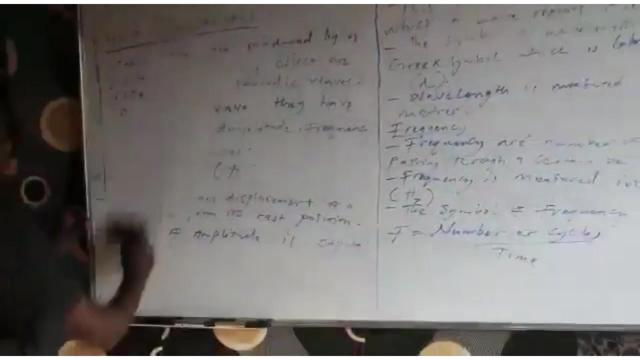 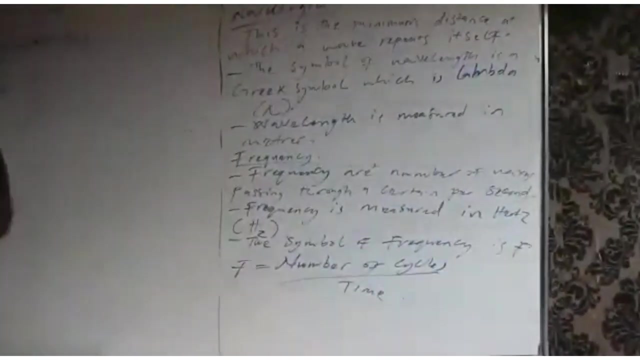 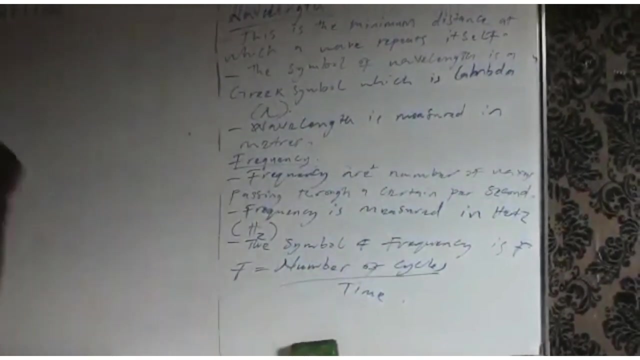 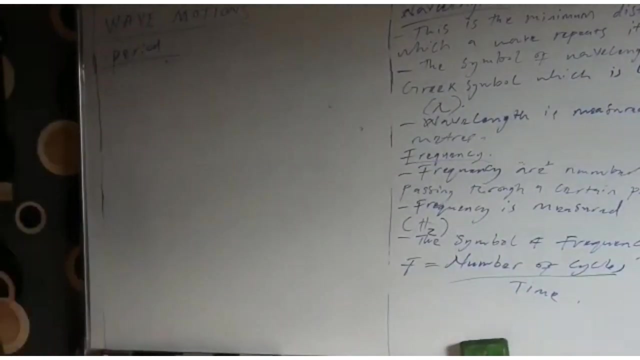 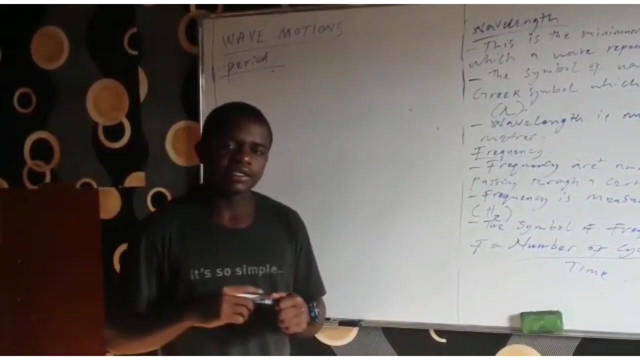 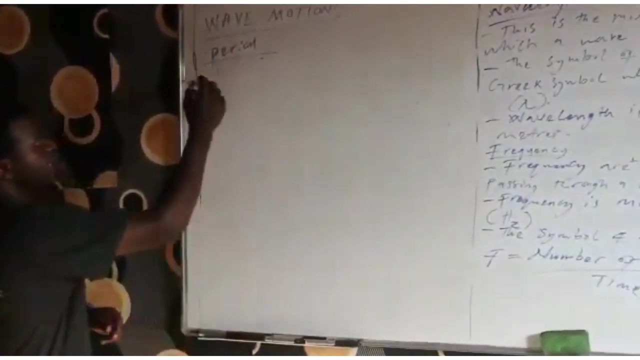 So period is defined as the time taken to produce one web, and period is measured in, And the symbol of period is capital letter T. So period is defined as this is time taken. 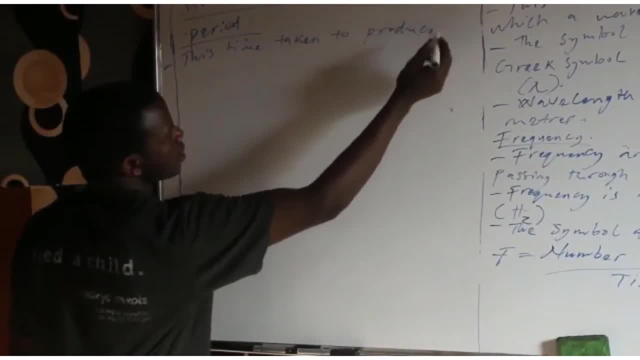 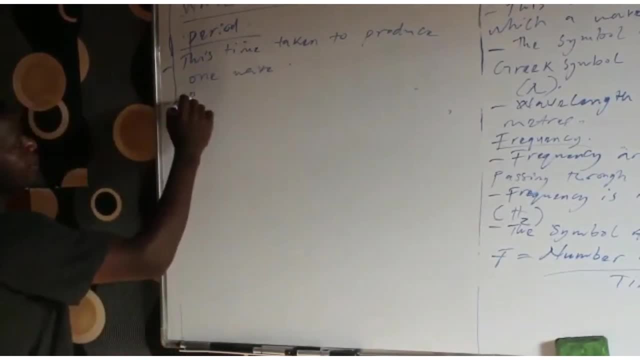 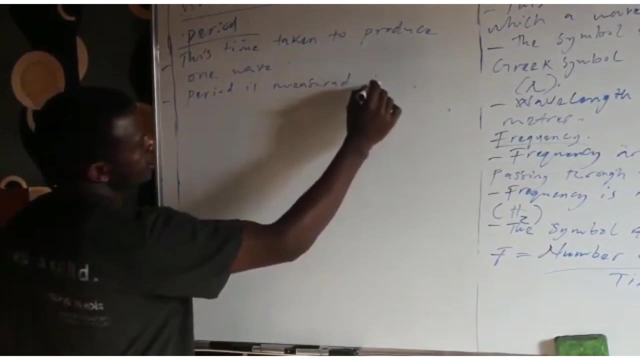 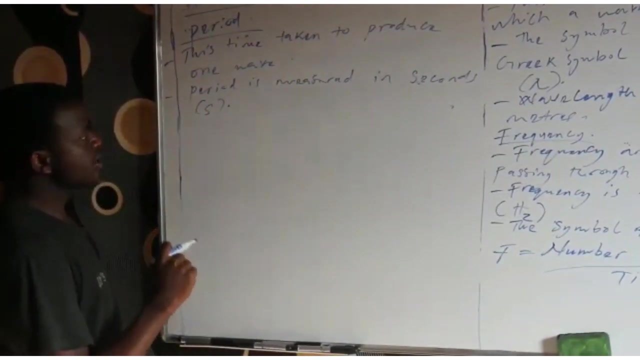 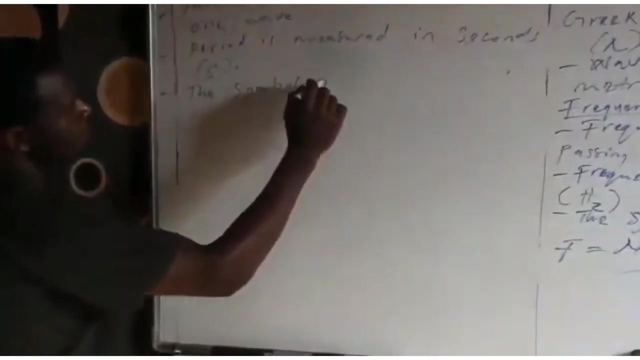 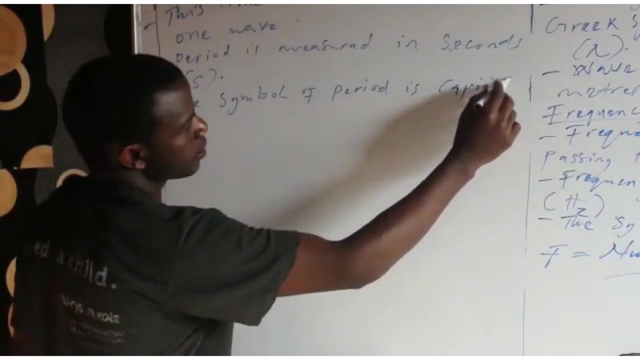 to produce one wave and period is measured in seconds. So period is measured in seconds And the symbol of period is capital letter T. The symbol of period is capital letter T. The symbol of period is capital letter T, So capital letter T. 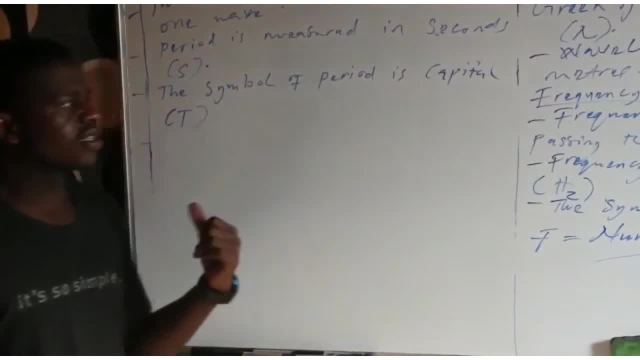 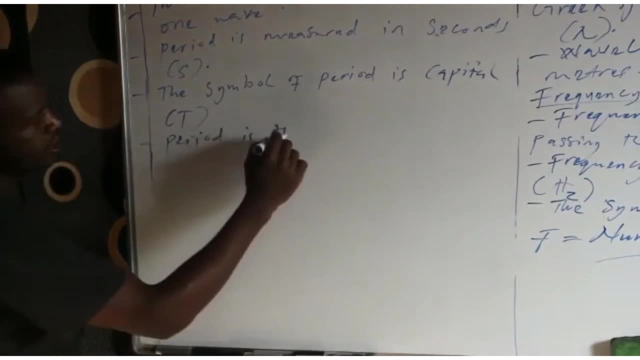 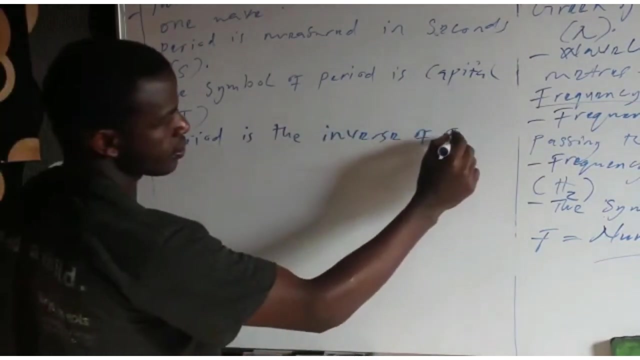 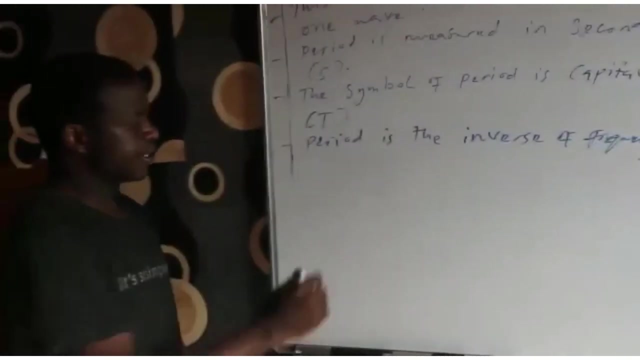 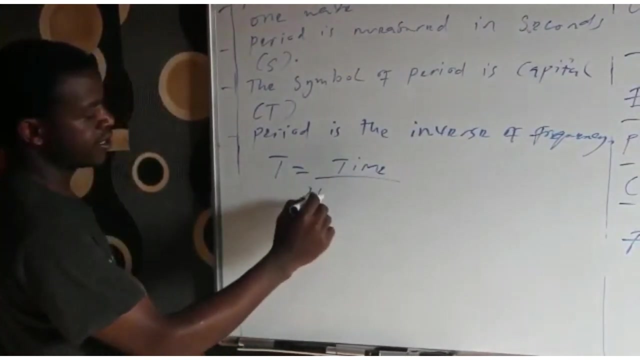 And you can also say: period is the inverse of frequency. So period is the inverse of frequency. So period is the inverse of frequency. So the formula that we use when calculating period- we say capital letter T is equal to time divided by number of cycles. 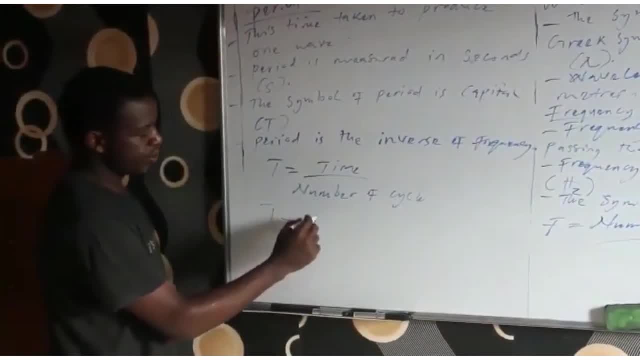 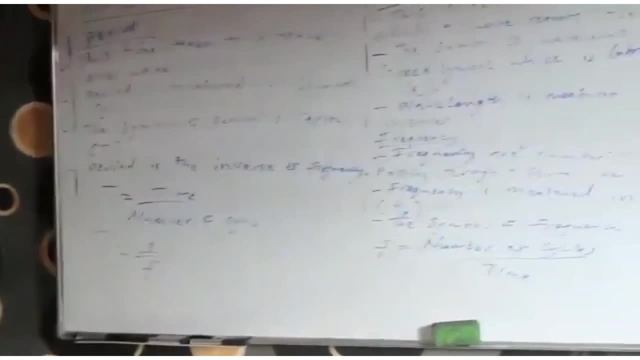 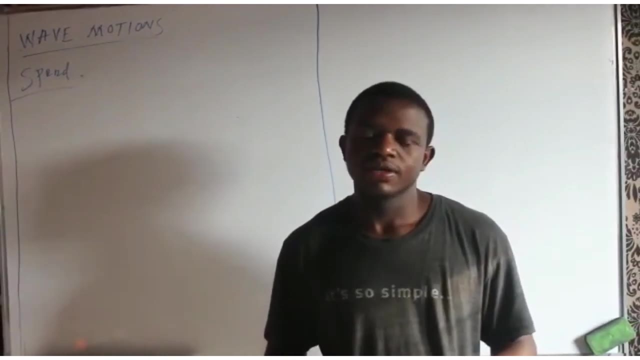 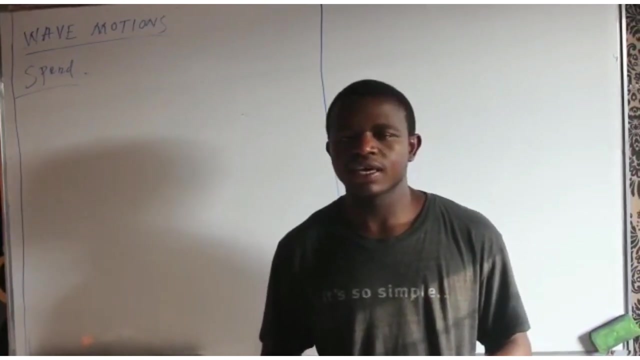 So we can also say: T is equal to 1 divided by F. So another way of characteristic that we are going to talk about is speed. So speed is defined as the distance travelled by a particle from its rest position per second. The distance travelled by a particle from its rest position per second. 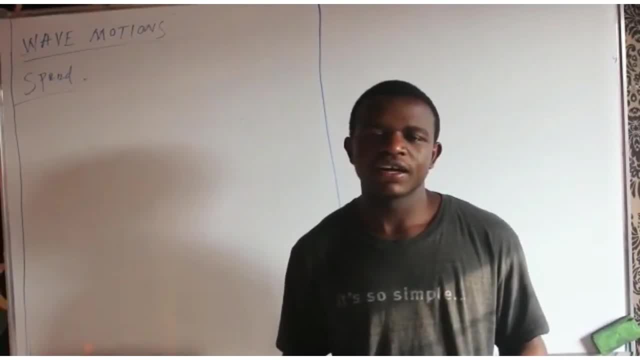 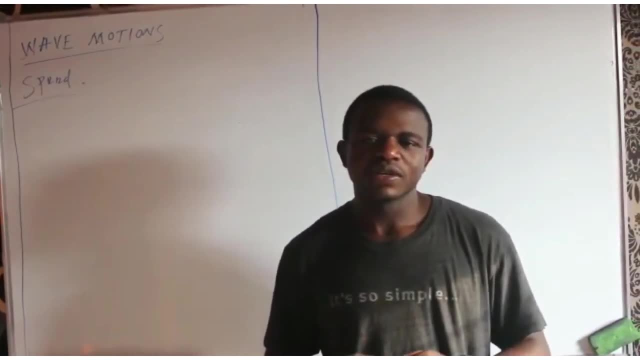 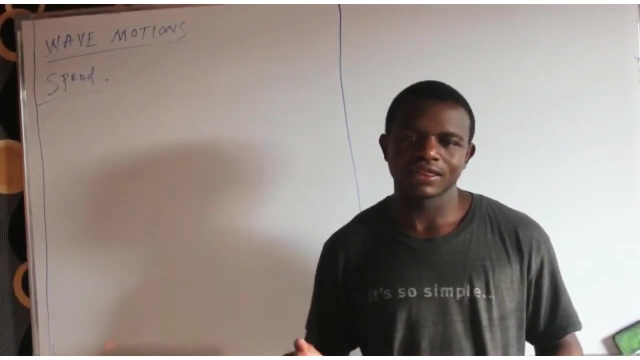 And the symbol that is used to represent speed is V, And speed is measured in meter per second, And the formula that is used when calculating speed is V equals to frequency multiplied by wavelength. So I am going to write these notes on the board. 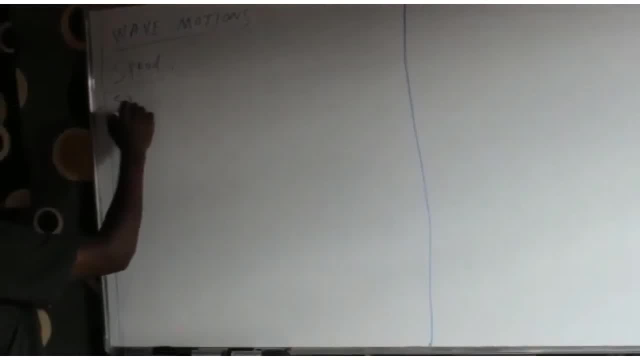 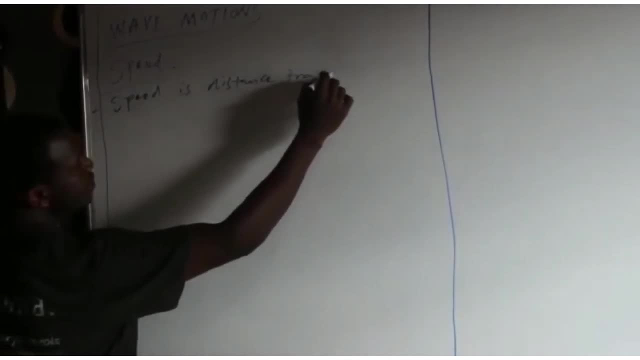 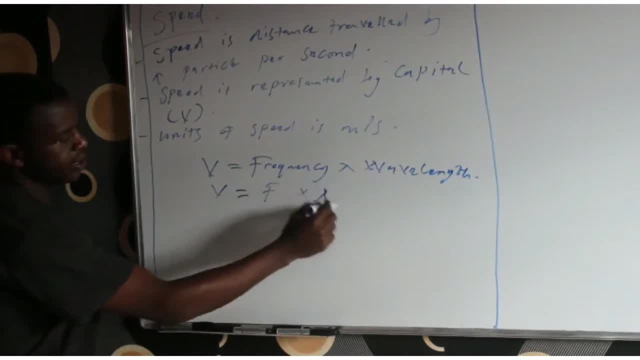 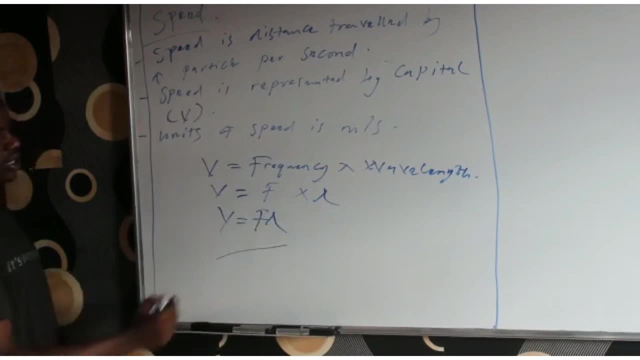 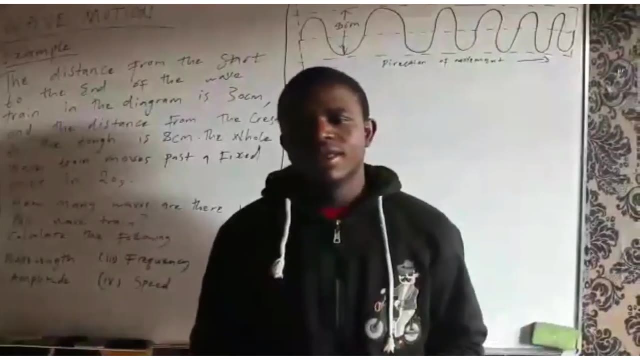 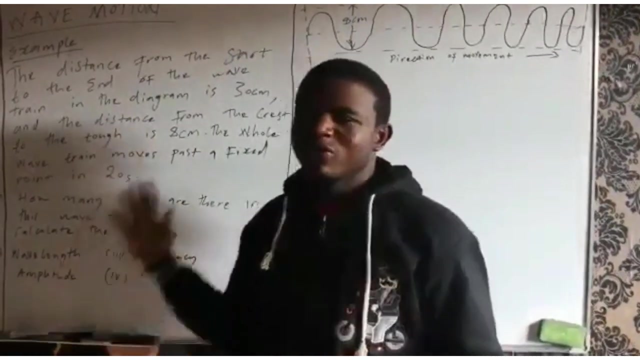 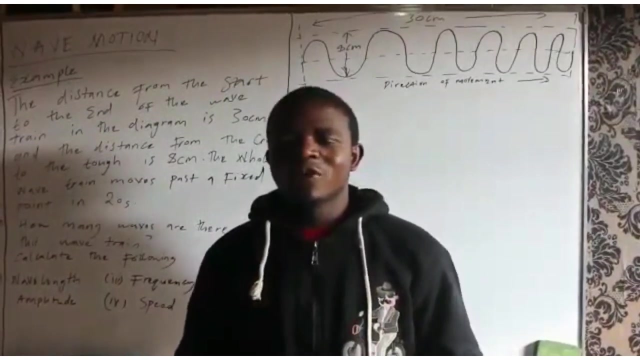 So speed is distance travelled by a particle from its rest position per second, And the symbol of wavelength is lambda. So you see, v is equal to f multiplied by lambda. So this is the formula that you use. So today, in wave motion, we're going to look at an example- So I've already written this example and we're going to go through this example. So we're going to calculate the wavelength, the speed, the frequency and the amplitude of this example. 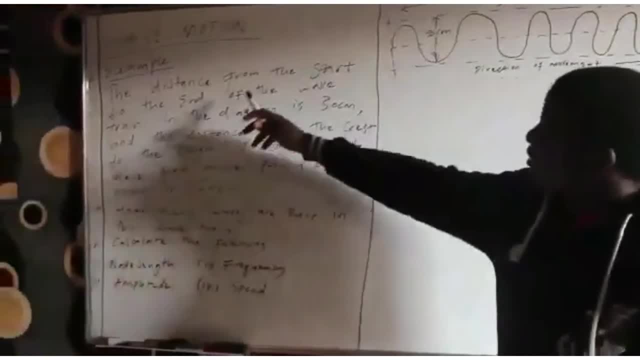 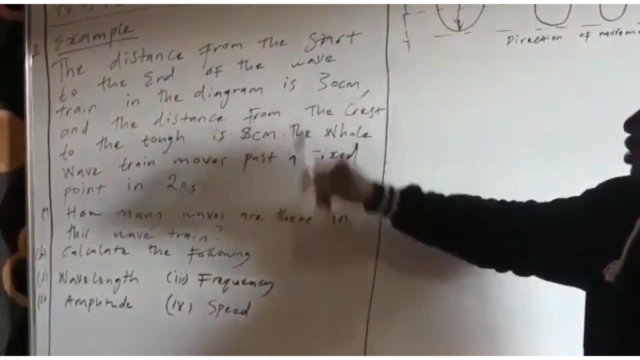 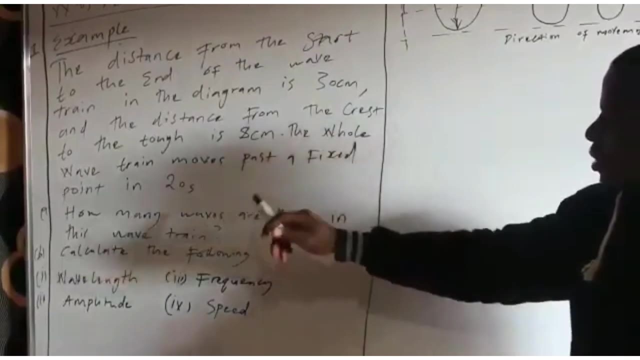 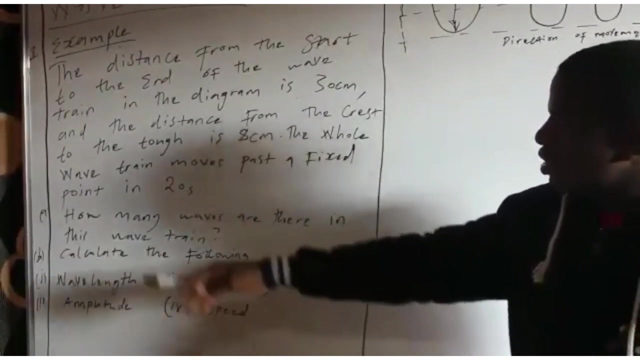 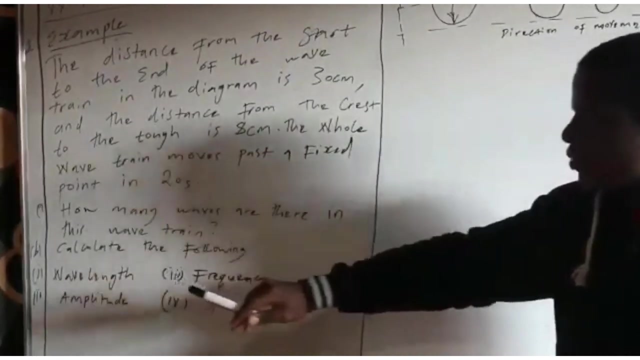 So the example reads: This diagram is 30 centimeters And the distance from the crust to the trough is 8 centimeters. The whole wave trend moves past a fixed point in 20 seconds. Then question A reads: How many waves are there in this wave trend? 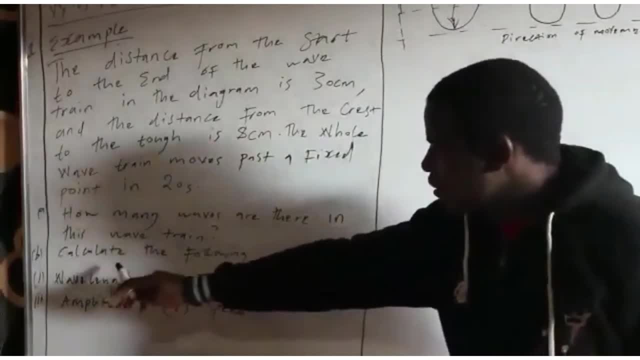 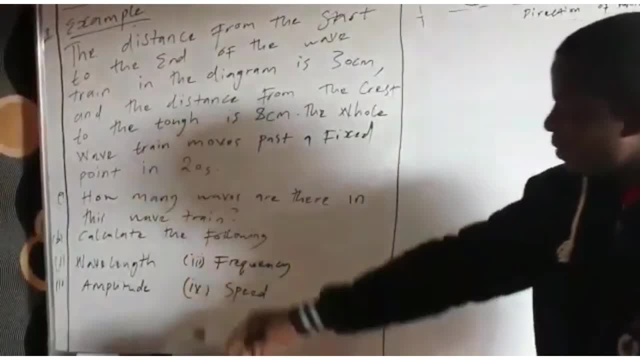 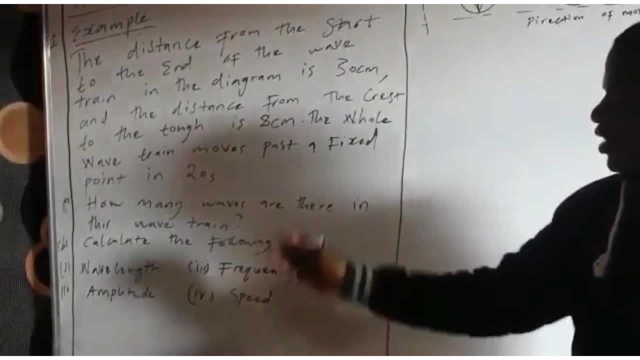 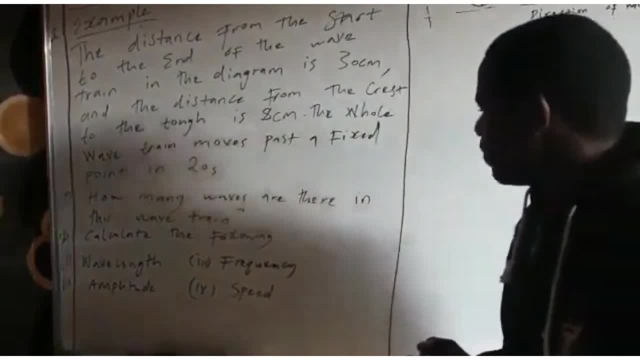 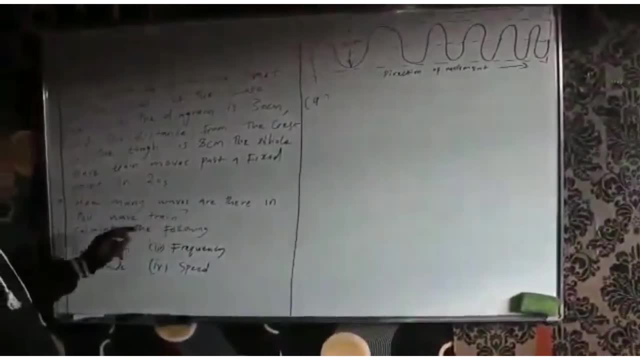 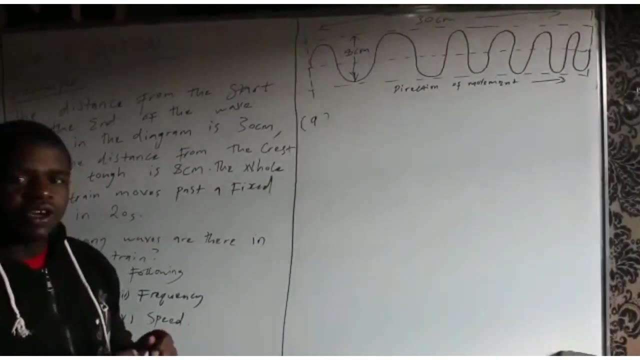 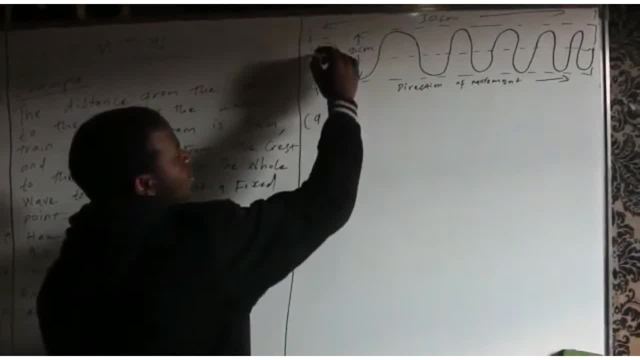 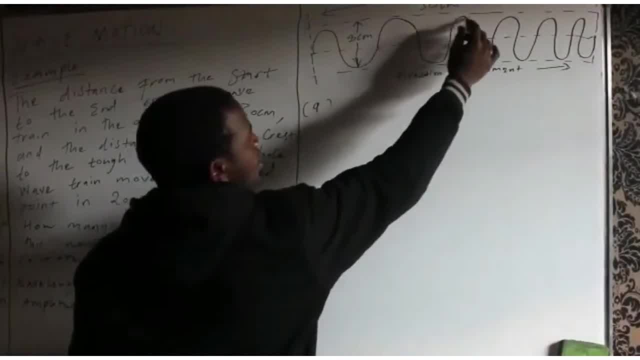 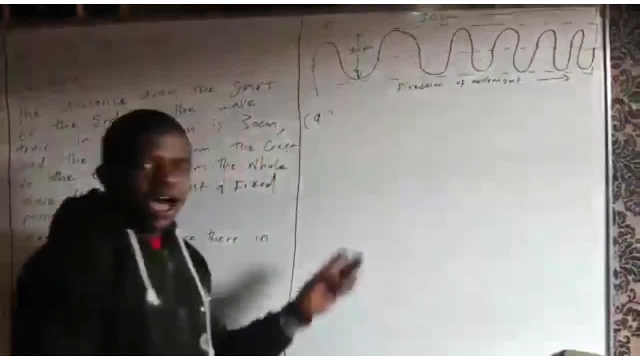 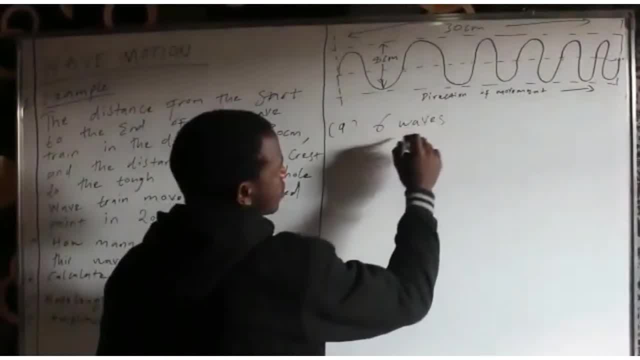 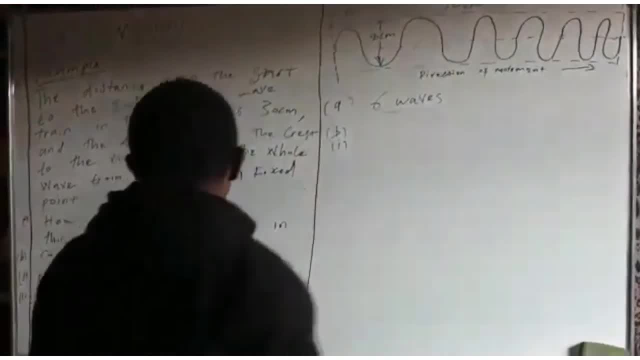 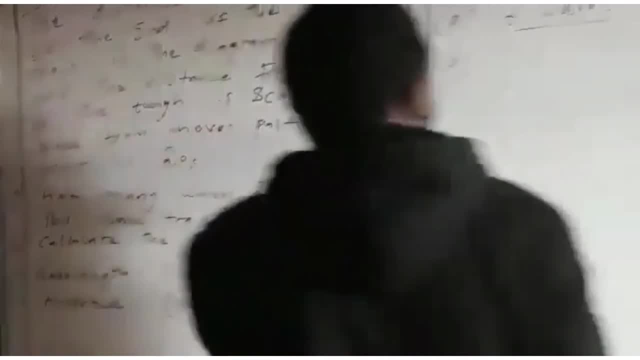 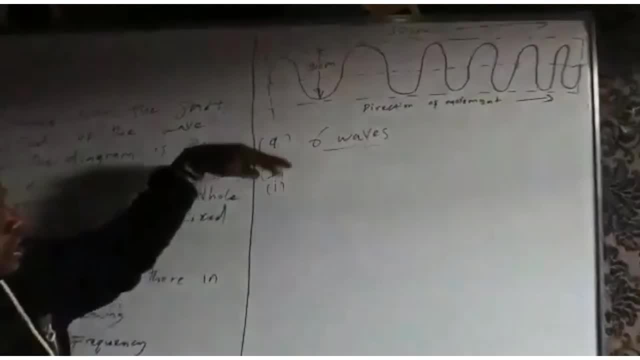 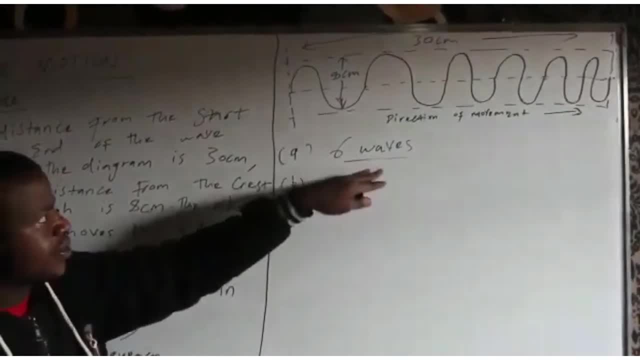 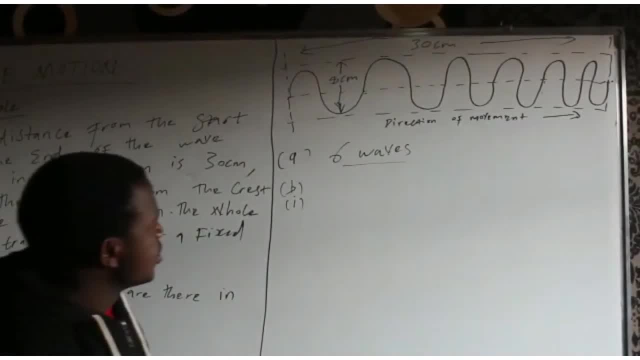 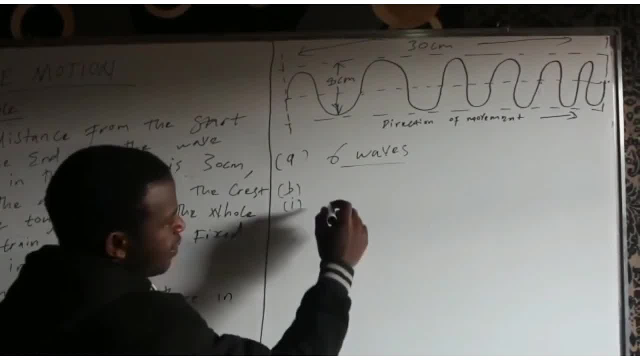 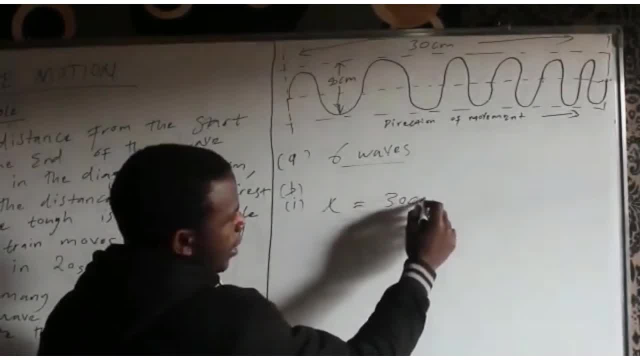 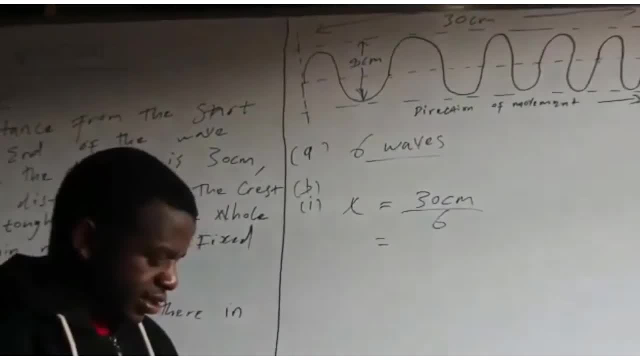 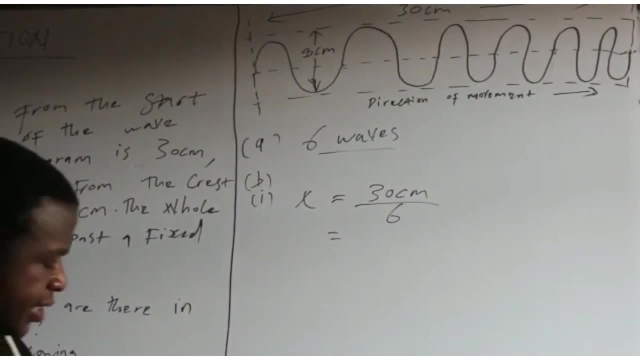 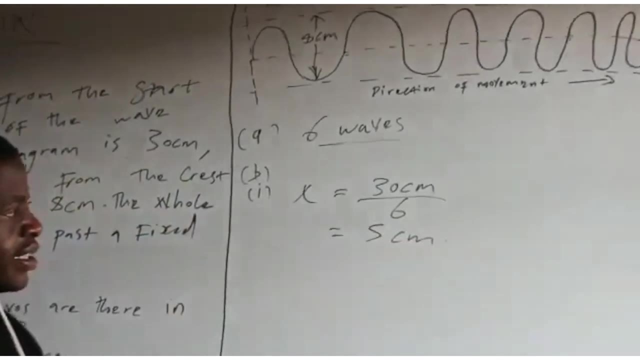 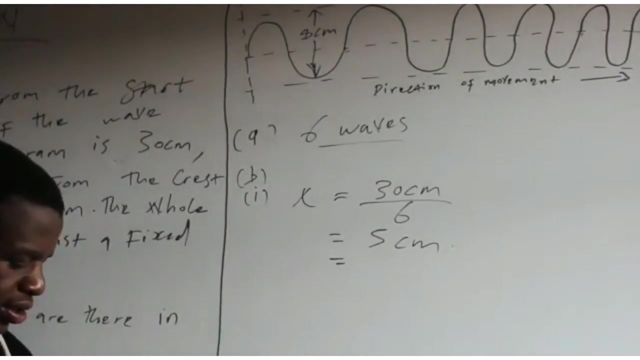 and this is giving me. so 30 divided by 6. 30 divided by 6 is giving me 5 segmenters. then, since the unit of wavelength is meters, I'm going to divide this 5 by 100, so I'll say 5 divided by 100. 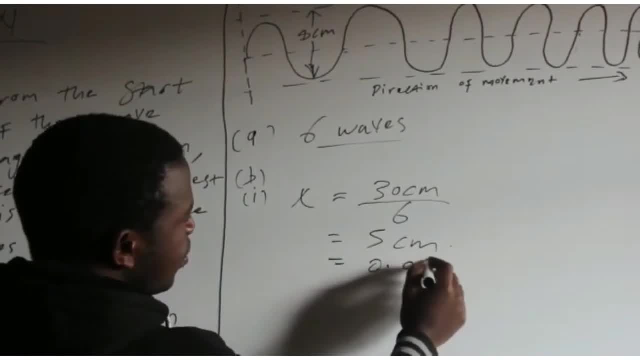 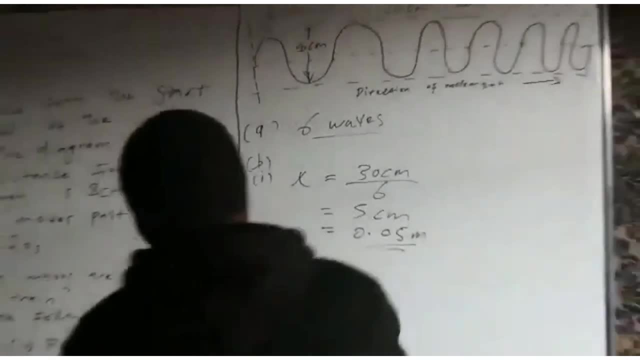 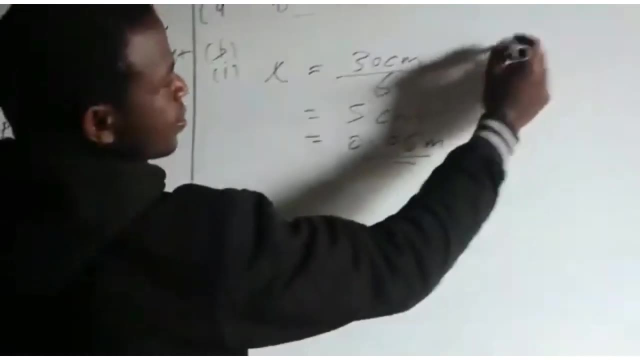 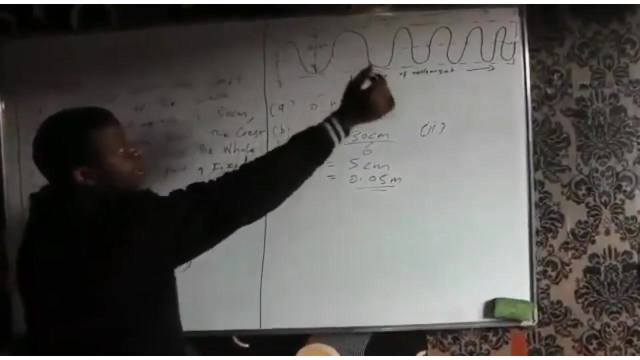 I'm having 0.05 meters, so this is the wavelength. let us proceed. let us look at Roman numeral 2, which is the amplitude. so, Roman numeral 2, I'm supposed to calculate the amplitude. so the amplitude is the distance from here to here. then I know that the distance from the trough to the crest 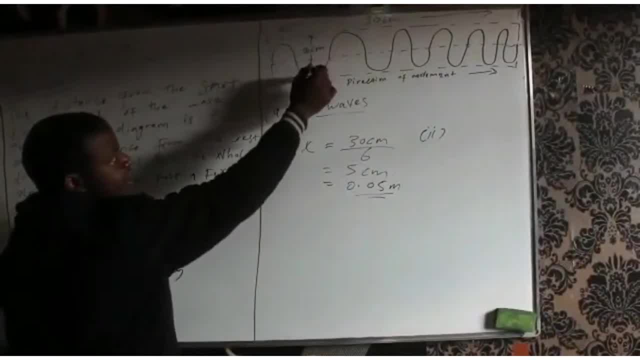 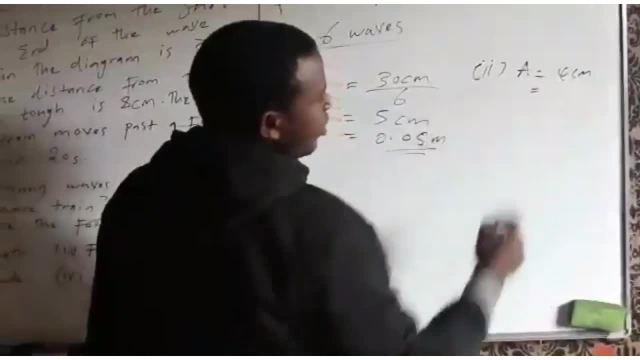 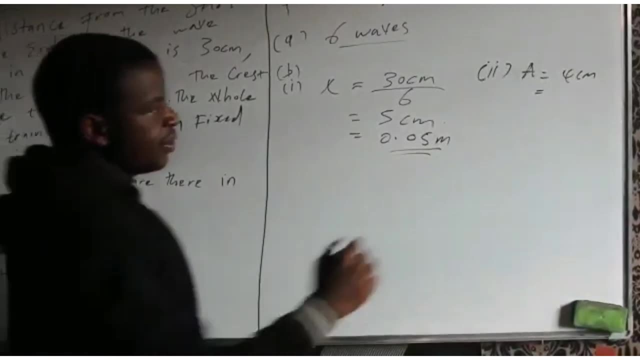 is 18 meters, so this means the distance from here to here. that's 4 segmenters. so amplitude is 4 segmenters and I know that amplitude is measured in meters. so I divide 4 by 100 and that's giving me 0.04. 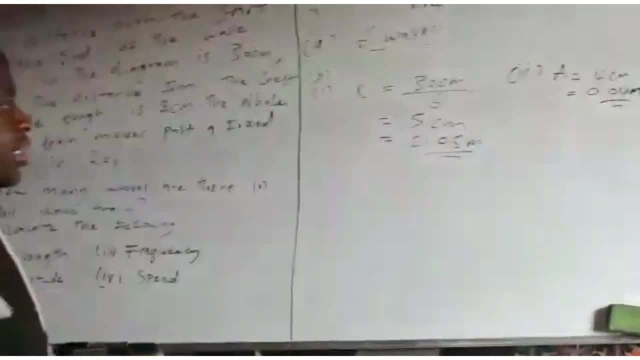 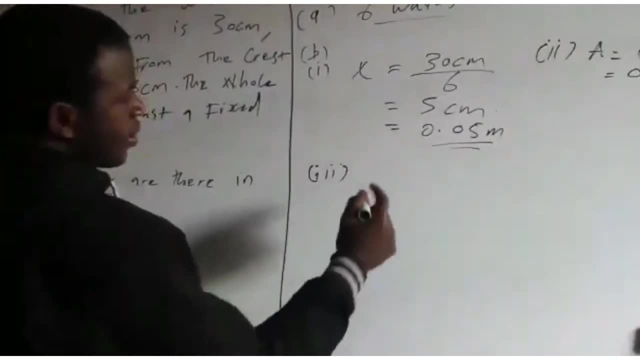 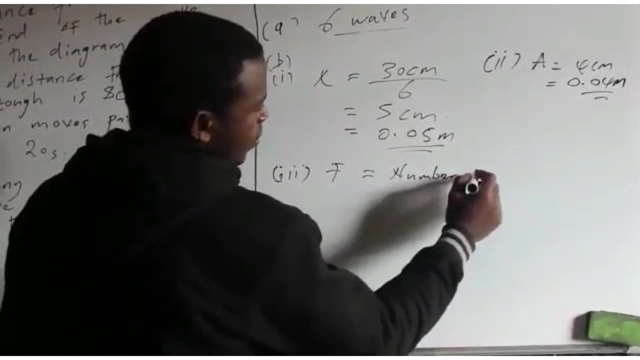 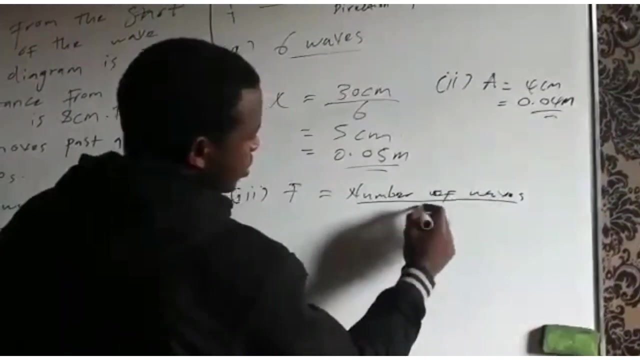 meters. then let us calculate the frequency. so this is Roman numeral 3. so frequency is 0.04 meters. so frequency is 0.04 meters is given by the formula: number of waves, number of waves over time. so my number of waves- I know that I have 6 waves- 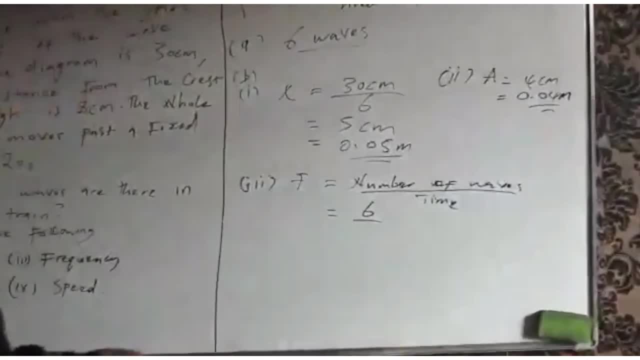 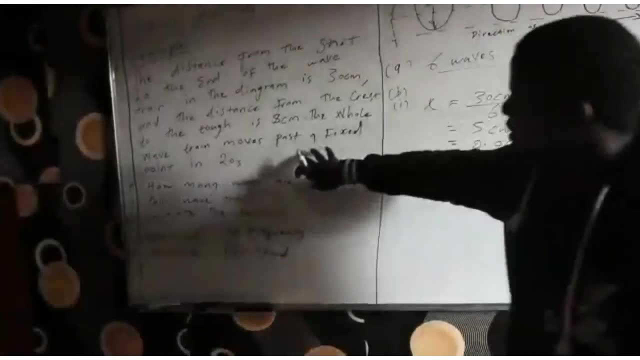 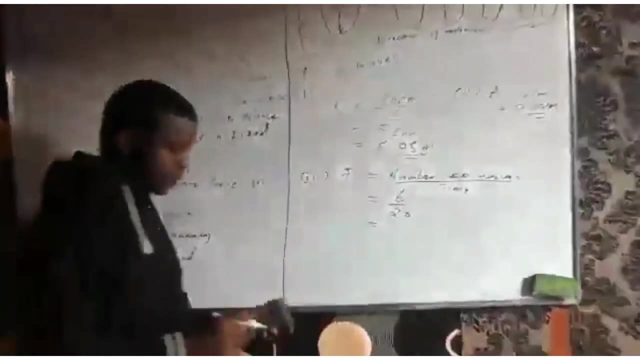 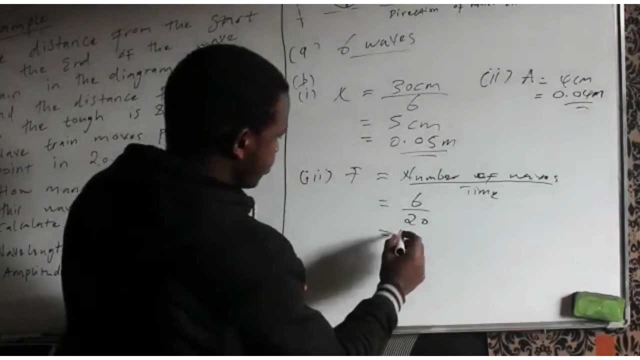 so 6 divided by the time, the time that the train takes. let us read the question. the whole wave train moves past the fixed point in 20 seconds. so it is 20 seconds, so 20. so 6 divided by 20 that's 0.3. 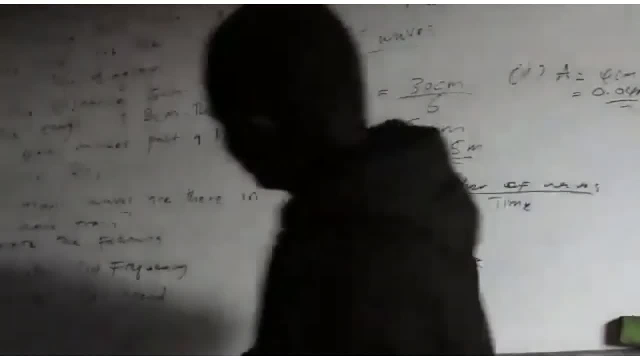 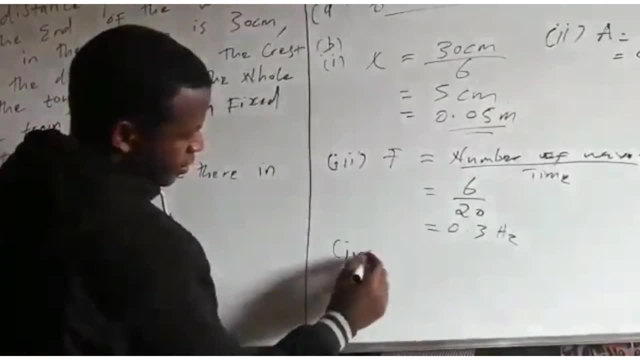 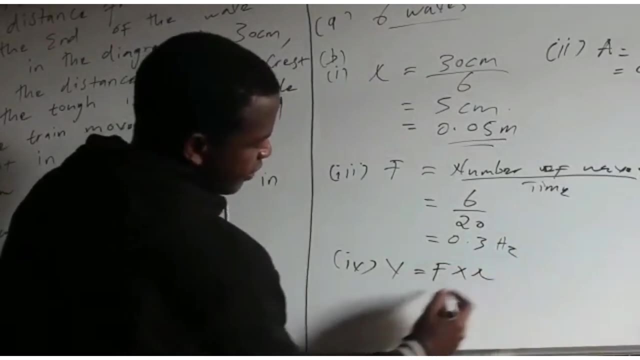 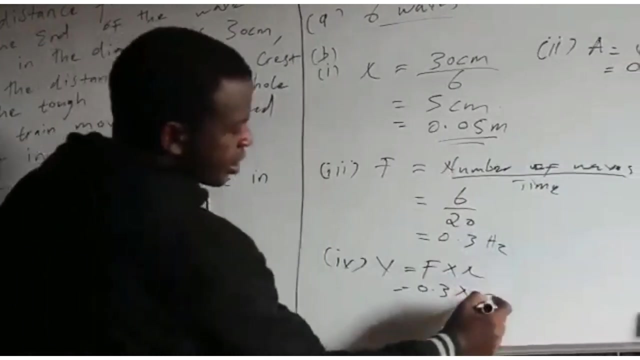 hertz? what about Roman numeral 3? I'm supposed to calculate speed. so I know that the formula of speed is: V is equal to frequency multiplied by wavelength, so my frequency is 0.3 multiplied by the wavelength is 0.05, so my speed is equal to. 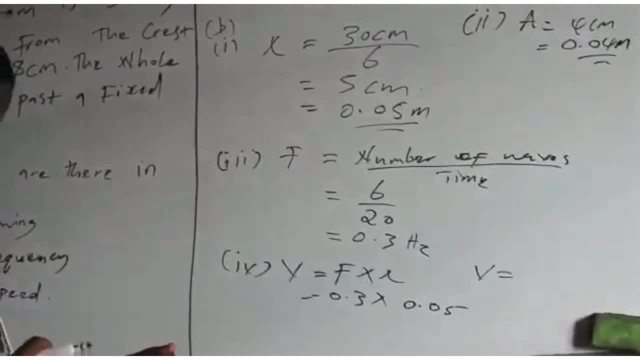 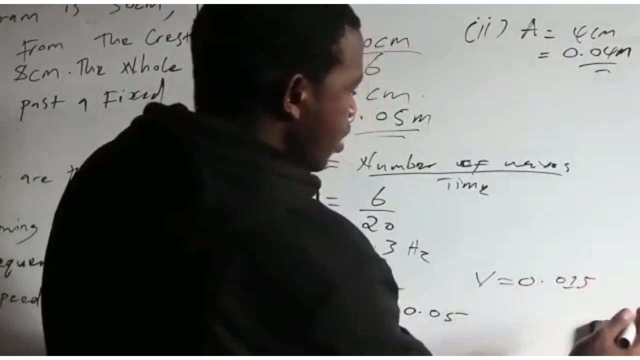 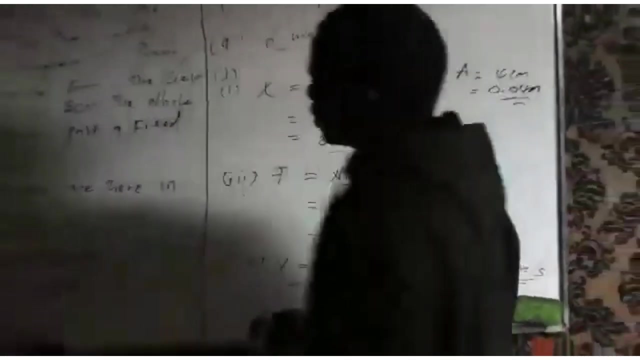 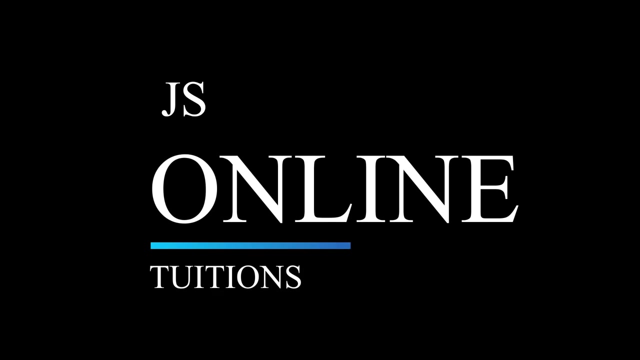 0.3 multiplied by 0.05, it's a 0.05, it's a 0.015 meter per second. so this is how you can calculate this question. JS online tuitions are available each and every month and we provide the following subjects: 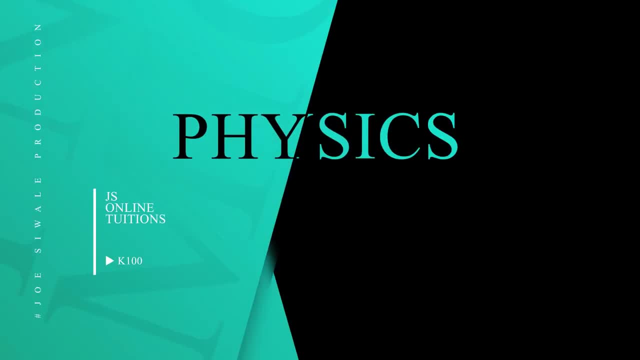 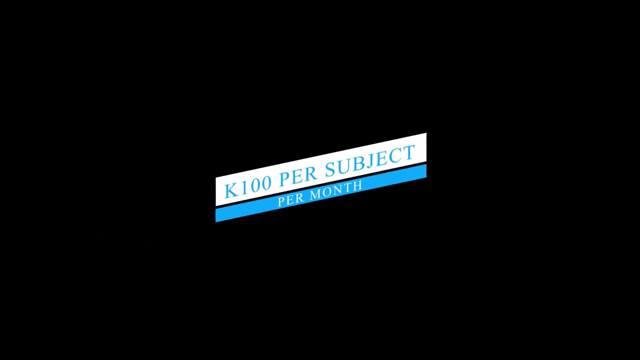 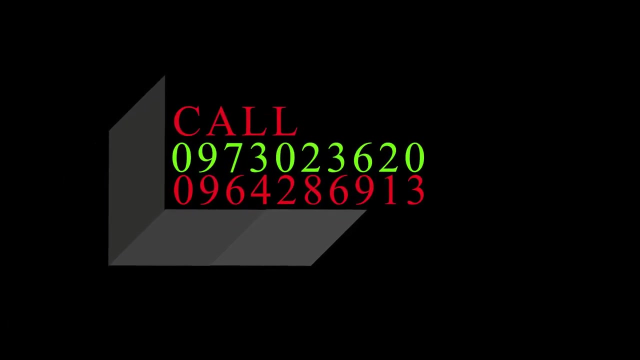 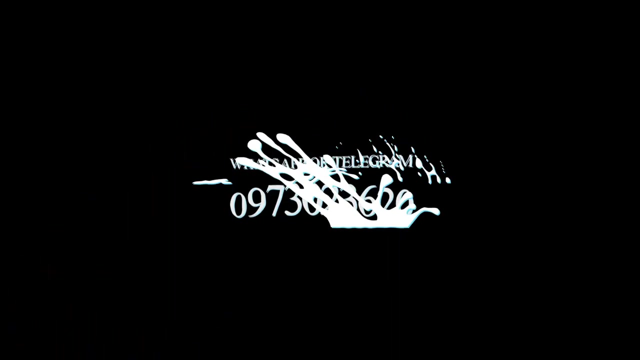 mathematics, biology, physics, chemistry and accounts. the price is only 100 kwacha per subject and that's per month. for further information, you can call me on these numbers, 0973023620 or 0964286913, or you can text me on whatsapp or on telegram on. 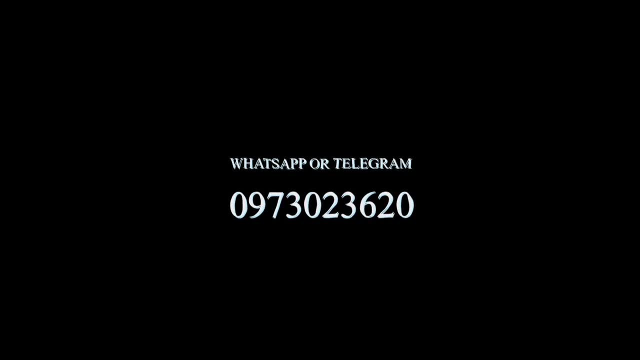 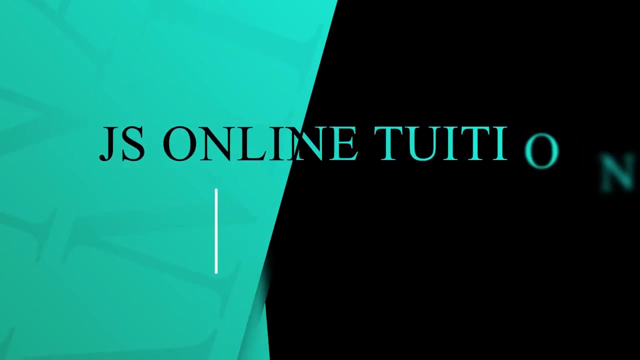 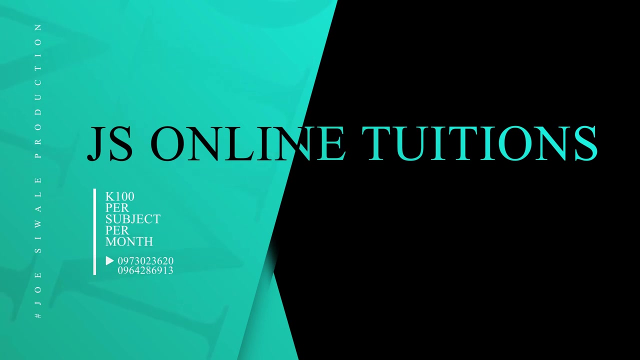 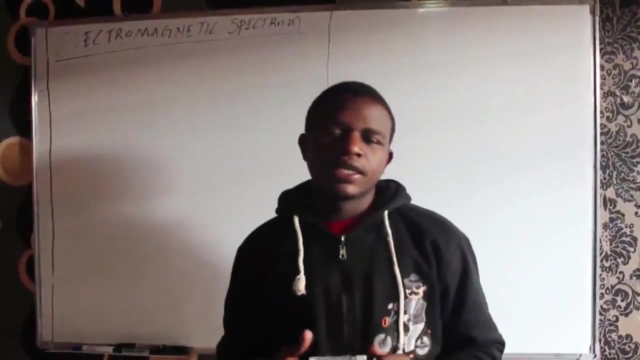 0973023620. join the online tuitions today and have a real life change with your education. I'll be hoping to see you soon, God bless. So the next thing that we're going to talk about is the electromagnetic spectrum. so the electromagnetic spectrum consists of: 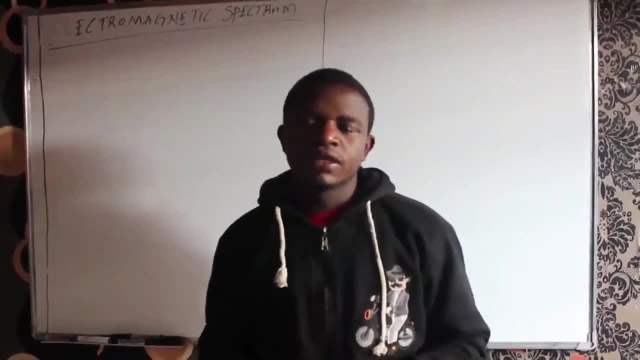 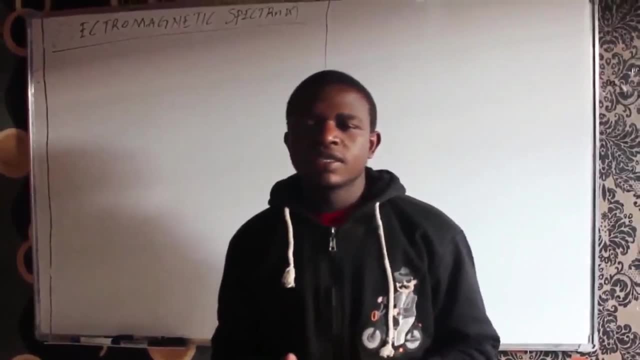 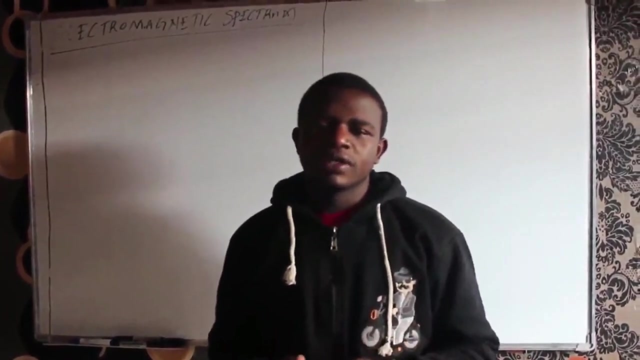 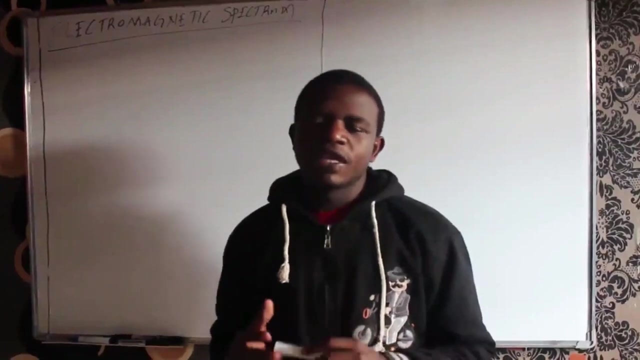 waves that are different wave types, different wavelengths. So this starts from the radio waves to the gamma rays, And some of the electromagnetic waves that we use in our daily lives include the radio waves, the microwaves and the infrared, Then the X-rays and the gamma rays. they also form part of. 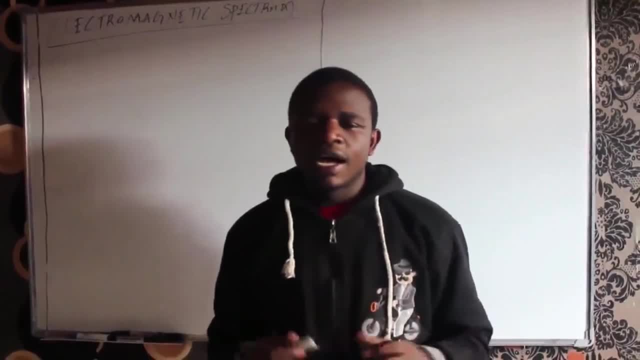 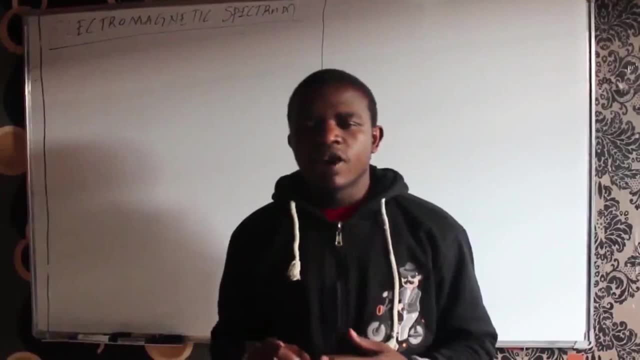 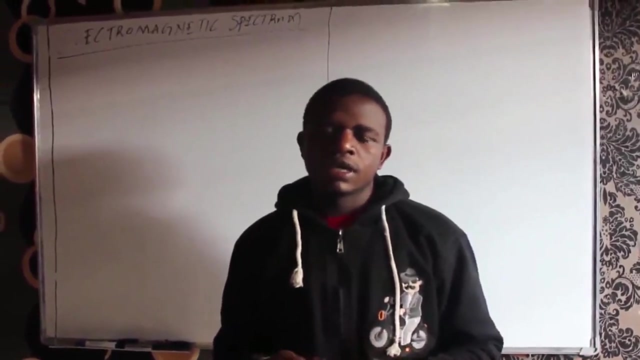 the electromagnetic spectrum And how the sequence is arranged. we have the radio waves, the microwaves, the infrared radiation, the visible light, the ultraviolet waves, we have the X-rays and we also have the gamma rays. So let me just write these points down. So 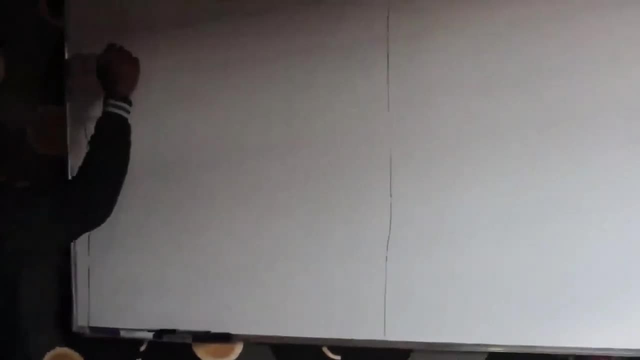 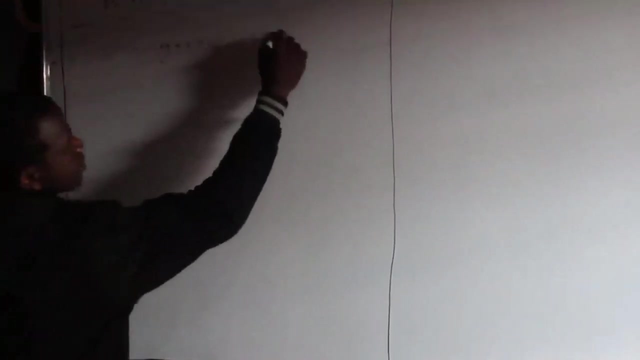 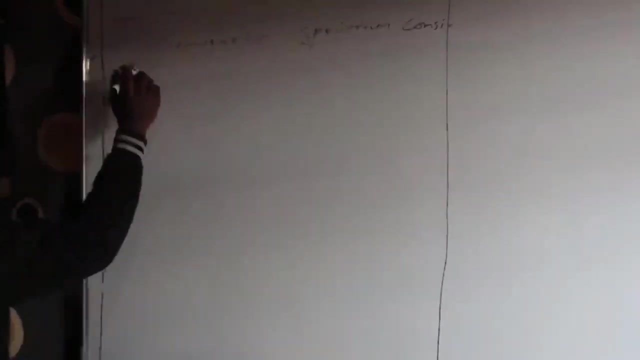 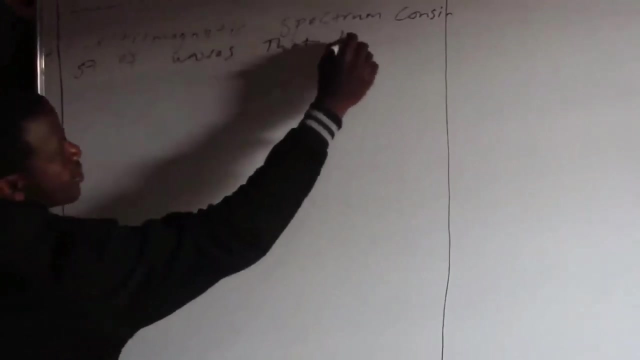 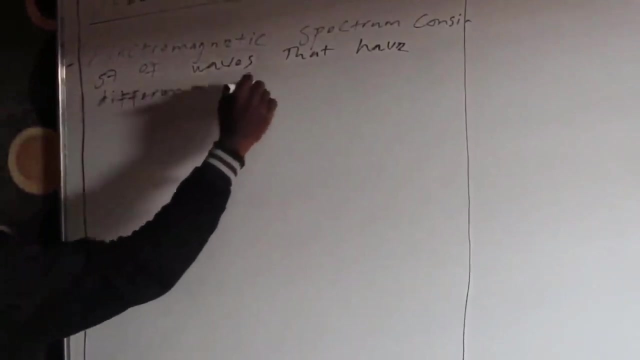 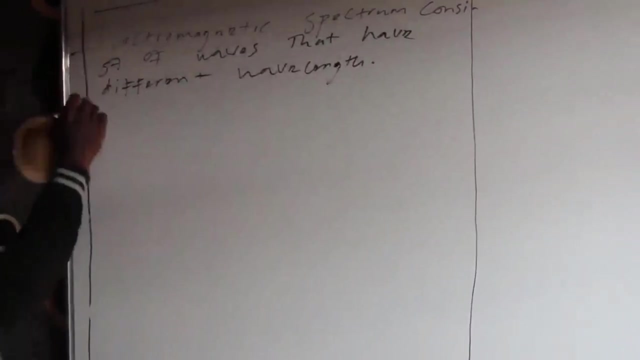 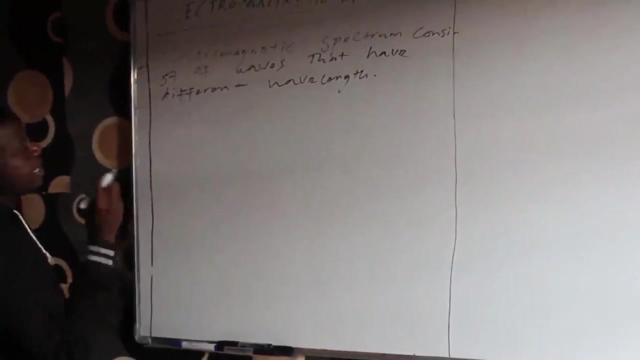 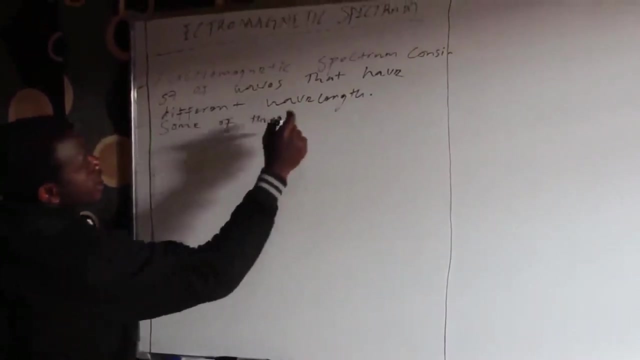 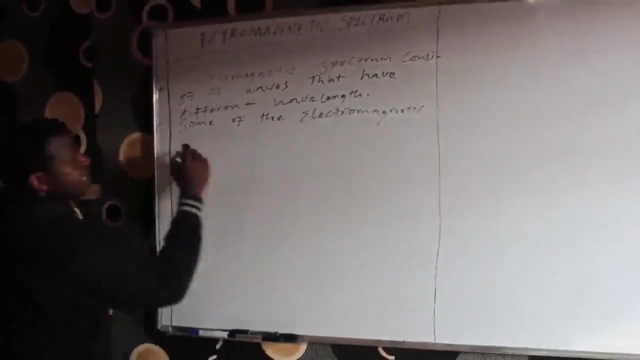 I've seen the electromagnetic. The electromagnetic spectrum consists of waves that have different wavelengths. Then some of the electromagnetic waves that we use in our daily lives include the radio waves, the microwaves and the infrared. So some of the electromagnetic waves that we 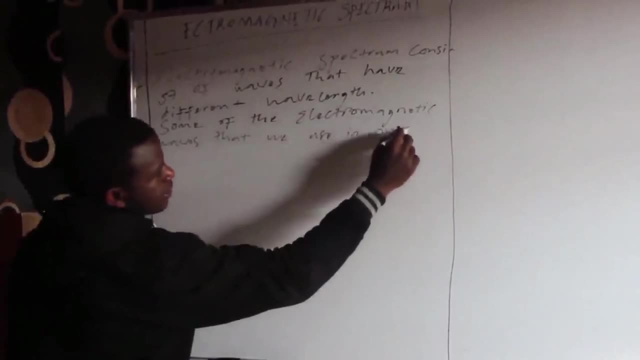 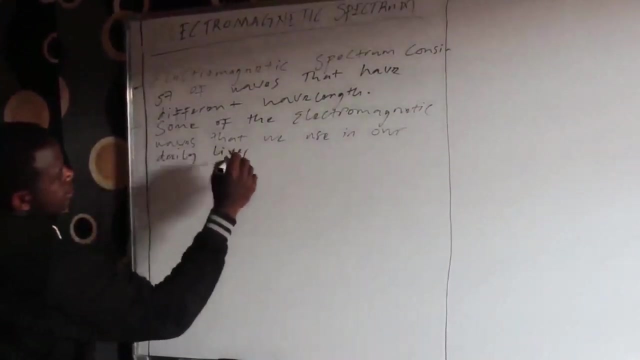 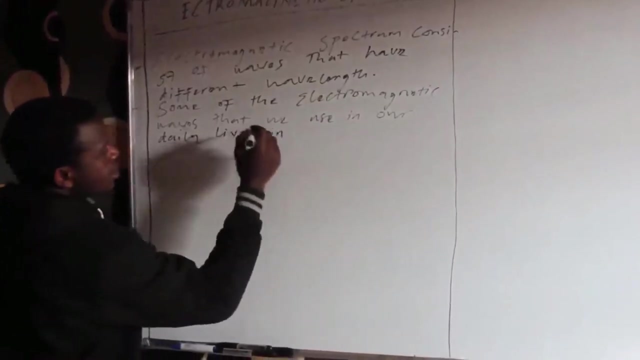 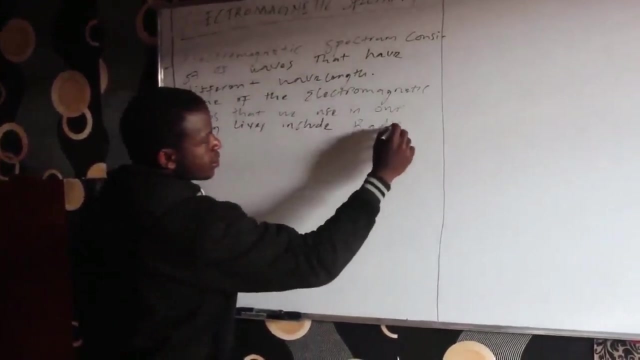 use. So some of the electromagnetic waves that we use in our daily lives, In our daily lives include In our daily lives, include Include the radio waves, the microwaves and the infrared. So the electromagnetic spectrum consists of the radio waves, the microwaves and the infrared. 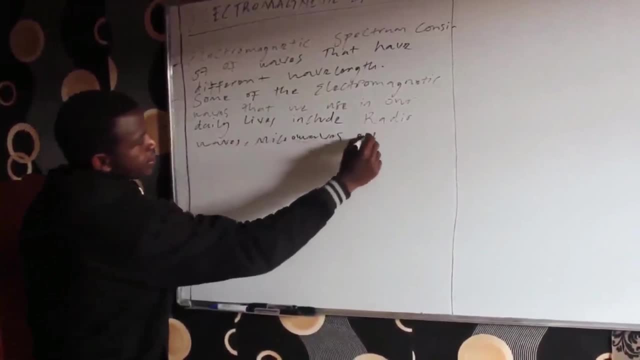 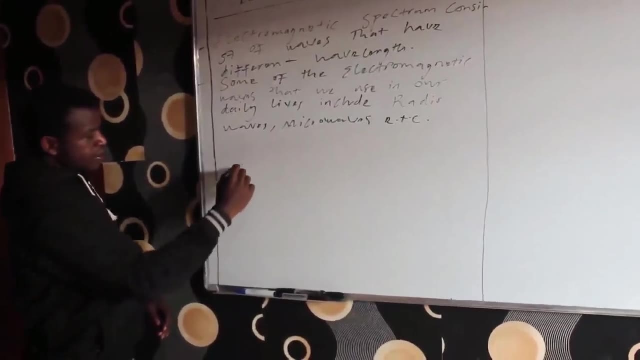 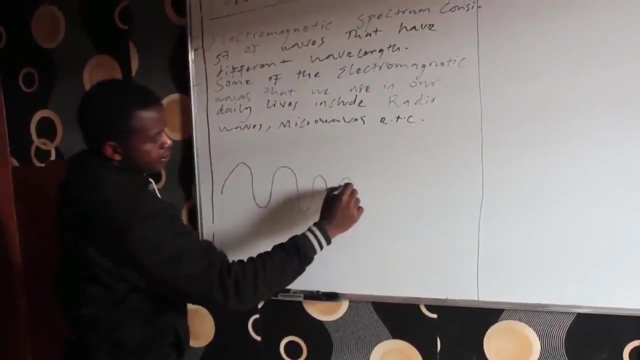 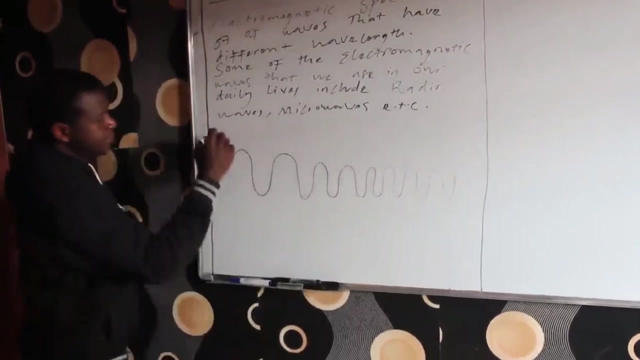 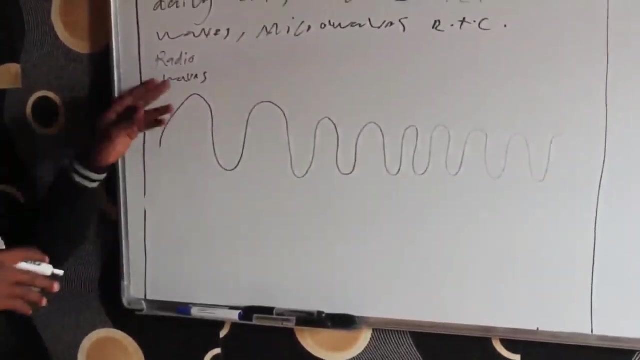 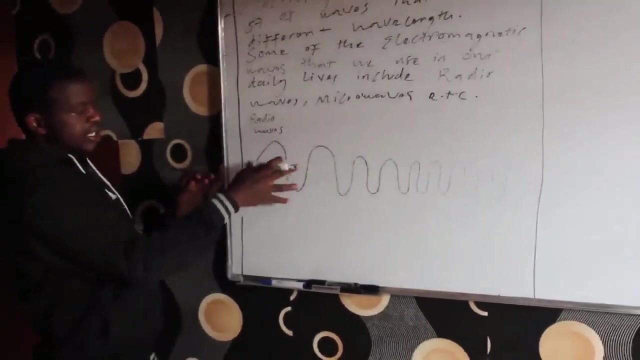 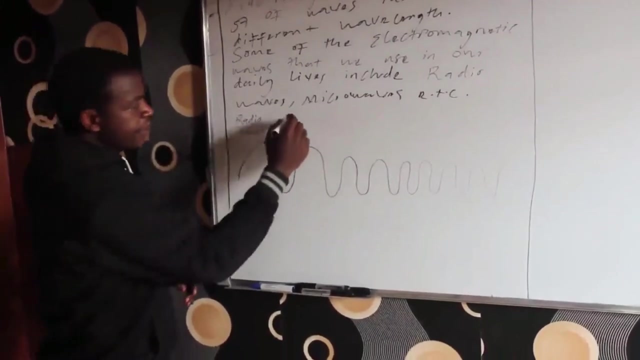 and etc. then the sequencing. so this is how the sequence is. so, as I'll draw, these are representing the wavelength. so the radio waves they have, their wavelength is large, as you can see, their wavelength is large. then, coming after the radio waves, we have the microwaves. 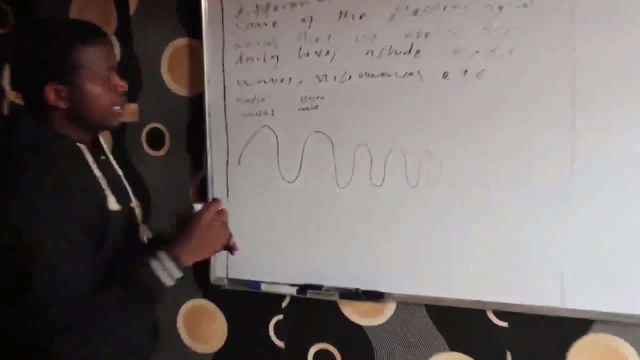 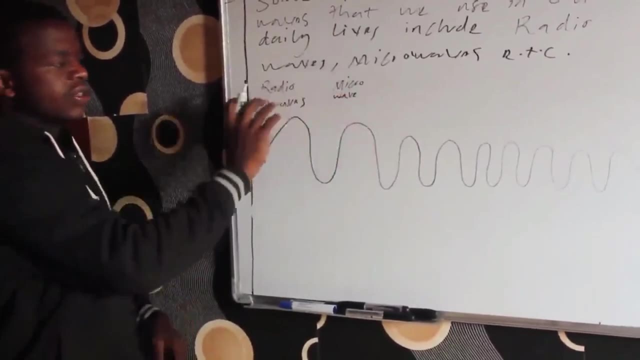 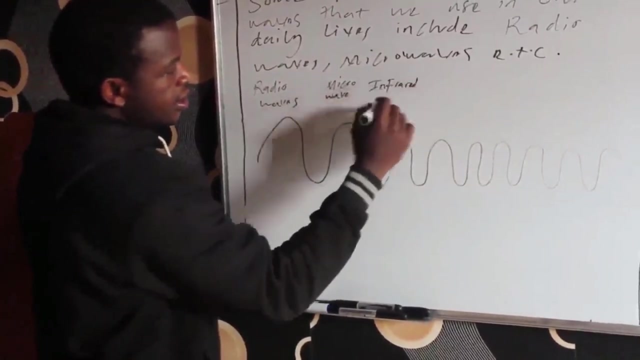 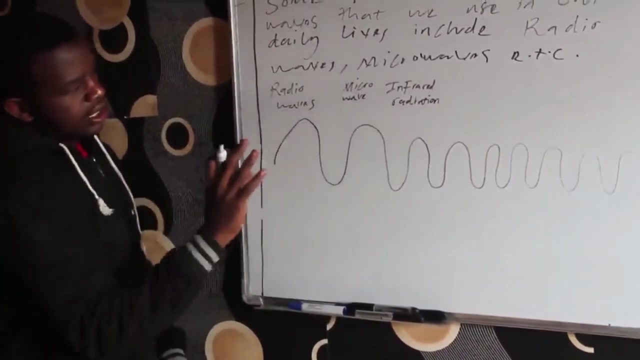 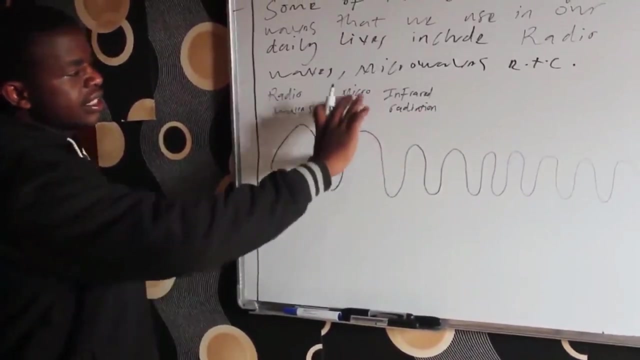 the microwaves, then the wavelength of the microwaves is also large, but it's not larger than those of the radio waves. then we have the infrared radiation, so also these, they have a large size of the wavelength, but their wavelength is less than that of the microwaves and the radio waves. then 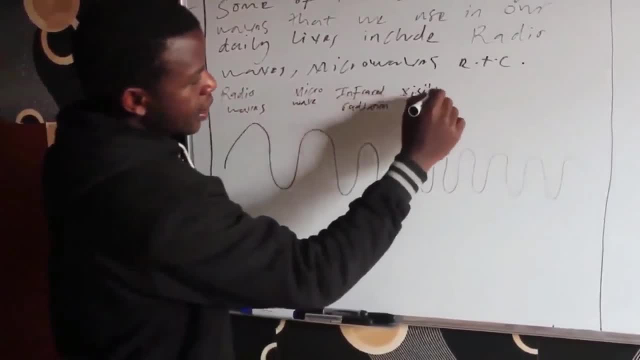 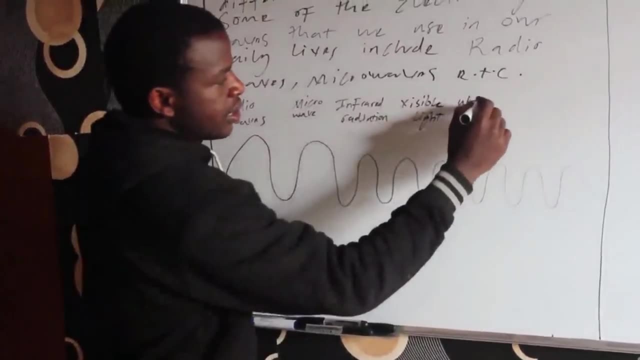 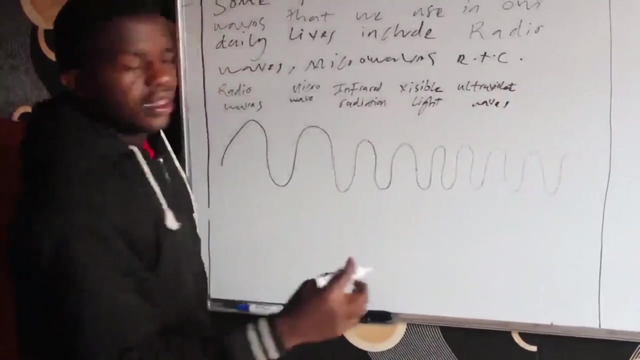 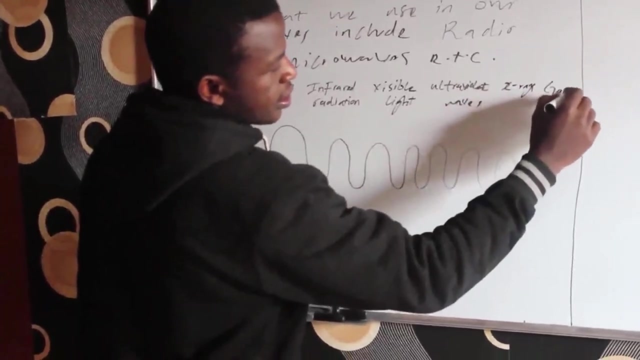 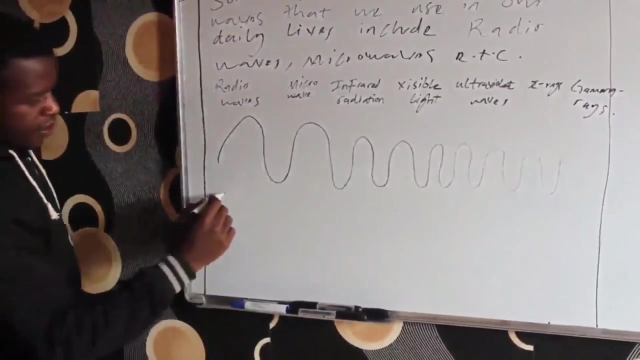 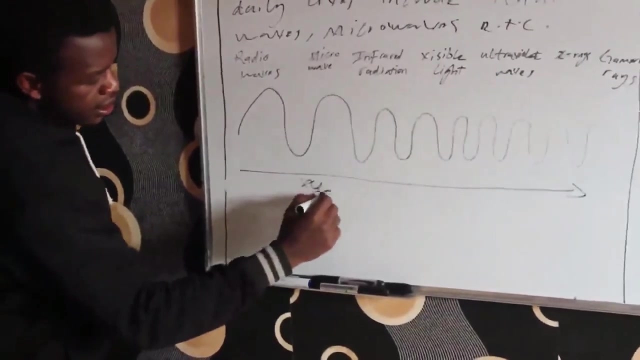 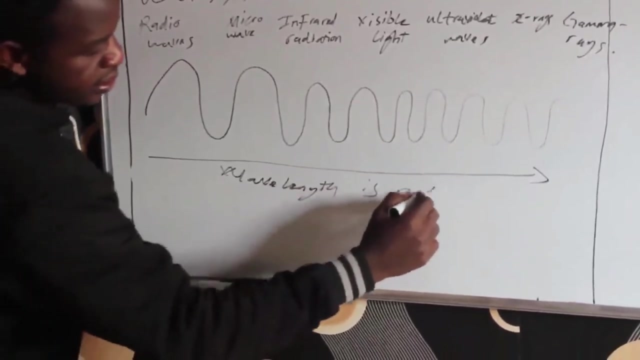 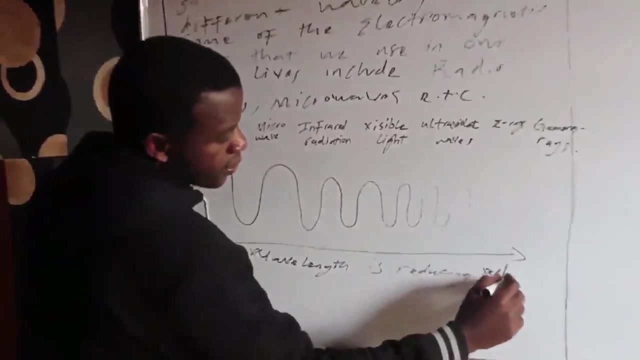 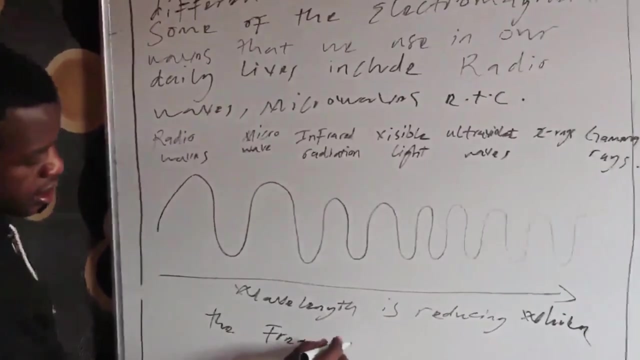 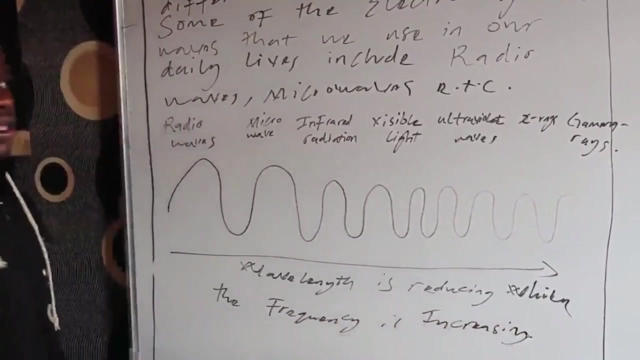 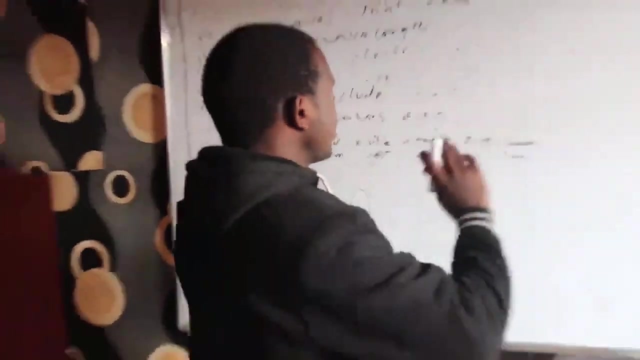 we also have a visible light. visible light, we have ultraviolet, ultraviolet waves, then we have the X-rays and the gamma rays. so, moving from from left to the right side, here the wavelength, the wavelength is reducing while the frequency is increasing. so one, the frequency is increasing. then let us now look at the length of the wavelength, so the 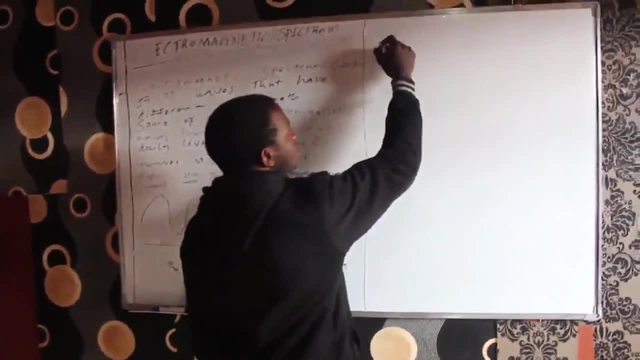 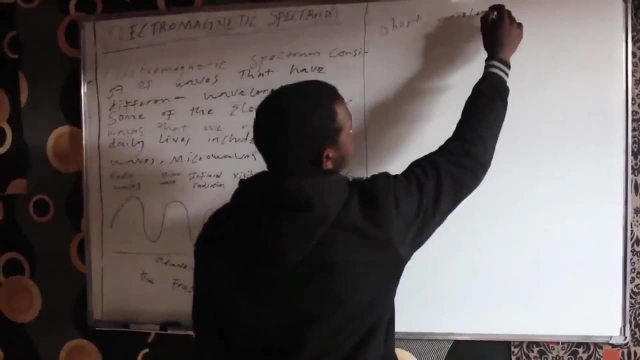 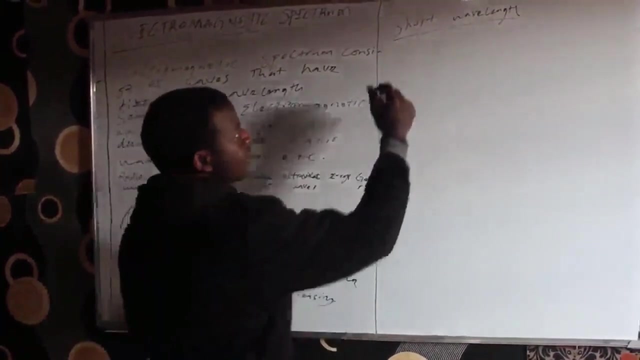 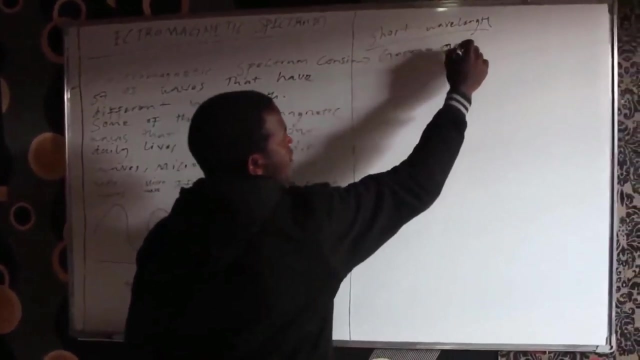 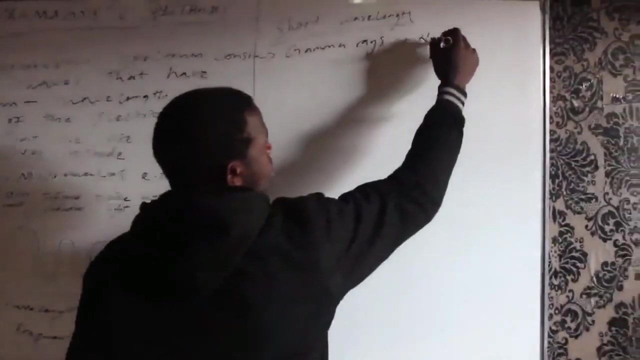 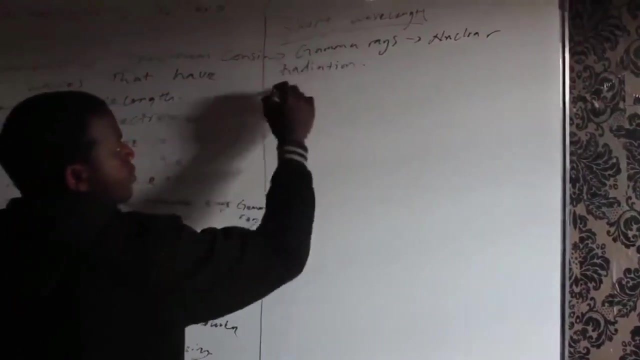 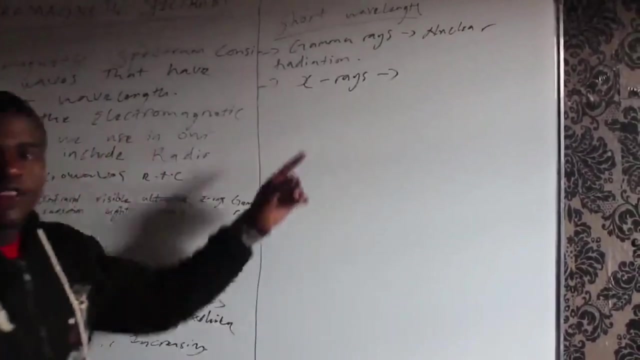 electromagnetic waves that have a short wavelength. so electromagnetic waves that have a short wavelength. we have the gamma rays. we have the gamma rays and the source of the gamma rays is a nuclear radiation. so nuclear radiation. we also have the x-rays and the The source of the X-rays is explosions. 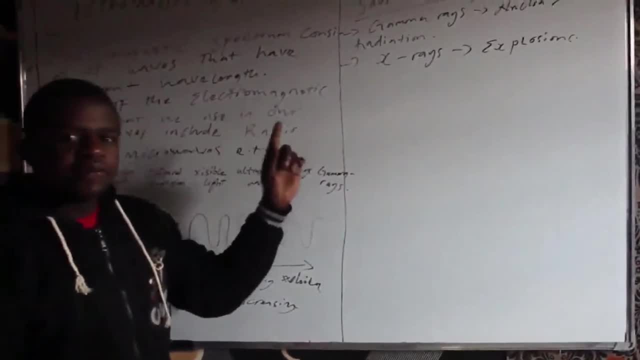 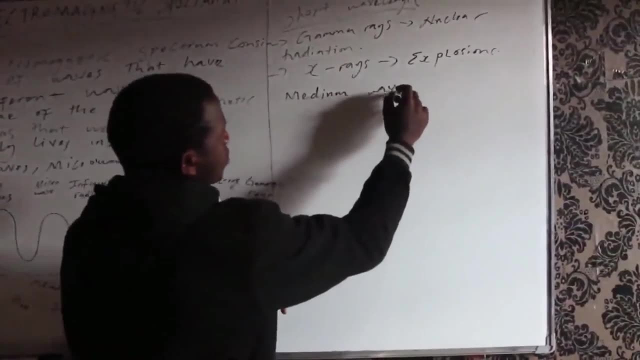 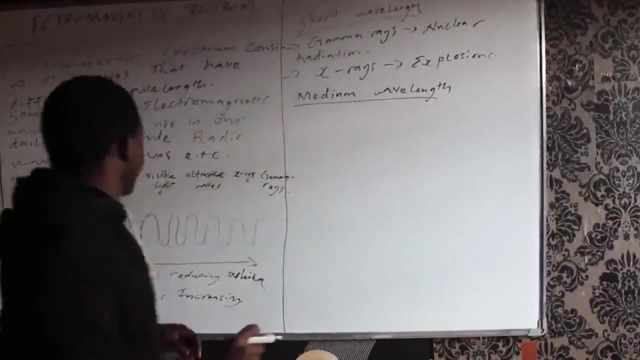 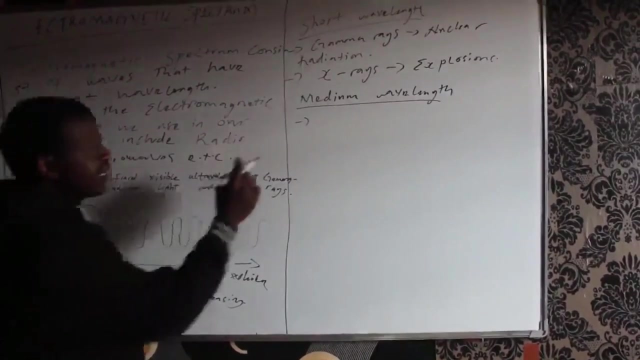 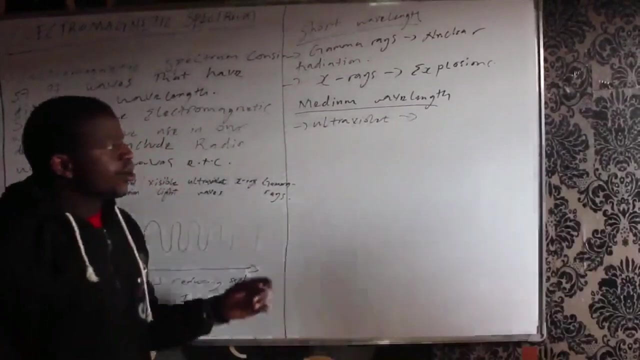 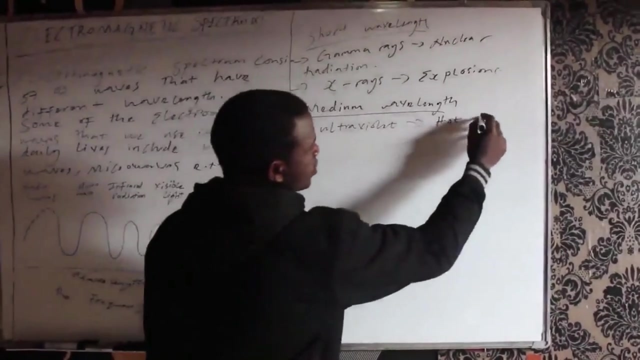 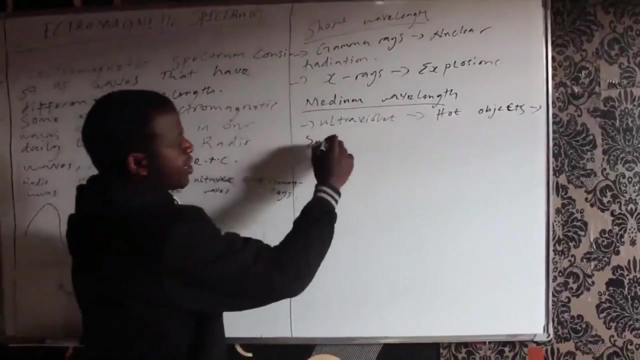 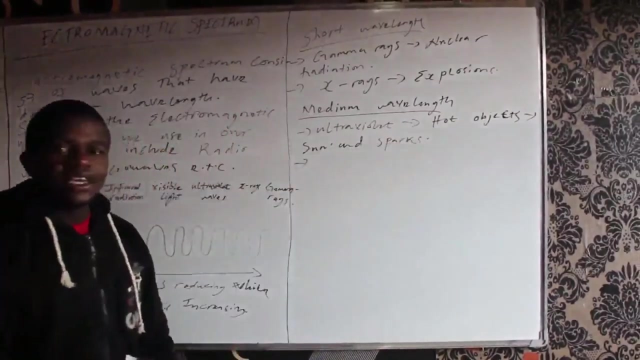 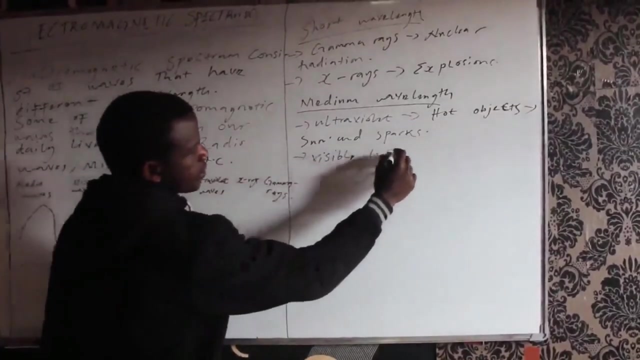 Then the wavelength are the electromagnetic waves that have a medium wavelength. We have the ultraviolet. So the source of the ultraviolet: they come from hot objects. These include the sun and the sparks. Then we also have the visible light. The source of the visible light: we have hot objects. 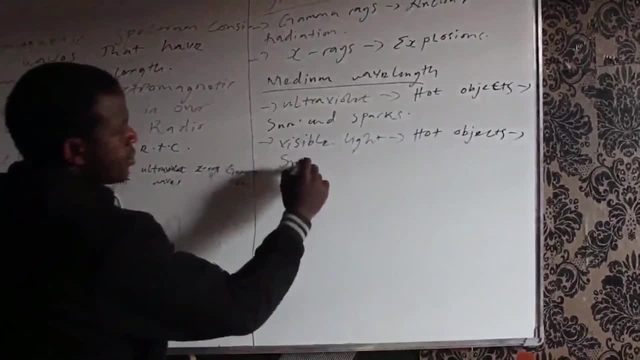 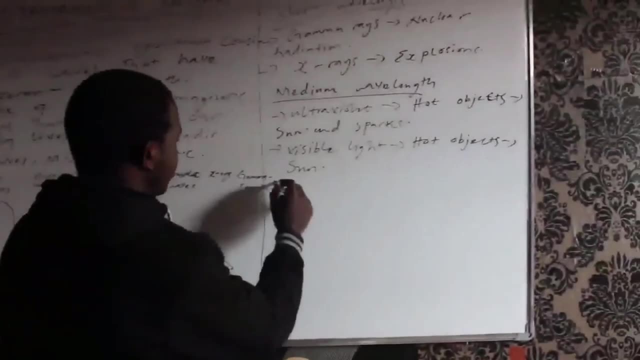 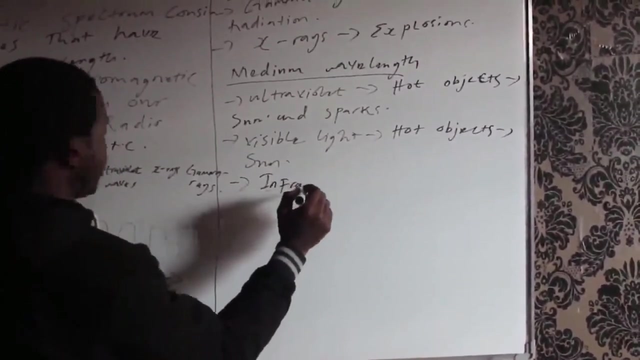 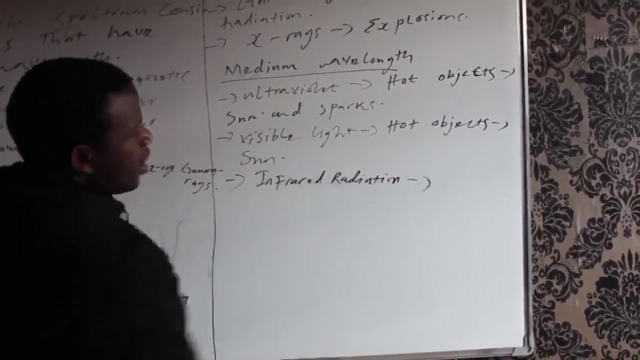 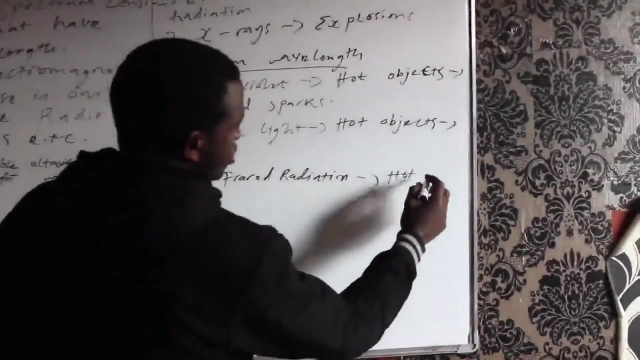 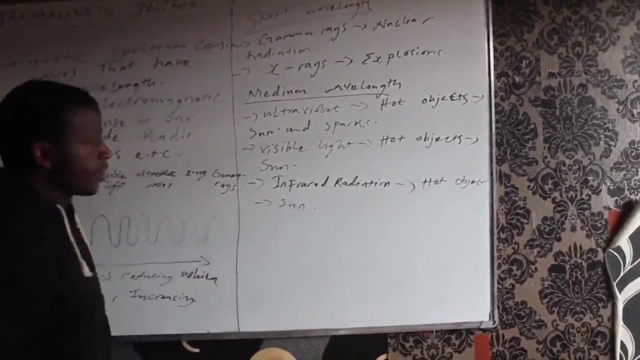 So this includes the sun, Then the other electromagnetic wave that has a medium wavelength. we have the infrared Infrared radiation And the source of the infrared radiation. we have hot objects, So hot objects, one of them is the sun. Then we come to the microwaves. 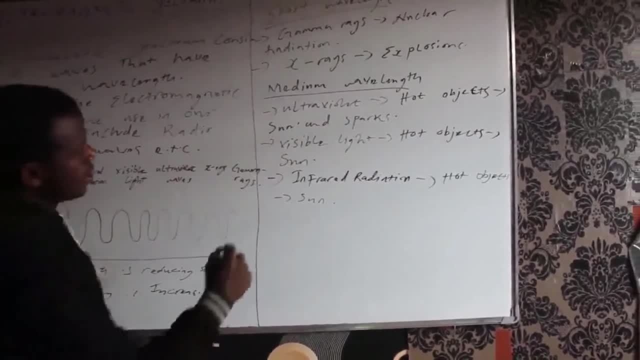 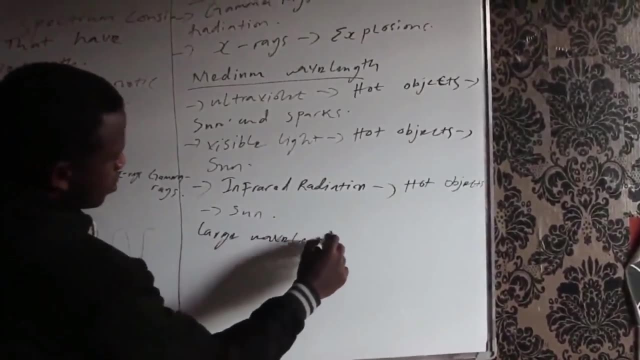 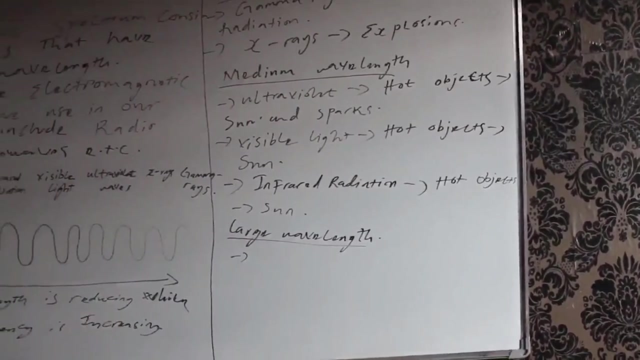 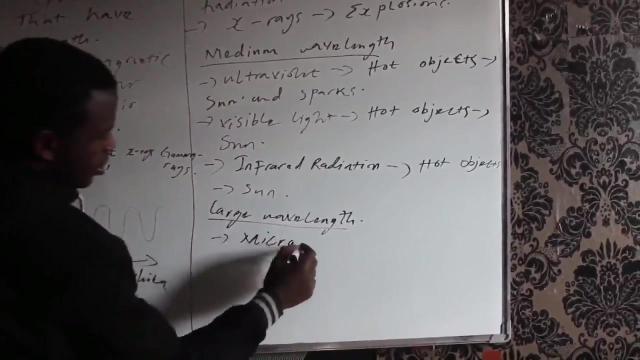 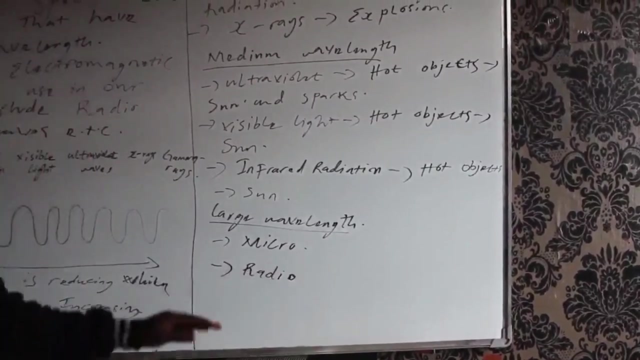 In the radio waves that have a large wavelength, So those that have a large wavelength, we have the microwaves in the radio waves. So the microwaves in the radio waves, So the microwaves, they come from short transmitters. 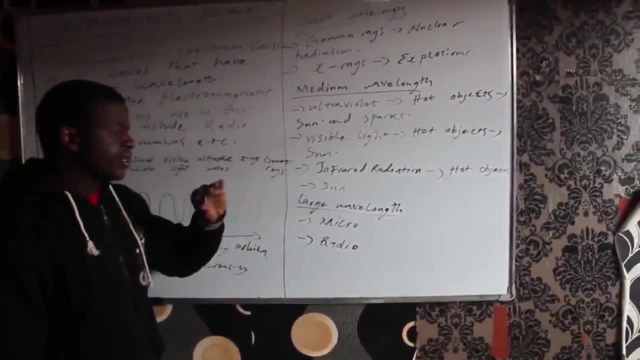 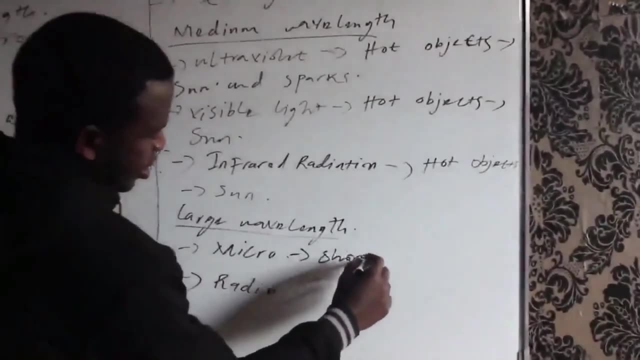 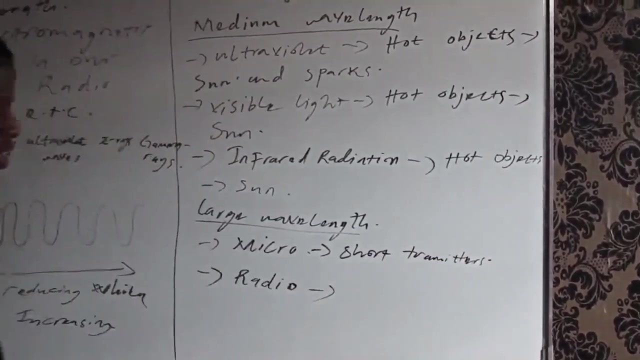 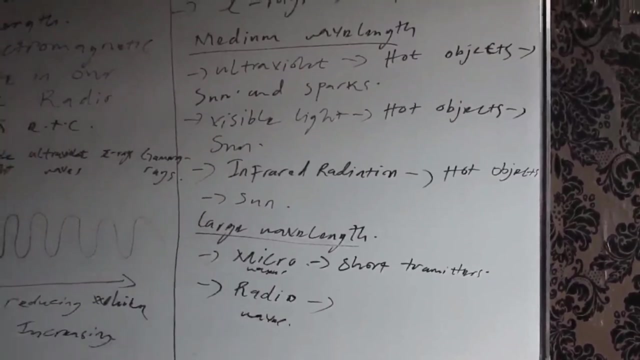 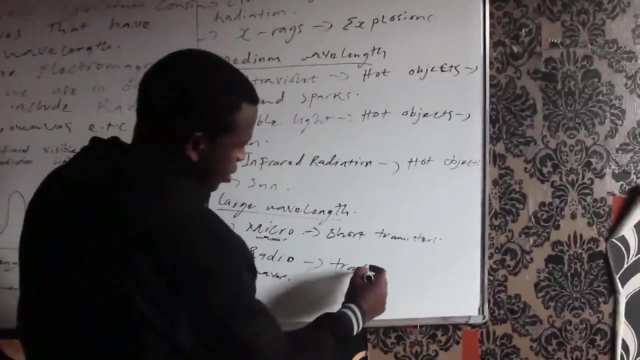 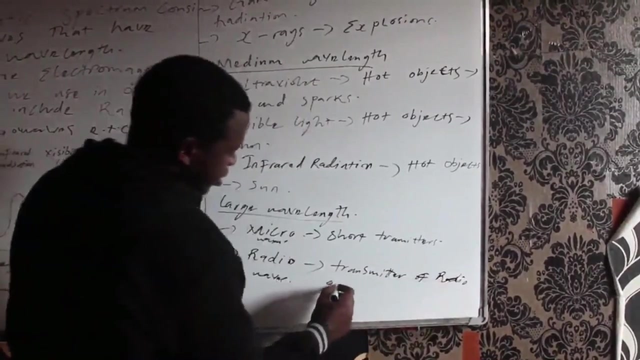 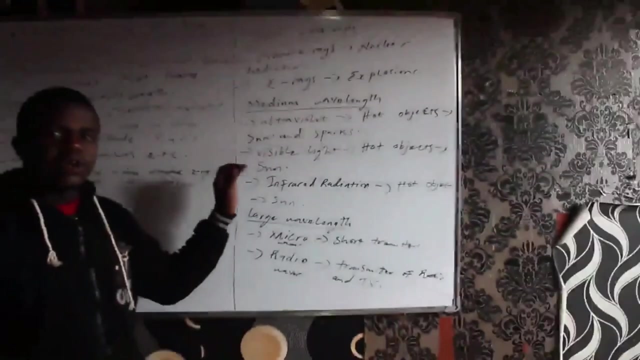 So these transmitters include those that transmit signals for the cell phones. So these, they come from short transmitters. Then the source of radio waves: They come from the transmitters of radio and TV. So transmitters of radio and TV. So the next thing that we are going to talk about are the characteristics of the electromagnetic spectrum. 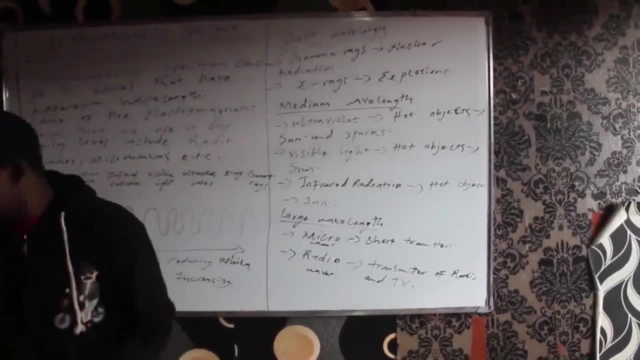